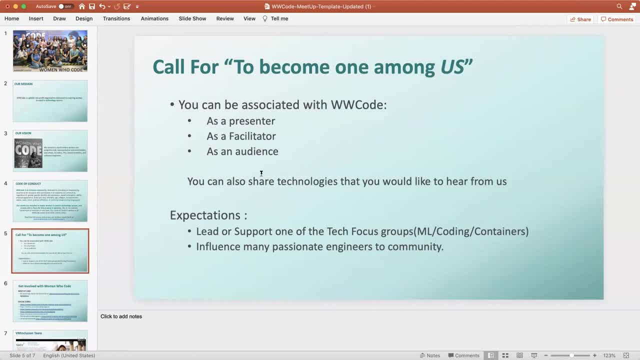 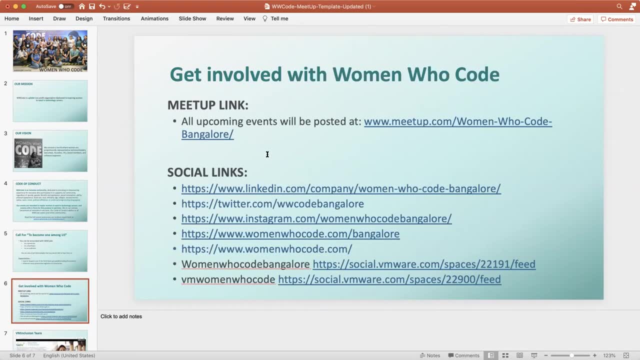 So those are the ways in which you can get associated with Women Who Code, And do check out the Meetup links and the social links that are available for people who can like follow us on Twitter, on Instagram or the global Women Who Code links also. 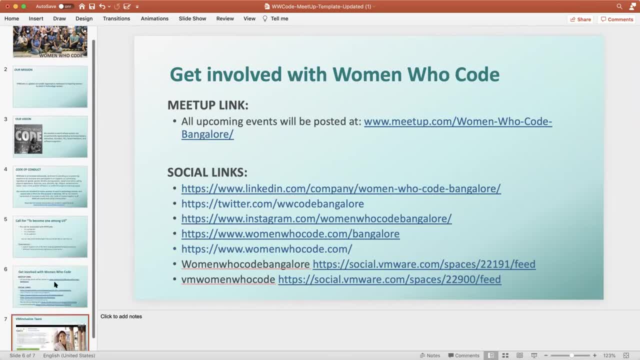 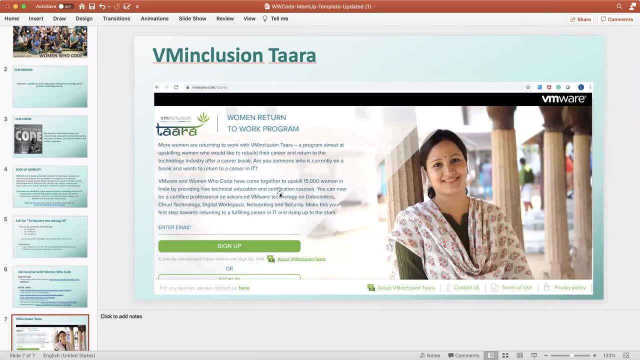 So these are some of the links And there is an interesting opportunity that is available for women who has taken a break and are aspiring to come back to work. This is a different program that offers VMware certifications on three levels of certification which can be taken at a self paced way by by women who are currently on break and can give certifications. 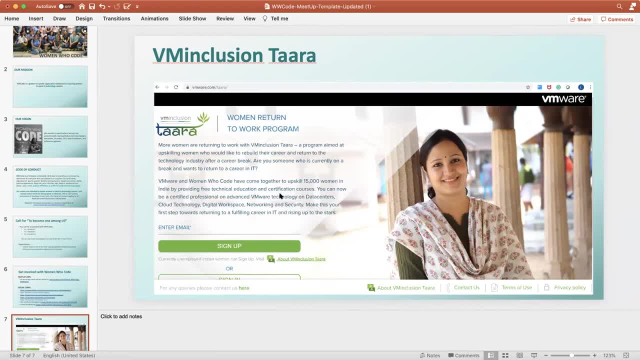 and like acquire certifications and become a like talented workforce that can like boost their resume and come back to the work for like come back to workforce. so do refer to any of our colleagues or anybody who is interested and currently on break to visit this tara website. 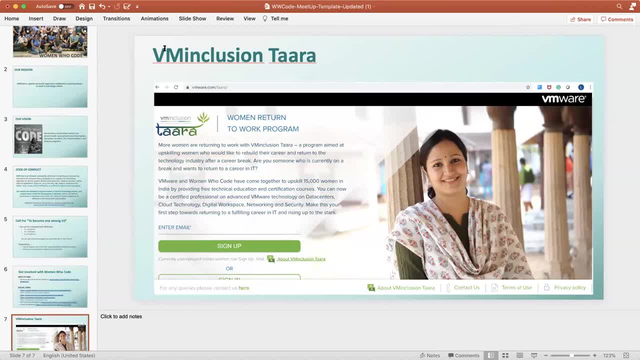 and without further delay, i would ranjini. there is a question in the chat window which is asking if one is interested to become facilitator. okay, what to do? yeah, you can write to like. you can visit the women who code global website and you can feel free to write to the. 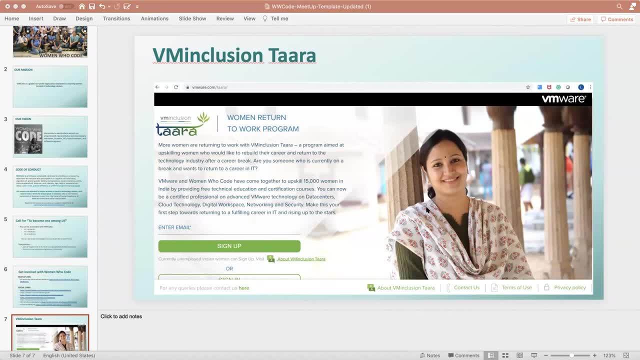 email id so one of us will respond to you with the session details that you are willing like wishing to conduct, or like the topic that you are willing to present. okay, those details will be, uh, like, we would be responding back to you. please feel free to write to that email address in the global women who code uh website. 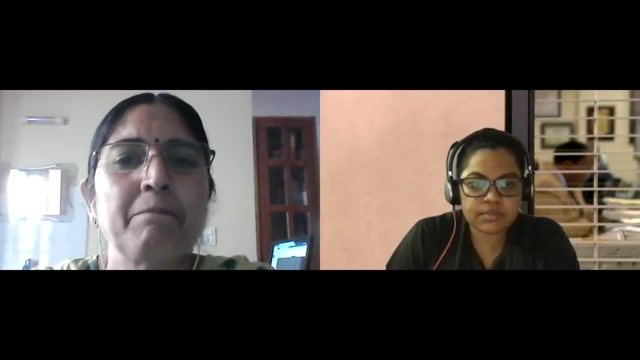 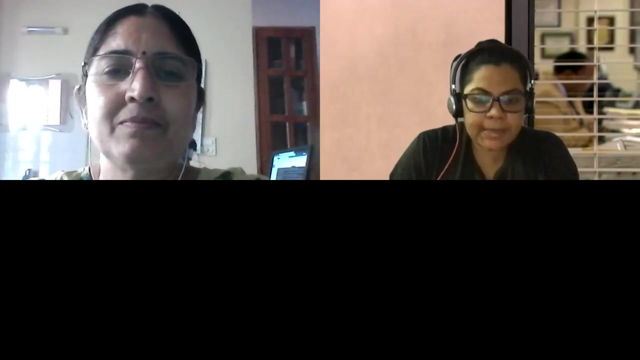 and uh, yeah, sorry, i missed introducing mini, so the session for today is, uh, introduction to fractals and uh, it is. it is uh something different from whatever we have. we have had, like, uh, the technical topics around latest technologies and some things related to kubernetes or the artificial intelligence, machine learning or cloud related. 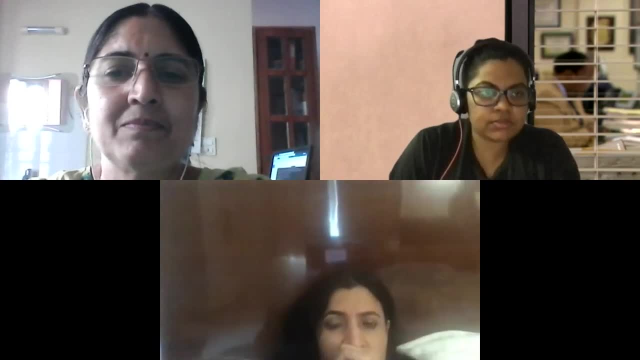 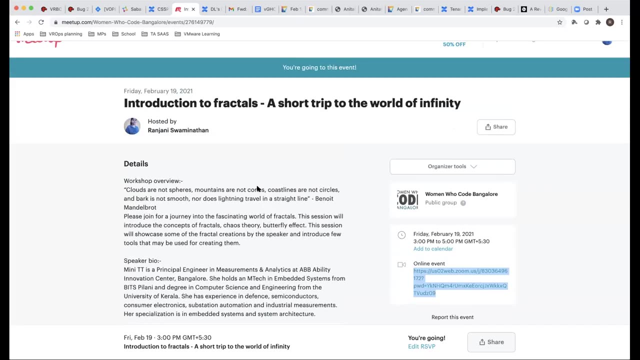 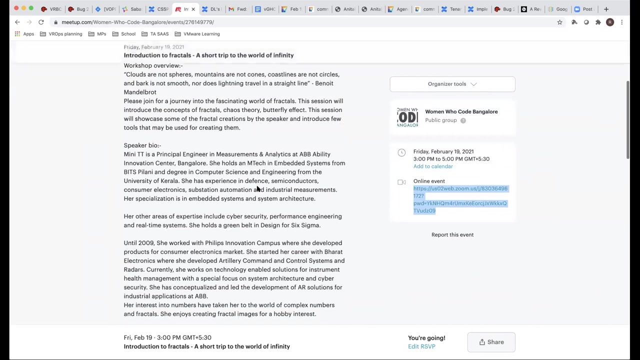 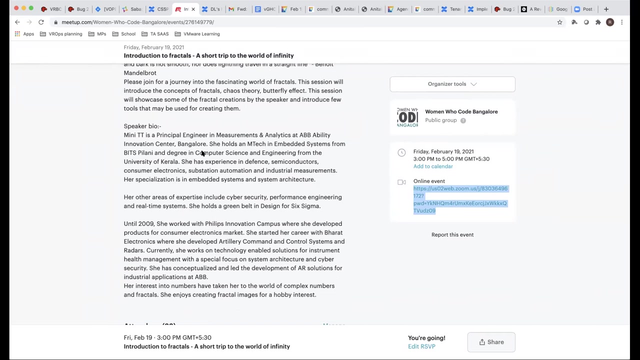 technologies, so this is something different. so i am also interested to know, like, what i can learn from this session. so this is an introduction to fractals and the speaker is uh, who is a principal engineer in uh measurements and analytics that abb ability innovation center, bangalore. she holds an mtech in embedded systems from bits palani and degree in computer science. 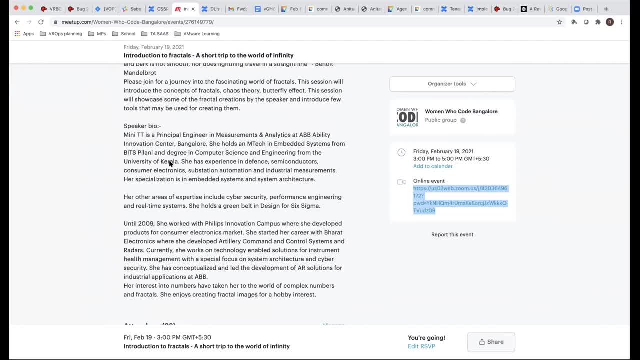 and engineering from university of kerala. she has experience in defense semiconductors, consumer electronics, substation automation and industrial measurements. so we got her like acquainted with her and she is a professor at the university of kerala and she is a professor um and she has a degree in electrical engineering and we got her hand in mind the next session. 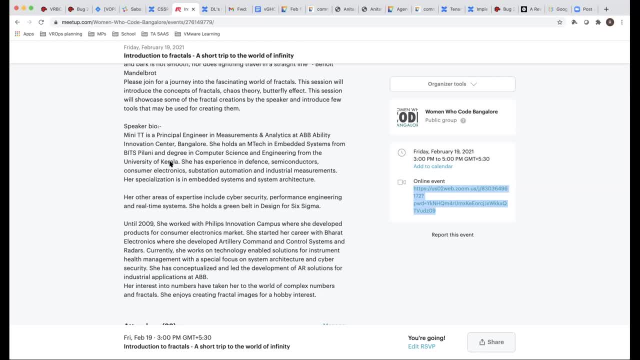 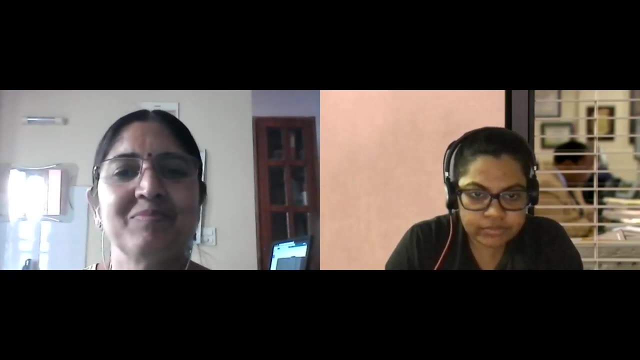 are um head and shoulders disadvantage of voodoo. this is something that we can learn about um in the current style. so i think you be, if we take the opportunity to. we are very pleased to have your壓 in SOFTLINK in our hand in mind that entire coming. but i will be upon you, sir. 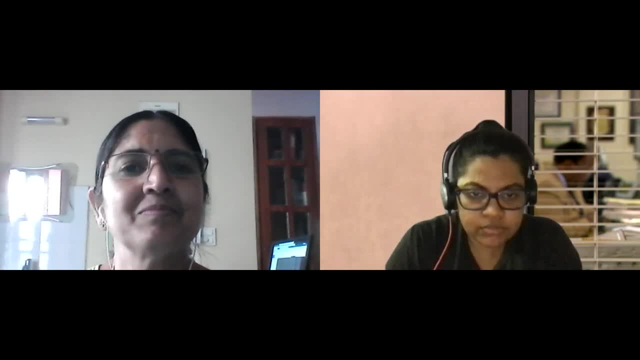 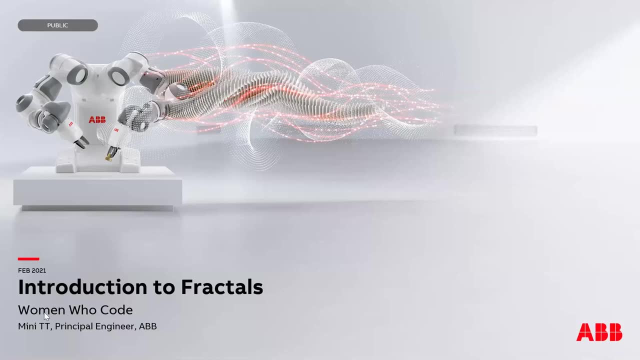 okay, now is my screen visible already. yes, I'll switch on my video for a moment. I think probably I'll switch it off after a while. okay, so that's me, because have some familiarity. after that I'll switch off and then we'll continue and focus on the contents, and I'm very happy to see that. 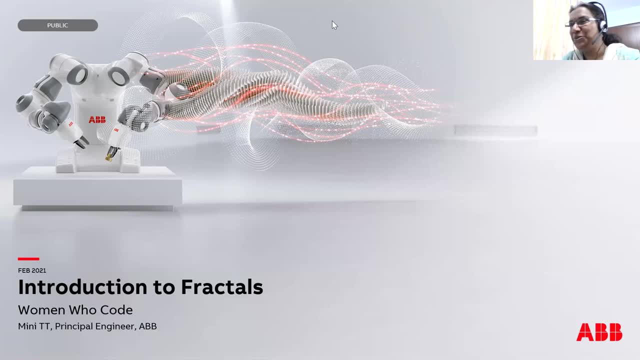 there are some familiar faces. who is inside, especially Shubha and Nisha and all that. very happy to be talking to you people in some kind of a presentation time after long, long, long talk time, and you can type in anything that you want in the chat window. I'm seeing the chat window also. 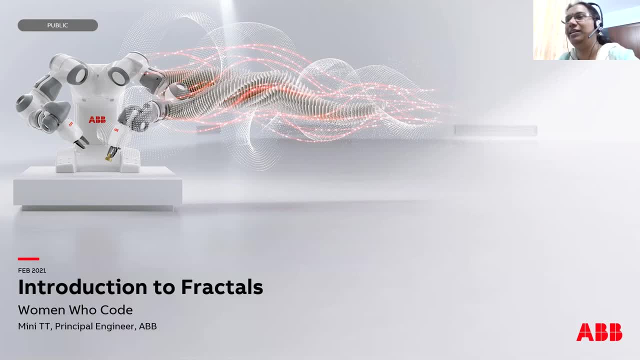 may not be continuously, but at least off and on I will have a look and if I go too fast, please stop me, and you are also free to stop anytime and ask any questions. the contents are interesting. it's something slightly different, so the topic is about fractals, introduction to fractals and thanks for women who code for. 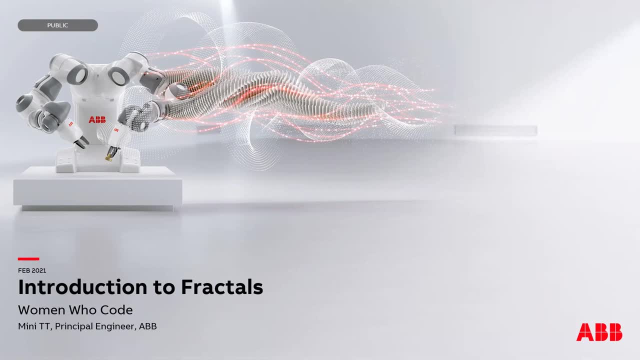 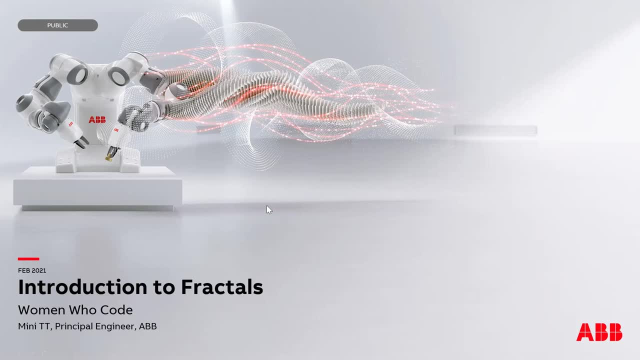 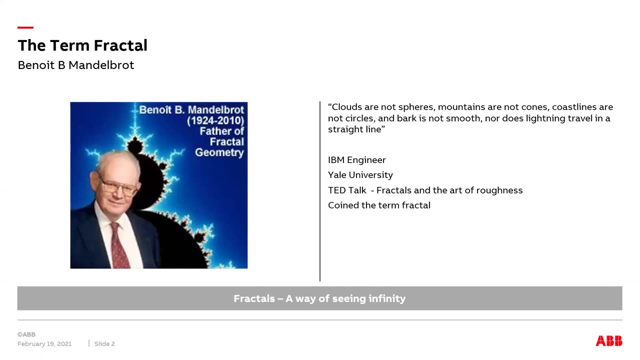 the topic. so let us start, okay. so let us understand the term fractal. this is about giving respect to the person who coined this term, called fractals engineer. I'm stopping to see that sat window. if there are questions, you please. you know, to see that chat window if there are questions, you please. 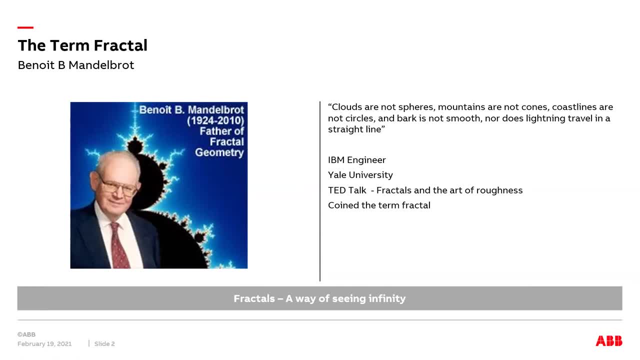 yeah, thank you, yeah, yeah. so let us see who came up with all this and the person who introduced this concept of fractals, so that we use this window also. maybe i should minimize it, okay, so that whoever gave me so much of pleasure and enjoyment? so it is good to know who that created all this. so, if you look at, 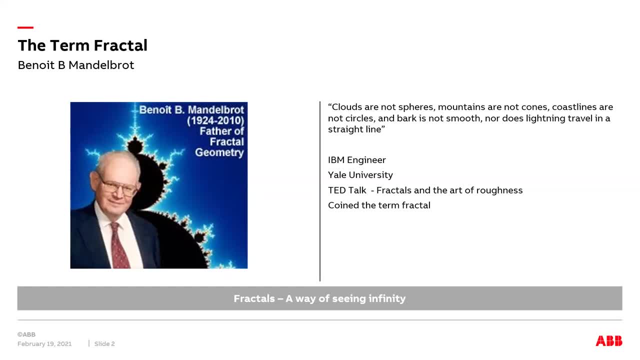 computing. long ago, long, long back ago, computers did not have so huge of a computing power. so if you are looking at old microcontrollers, they only could do only very less amount of computing. so this complexity and these patterns that are hidden behind these numbers, they were not that. 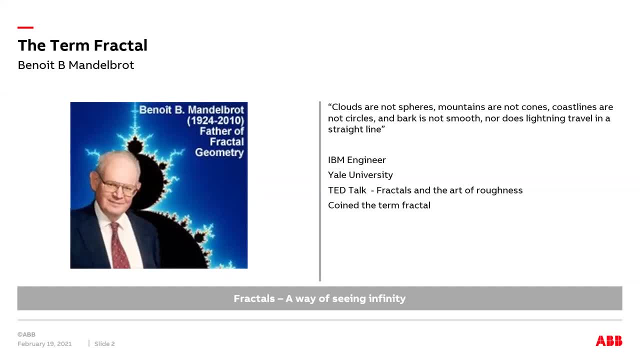 easily seen, for the reason that you could not afford to have that level of computing. okay, so just give me one minute, let me just put some time around so i'll have some control on time. okay, thank you. so this is a person who is known as manuel. 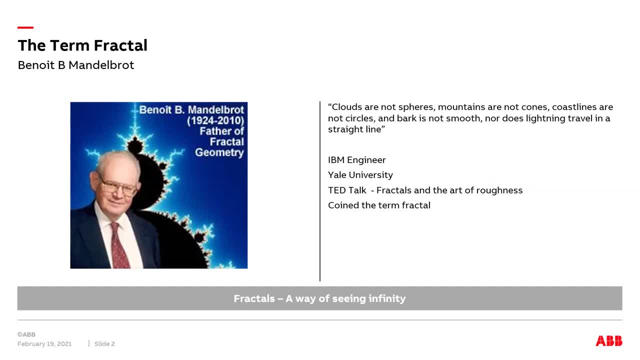 brott. so this manuel brott was an ibm engineer, so who used to work on these computers in the early days of heavy computing time and, at that time, having the computing power available at his disposal. that was the time that these fractals came into being, or the discovery of this computing. 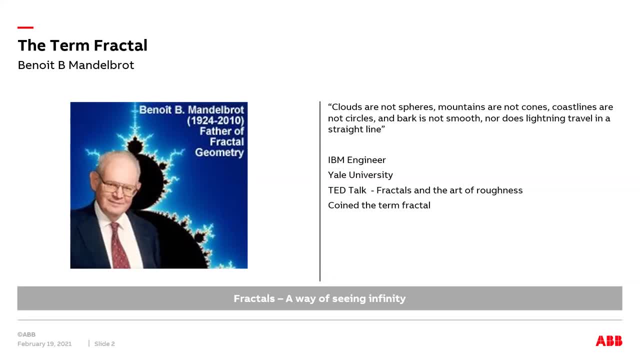 and the equations of nature came into visibility, though it was always like that. so that was what we are seeing, this a very fantastic discovery. so if you hold that, you're able to yourself paper, actually understand that from thiscimento Ф, nämlich beautiful: этотstä thứ السماء. 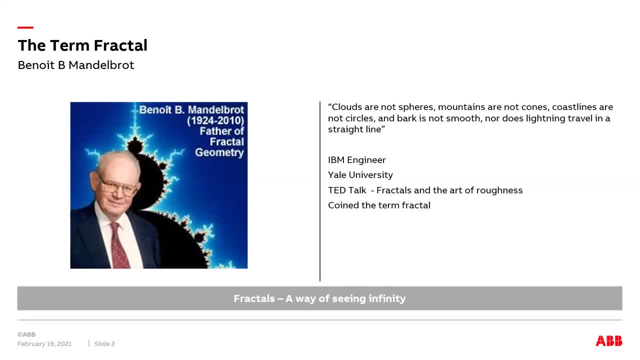 sochu Shaun. very fantastic world to understand because this is a universe in itself. and this mandelbrot is the person who coined the term called fractal and he is also known as the father of fractal geometry. so if you look at nature, like when you see a lot of walk around, and if you see around nature, you 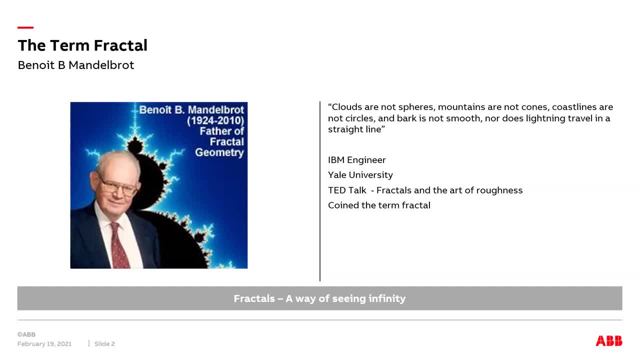 will see a lot of fractals. the moment you are recognizing the patterns, you will see a lot of them. so if you are more interested in knowing about the person, yale university. yale university has a dedicated page where all his works are put on display, so all his writings. 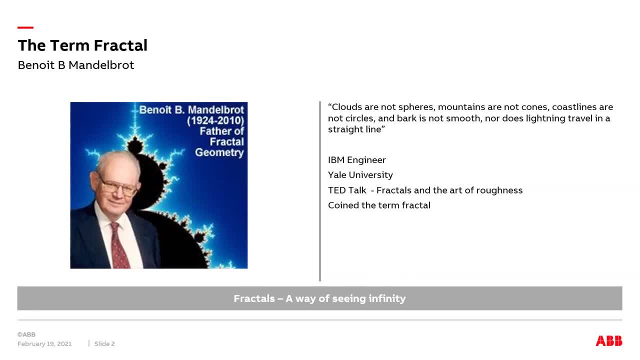 papers, publication, everything is there in yale university page and there is a ted talk. the video is available. it is called the fractals and the art of roughness, and if you are thinking that, when did this all happen? it's not too long back. see like he passed away only in this year, 2010. 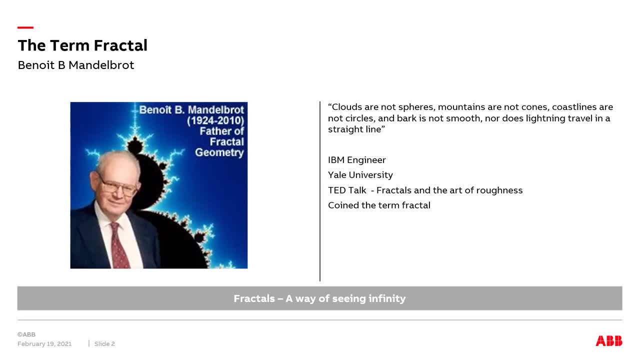 that is very recent. it is only 2020 that we are talking. so this is the person who came up with all this concept of fractals and who came going to the term called fractals, and that is what we are enjoying today, and this is about infinity. like we will come to that later, it is all about infinity. 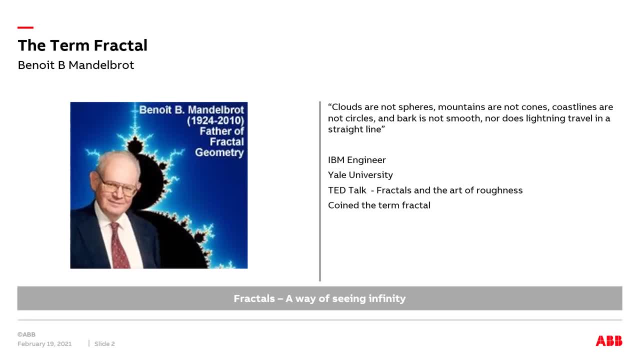 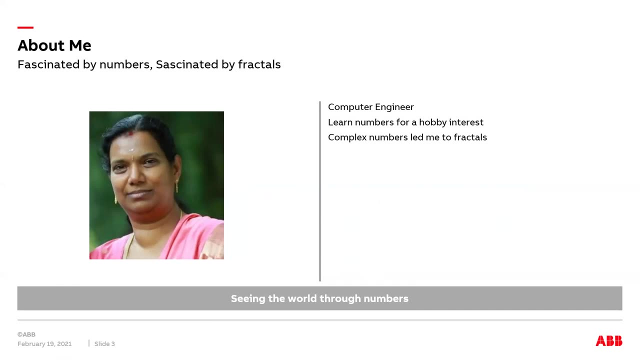 and what we see in nature and what we see in the universe around. that is all to do with infinity. i would suggest that you have a look at that ted talk, because that is very interesting. ted talk and then about me, as an engineer introduced me. i have done my computer science, engineering and 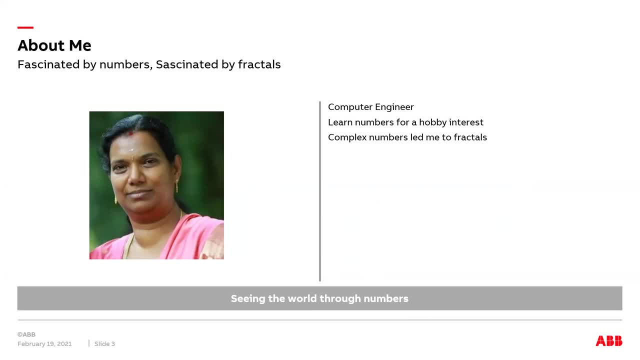 primarily i am a programmer, computer engineer- that's what i am, and i learned numbers for a hobby interest. that fascination for numbers was always there. like, if you see the audience here, like some of them they know me from my college days itself. there was some hidden number interest. 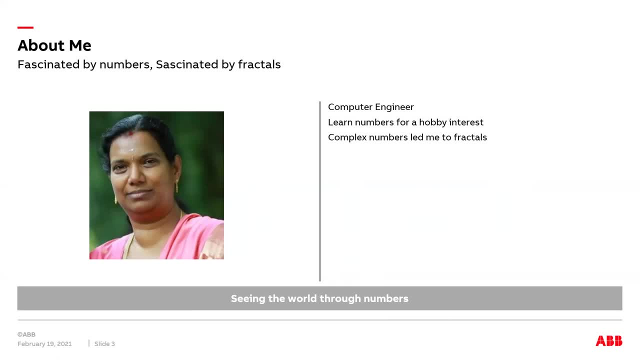 which used to be there. that is what popped up and then got me into this, uh, fractals. so i'm learning this more like a hobby, interest and the fascination for complex numbers. that's what got me into this fractals and once i am into it, like i off and on as i keep getting. 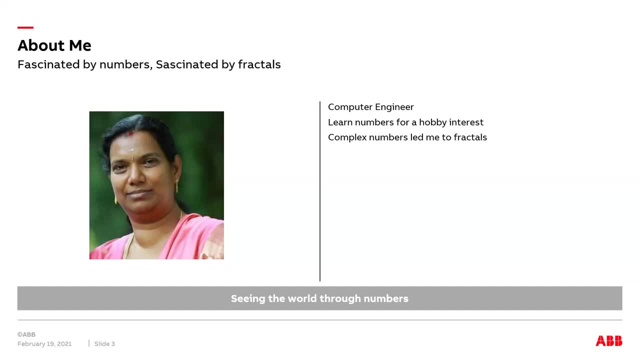 time. i keep doing it. so this is a way of seeing the world through these numbers. so now my challenge is that, as you, as i, find so many things around. instead of just finding the beauty of things, you are seeing the numbers, so i do not know whether the number is more than the number of the. 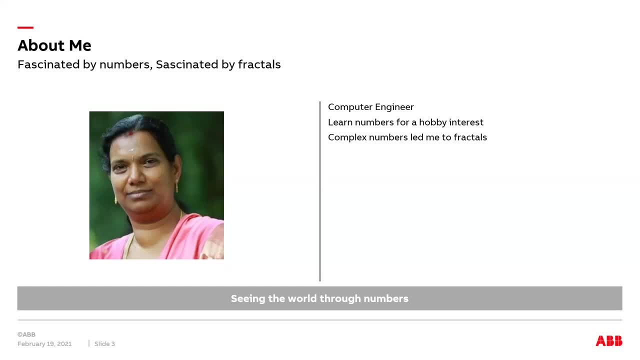 boxes, or the number of the boxes is more beautiful or the picture is more beautiful. that is what the challenge that i'm facing right now, by seeing this kind of understanding in mind. so you see a tree there, then you do not know whether you have to see a tree and green and 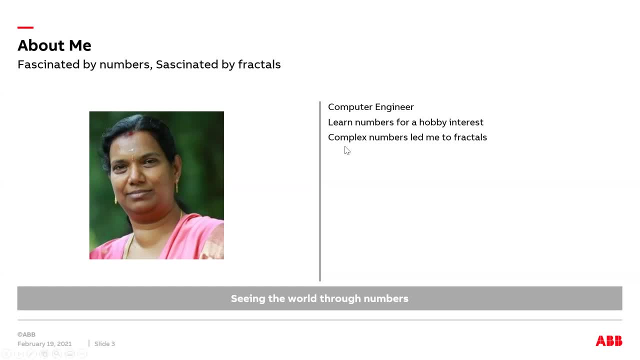 picture, or whether you are supposed to see numbers and equations. so that mix is something. sometimes it creates one confusion, but still that's also something which i am enjoying also. and let's see what are fractals? so fractals? this is to do with the fact that this is all the fractal. 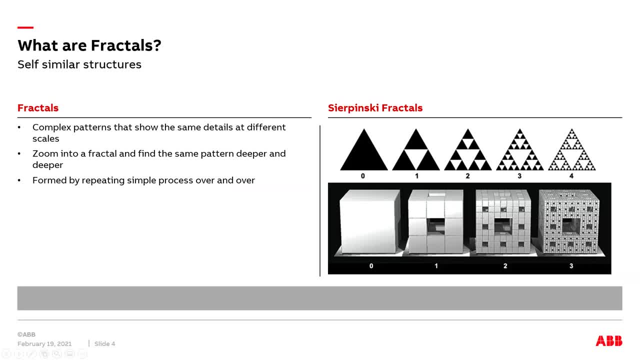 the self-similar structures. so self-similar means at different scales, they all look the same. so you get into the different level of scale, the more and more you get into details, you will again see the same thing happening again. so that is what the all about: self-similarity, the complex patterns. 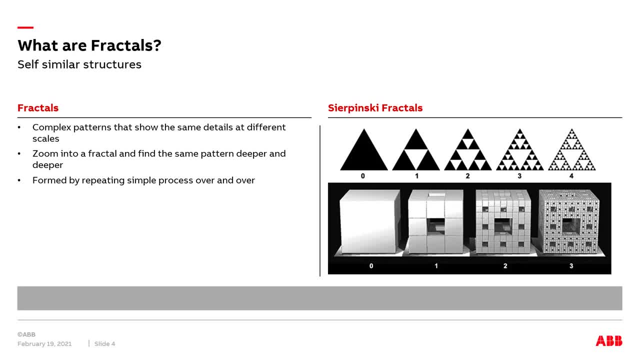 the complex patterns. so they are very complex, but then it's not like like. it's not like a long partial differential equation with so many things inside. that's not the way we are talking. it has its complexity at the same time they are very similar and very same. and then that same pattern. 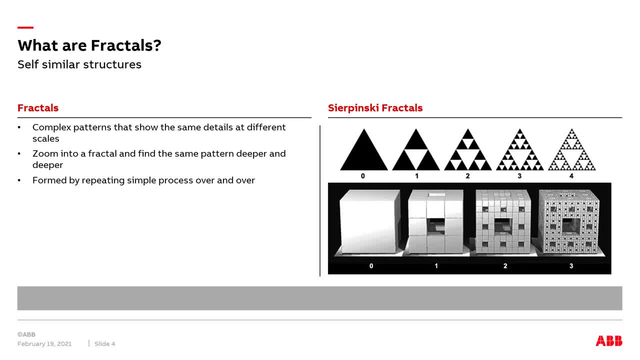 repeating. and if you zoom into a fractal and then you it, it's like you are walking into the infinity. as you get into the deeper and deeper into it, you will keep seeing the same pattern, again and again and again. that's what you will see in a fractal pattern and it is repeating, a simple process over 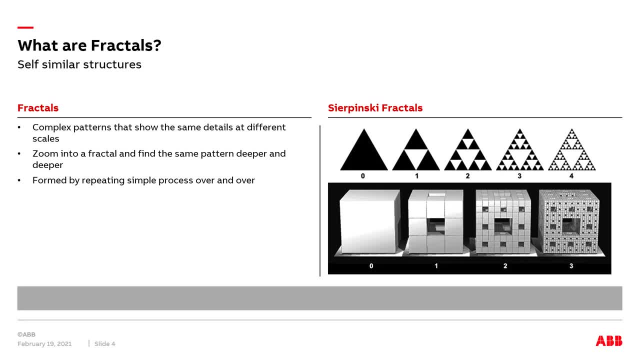 and over. it's not like the is a very difficult. it's not about difficulty, but it's complexity. you and there is a difference between complicated and complexity. so what we are talking is complexity. complexity is a behavior pattern that you will see about the systems in the nature. so you can see right now on the right. 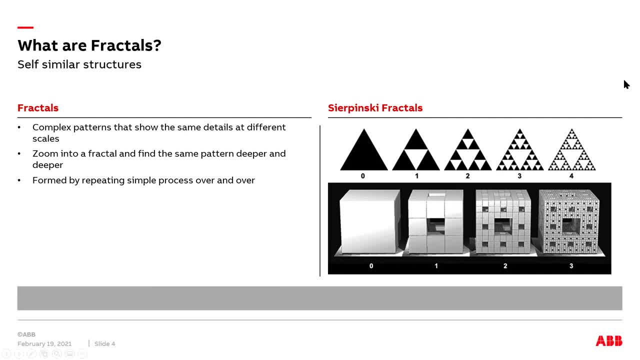 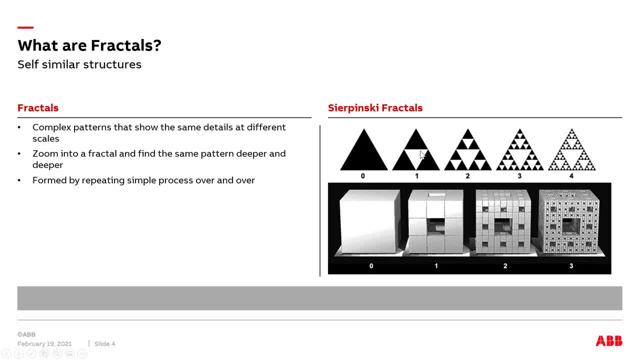 will keep getting the same patterns. you divided into the three, into multiple parts, and you again repeated the same pattern on the same, on one triangle and every other triangle, and you keep going inside. so your dimensions of the triangle may come down and down and down and down, but it 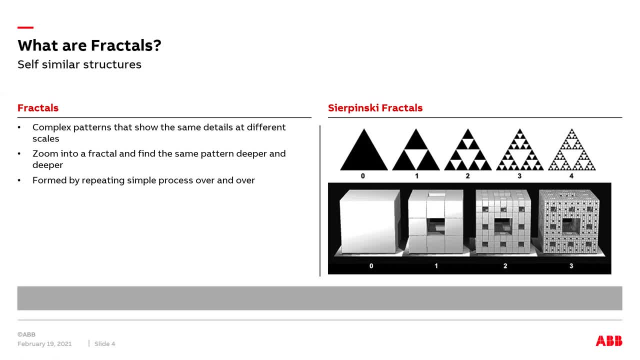 never reaches zero. so it doesn't disappear. it will keep going on and on. as you walk inside more and more, you will keep seeing the same thing again and again. that's what i'm trying to show here by these geometric patterns. so this geometry, these are not the same patterns. they are not the same patterns. 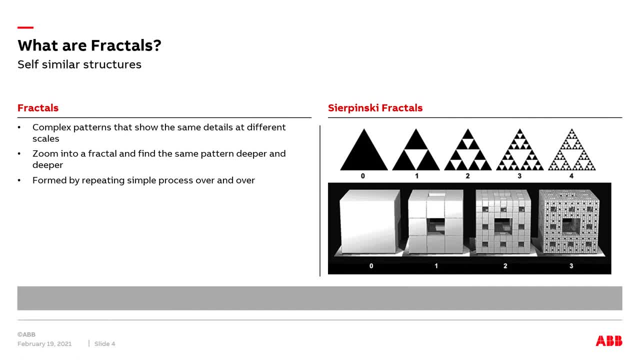 these are known as geometric fractals because we are creating out of this 2d geometry or 3d geometry. so down you can see one which is a 3d geometry based one. see, that is a cubic fractal. you take the cubic and then you're creating the same pattern again and again. then you will get here. 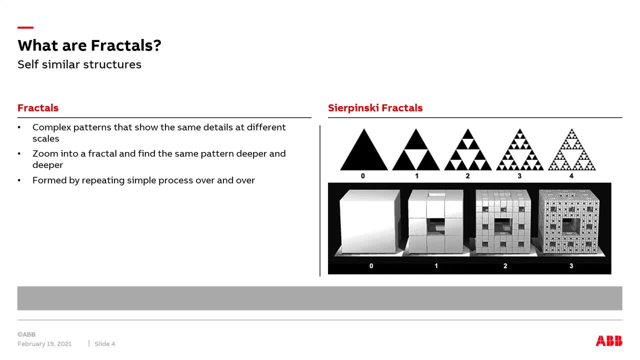 so there are so many in my system, i'll show you at the end of the session, if there is time, whatever i have done over the this period of time. there are so many. i'll show you some of them. so those are the patterns that you will see. then, to continue, let us look at some of the fractals. 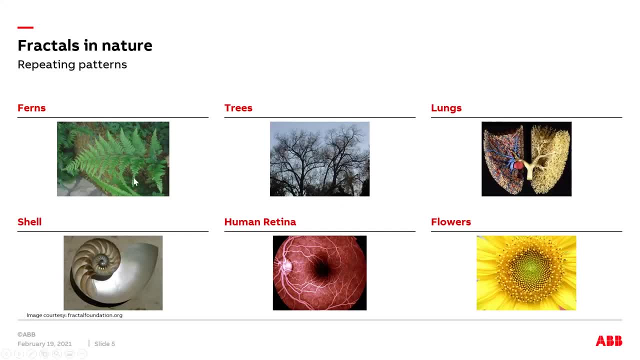 that we see in nature. so these are the patterns which i just copied from internet to these pictures. so they are repeating patterns. if you look at the first one, the ferns, what you see is that stem of the fern is there and then the side petals you are seeing. but if you look at that one, 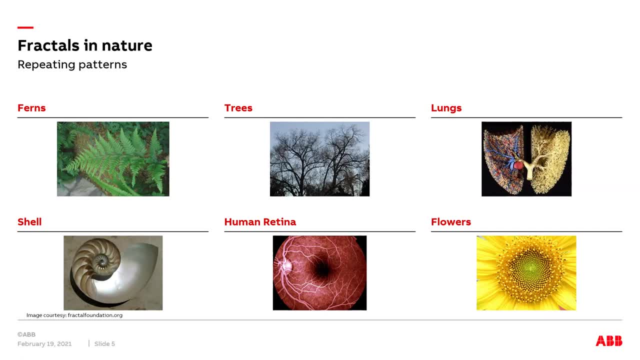 petal again, it has the same pattern once again inside. so if you are given the entire fern or if given only that one part of that phone, just by looking at it you do not know whether it is a whole, whether or whether it is only a part. you are somewhere, but you do not know whether you are in. 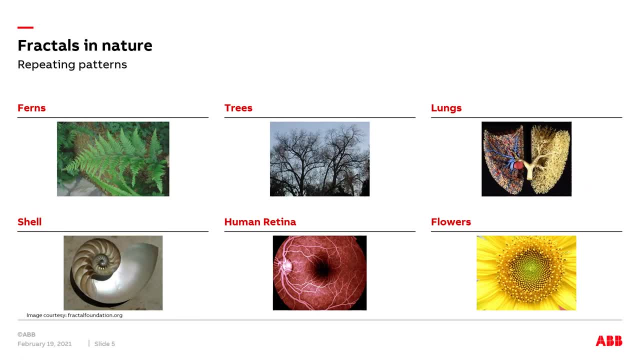 the beginning, or whether you are inside, or whether you are in the infinitely inside that you cannot make out. that's what the beauty of fractals. all together, these are all other some of the other patterns that you will see in nature, like trees, tree structures are very easy to see, the branching 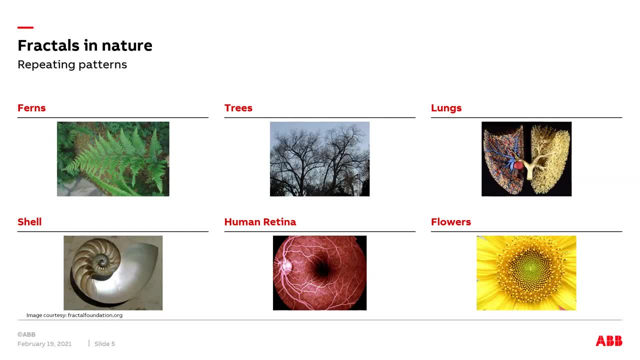 out, it will keep branching out and then you keep going. you see, like if structurally we are talking structurally, given a tree branch or given the entire tree, you do not know, like whether it is the entire tree or whether it is a branch. i'm not talking about the roots here, but the structure of 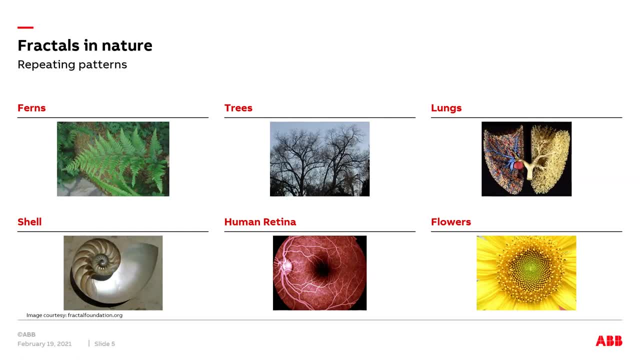 the tree in itself. it's the same with these veins, lungs, and the shell, seashell patterns, the human retina, blood vessels, even flowers. these are all nature, nature fractals that you see in the nature structures. so let us see something which pictures which i have created myself. these are the ones. 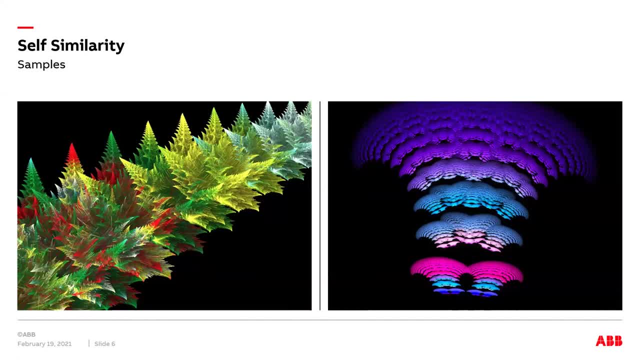 which i have created, especially the. these are very explicitly showing this self-similarity. that is why i put these two for an example. and then here, what you see is the right side. if you see you have those two patterns, three patterns or four patterns, it's, it's repeating five, seven, like that. but if you 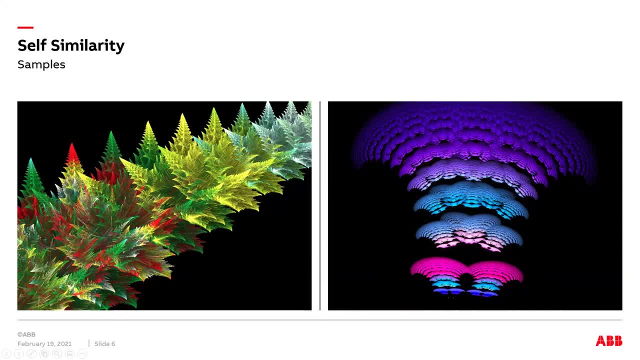 look at the one, one piece of it. the one piece of it also is the same in the similar on the left side. it is very similar to that ferns, that you were seeing the grass, the plant, so this also is very similar. but then i made it a little bit into a feel of cubic structure. 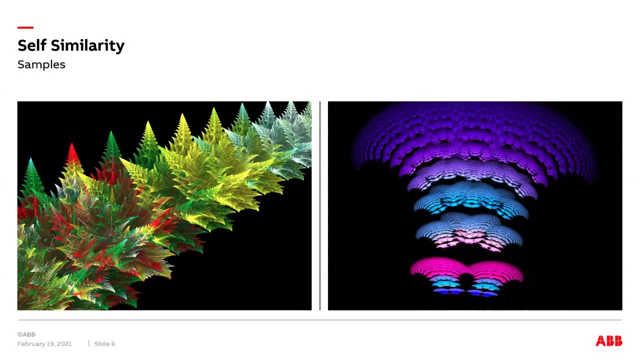 the entire stem given or the one piece given. you do not know it is. it's the same thing that is repeating, so it is infinitely repeating patterns. that is the self-similarity that we are talking about. i hope the audience is with me. is there any questions? 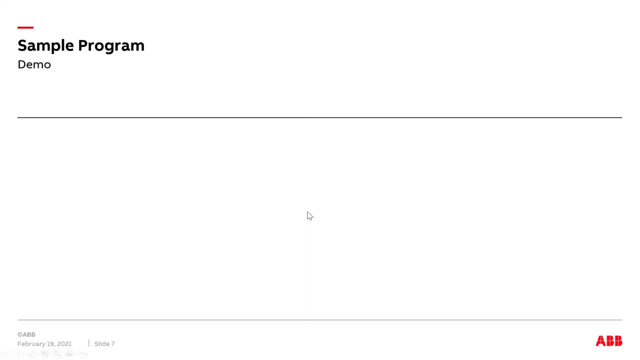 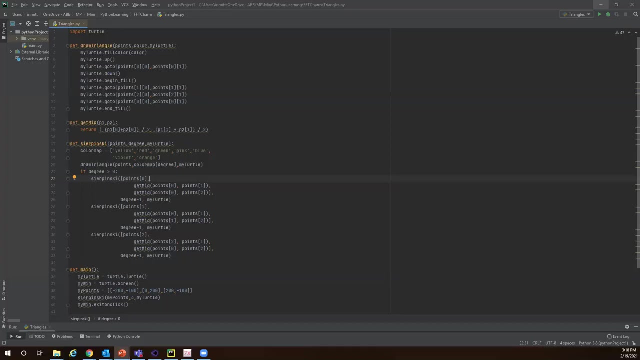 then let us continue. so i think i will: hello, yes, please continue. okay, so let us see one program. see you occasionally see, i don't write all the program. occasionally i write some programs but then sometimes i use ready to use program. so this is one python program. 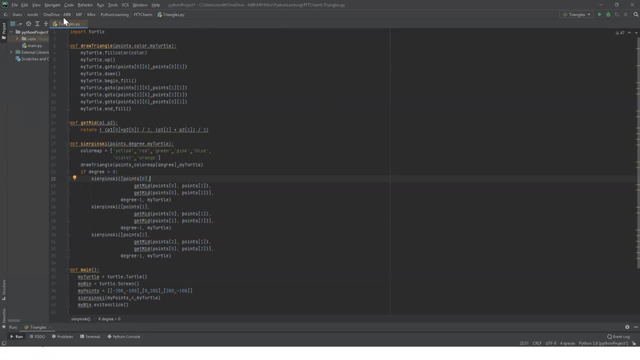 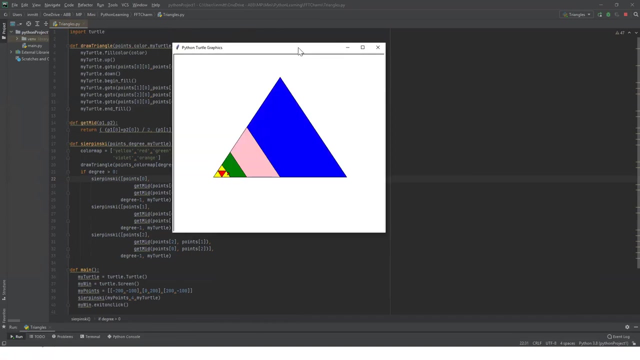 which is there for showing creating that triangle patterns which i was talking. so this is done with this: turtle graphics and basic 2d geometry. okay, you are just dividing that and then showing it, so we'll run this program. oh my god, i have to show this side. see, you are dividing. 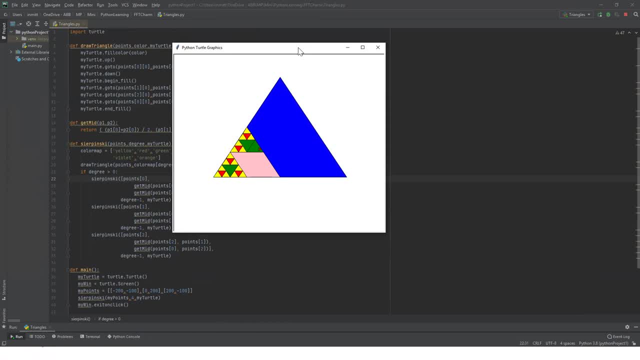 and going the. this is a program which, uh, where you were seeing that the serenpinski triangle patterns like, as you see, the beauty of it is this program: at some point it is stopping. but if you don't stop and if you have enough of place to go inside, it's just that the dimension is coming down, but then it is keeping on going. 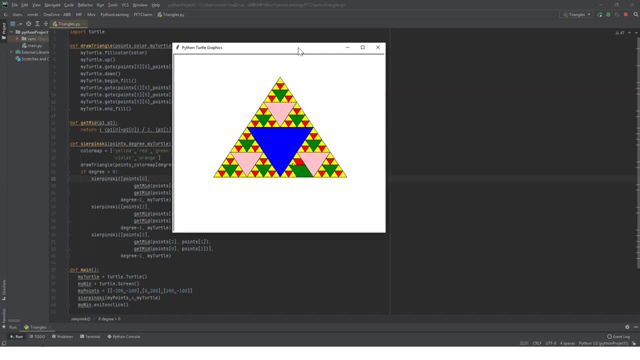 structurally it is still the same and it keeps going. so these are the things which i do for a hobby interest, like i just keep doing these kind of small pro small programs where you can see this mandelbrot set or the serenpinski triangle or even some of those lawrence equations and all. 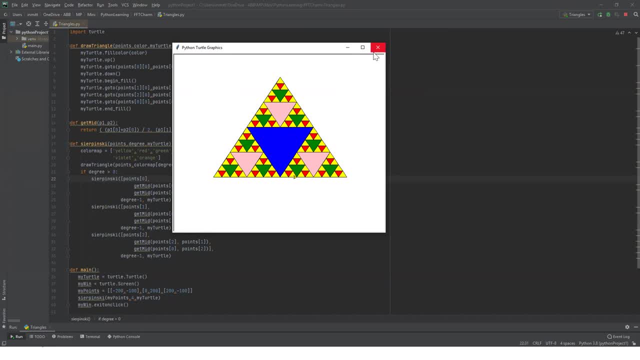 that these are one thing which, uh like, just for a demo, i'm showing you. so, if there are, since this is a women who code session, so there, like, if somebody is interested in coding, there is a lot of things that you could look at to see what is there around also. 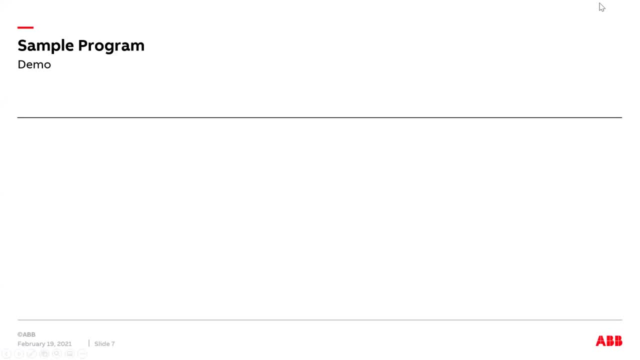 so i'll stop this one. so there is a question in the chat. yeah, yeah, yeah, they get a github with code for these factors. uh, might be there. might be, because there are a lot of some of the programs which i am using like i don't have. i don't spend money on this, so 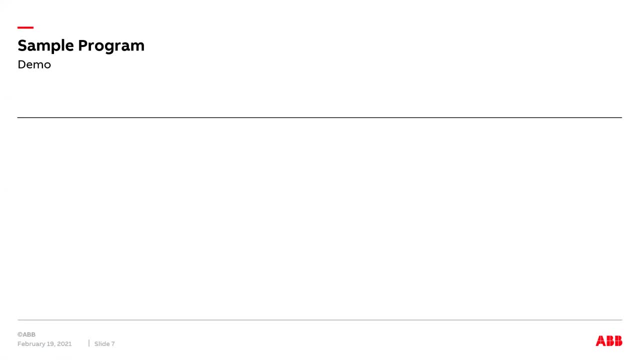 there are many programs which are ultra fractal and all that which are should be there. i'll tell the name of some tools as we go along. so all what i am using is open source program because i am not spending money on all this, but there are paid programs also. one other question is on. 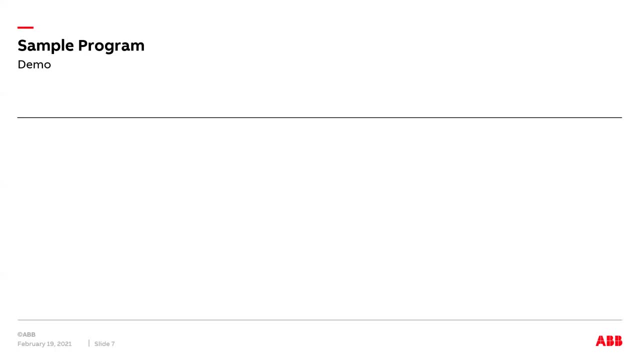 books that you would suggest to read or learn to create these books, to understand the concept of the chaos theory in itself. i have read a book, book called chaos, chaos, chaos, as a book which i have read. and i have read a book called chaos- chaos as a book, which i have read. 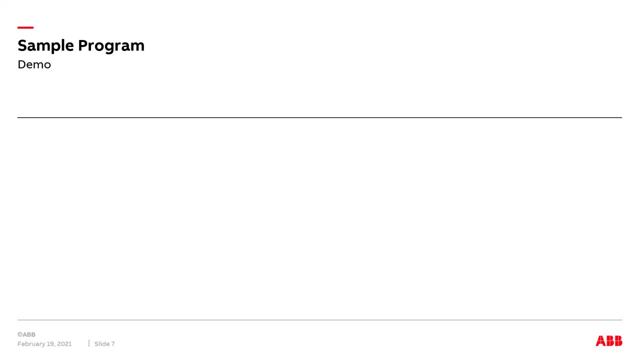 and i have read a book called chaos. chaos as a book which i have read. in fact, that is the only one book which i have read. other than that, i have studied from other public domain internet sources, like some of these data sheet and manuals of these programs themselves, or i have also referred to. 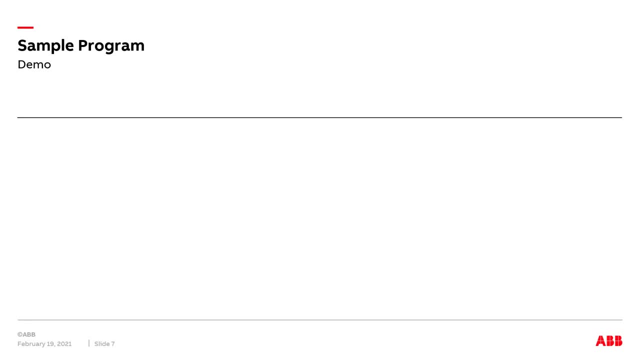 many things from these maths packages like this co-calc or mathematica or those kind of maths packages. i have learned many things from mass packages and some things i have also learned from a a graphics tools like, if you know this, gimp, inkscape and all those pro graphics tools are there right. 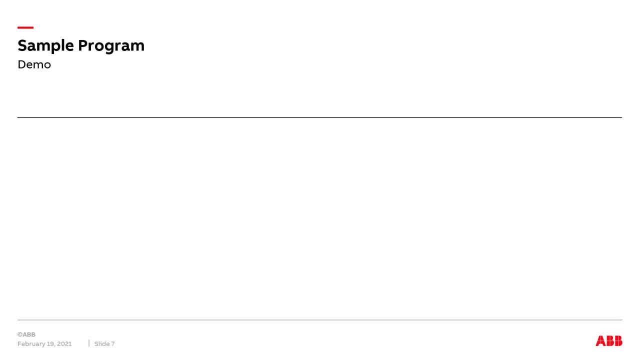 graphics, generating tools from that also. they- some of them- have these plugins for creating such things. so those are the sources which i have used and what i saw was generally these textbooks. in india. it was very costly, so that's also one reason i did not spend money on all this and do. 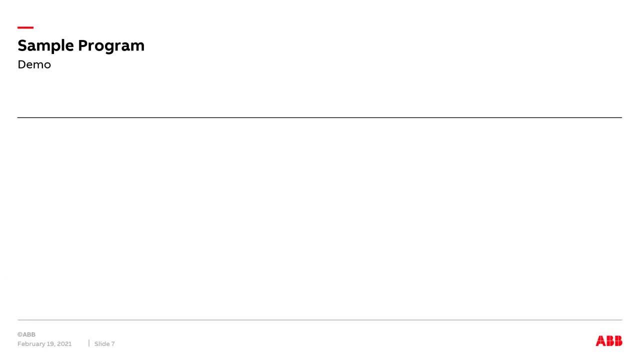 that. but the internet you will. you will see a lot of material in the internet itself. so there are forums i'll give you some links with. in fact i'm also part of one fractal geometry group in the linkedin. if somebody is interested maybe i can share that linkedin group. i'm not 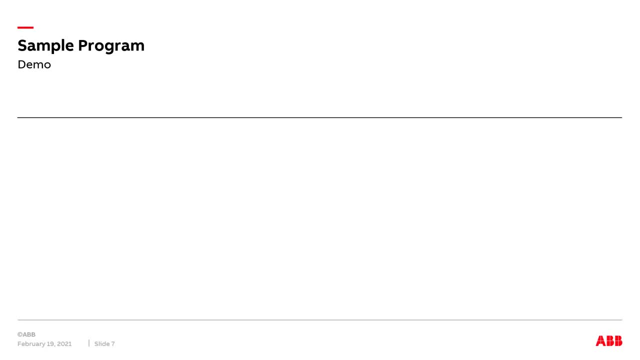 maintaining that group. but that group is there which i'm part of. maybe like i don't see too many groups, but there is a group which, if someone is interested, you can join. in sure that would help me. yeah, then let's continue. there's a group i can share it at the 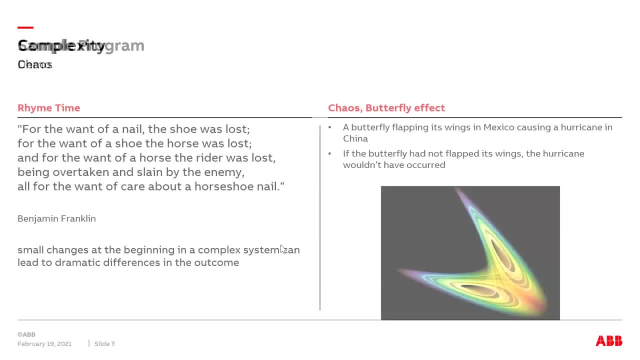 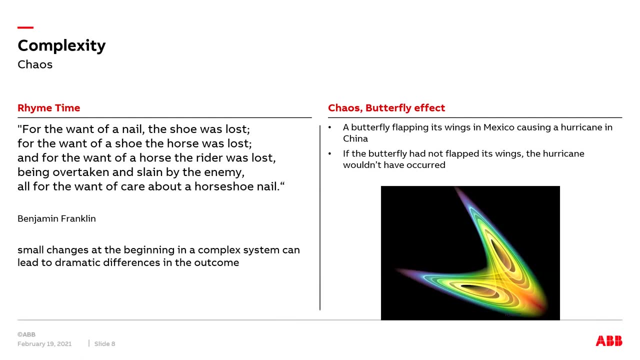 end of this session. so now let us learn. what is this concept of complexity? this is what we want to understand from all these complexities. it's a want to say it is a systems feature that the system is complex. when we say it, it means that the system is chaotic. so in the chaotic system, what happens is the very fundamental. 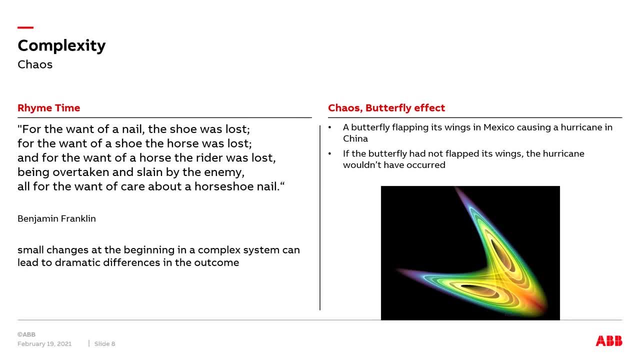 premises. a small change in the beginning of a system, a complex system, can lead to very dramatic differences in the outcome. that is what we are talking about here as complex system like. please do not equate complex as complicated. that is not what means. complex is a feature of a system. 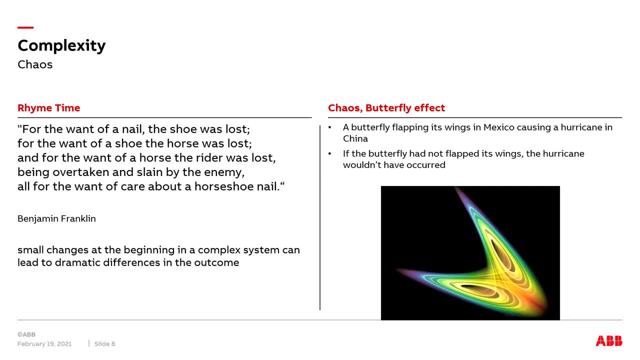 like the nature of being chaotic, and this is a nursery rhyme. so let us read this nursery rhyme then i think you will get that for this session. The rhyme says: for the want of a nail, the shoe was lost, And for the want of a shoe, the horse was lost. 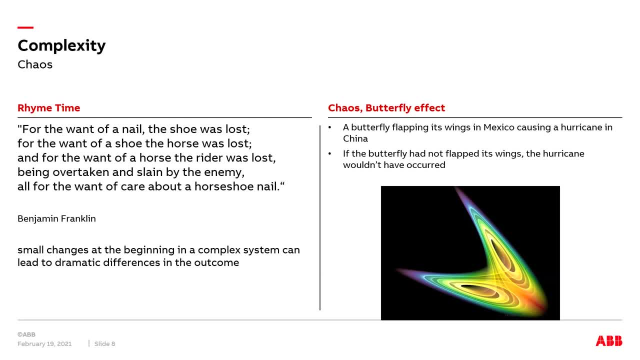 And for the want of a horse, the rider was lost, being overtaken and slain by the enemy, All for the want of care about a horse shoe nail. So what it is telling is about losing the whole war because you were missing a horse shoe nail. 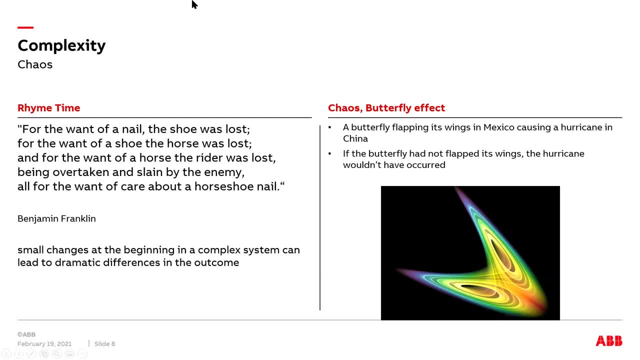 So this complexity is in that kind of a nature, like small changes. We are so used to writing that y equal to f of x. It is not in that one iteration of y equal to f of x that the whole change happens, from small change having huge effect on the outcome. 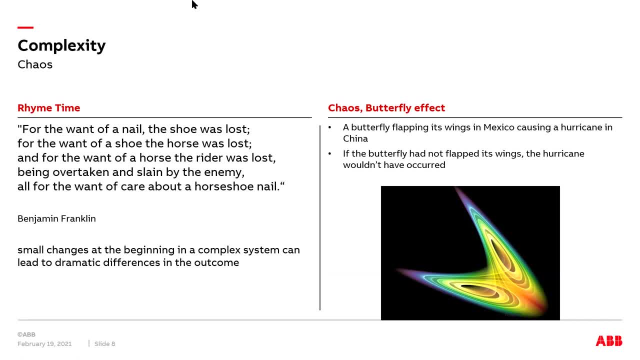 But when we do it over and over and when the system maintained for a long period of time, when that space and time becomes large, a small change can come And that can cause huge change in the outcome. That is what we call as a chaotic system. 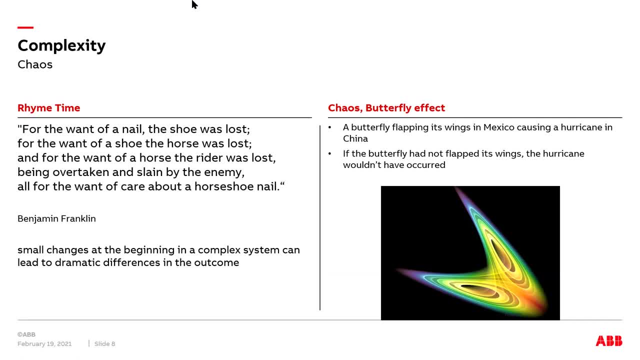 So if you are talking about mathematics, then it is beautiful and it is endlessly fascinating to call that. a system is chaotic- That's what the term to use. You can look at some kind of examples in Wikipedia and all that You will see chaotic system. 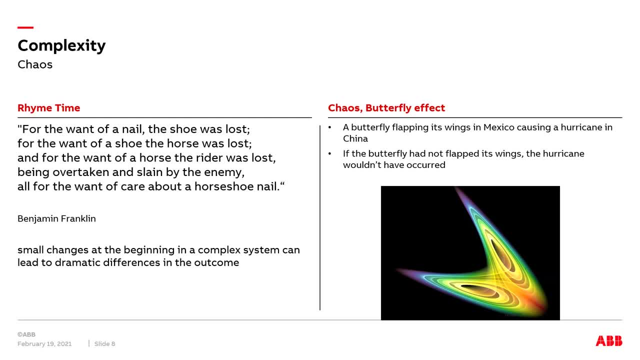 A lot of examples you will see. Some of them are about, say, how the market goes. You may not be able to predict from today, Tomorrow, but over a period of time you may not know what to predict because the system is chaotic. 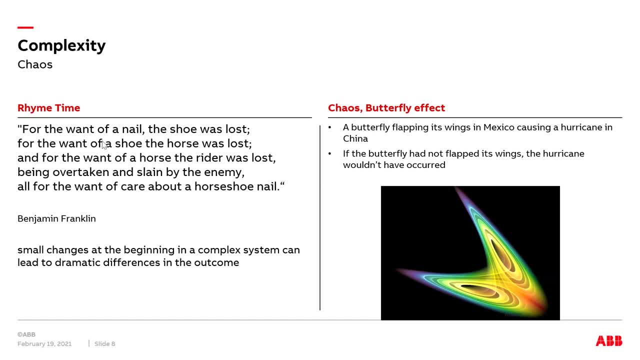 Small change can have a large effect on the outcome. On the right side you can see this is also called the butterfly effect. The butterfly effect is it's a mathematical concept. At the same time, it has a philosophical angle to it. The butterfly effect is telling that a butterfly flapping its wings in Mexico that could be causing a hurricane in China. 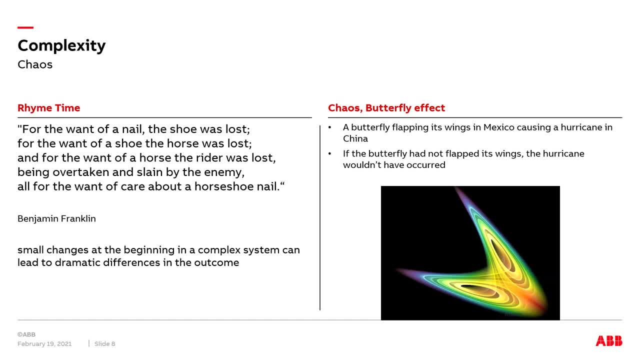 So the way It is telling is that small effect of the butterfly flapping the wing in one place, which is- you don't seem to relate it to somewhere in the universe, But that causes a large change. Hurricane is a huge change. There is no proof to say that this is what is happening. 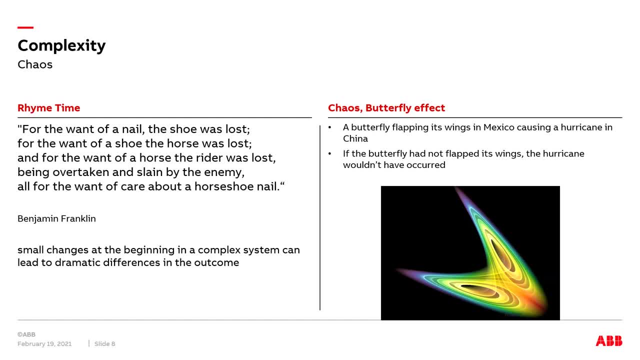 But the principle behind the chaos is this: butterfly effect: small change causing large effect on the outcome. And it's not that the butterfly flapping the wing caused the hurricane. It's not that that is the sole cause Of it happening. Instead, it is like if the butterfly had not. 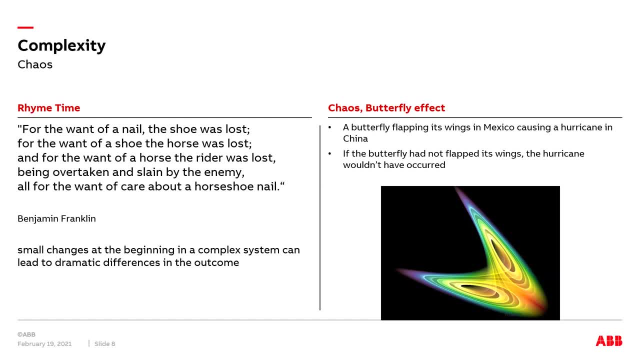 There are so many other factors, but that that one small factor also added to so that the effect occurred. if that small factor was missing, then it will not, wouldn't have happened. So what do you see there is, it's a Lawrence attractor. 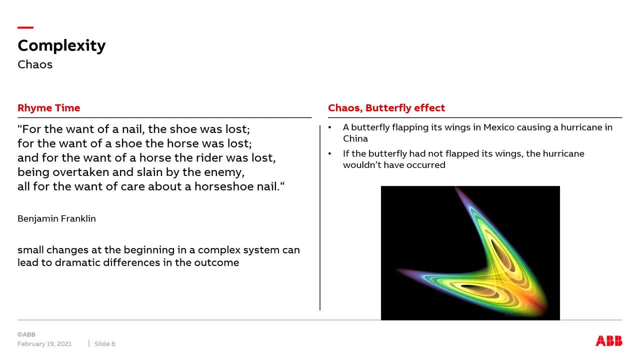 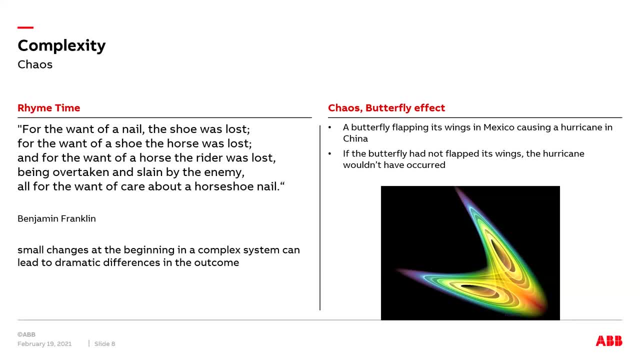 That's what we call us attractors. attractor Like, if you see some example. I'm not popping it up now in the interest of time. I think we may run out of time if I get to do all that- But if somebody is interested, you can look at how we are dual and pendulum works. 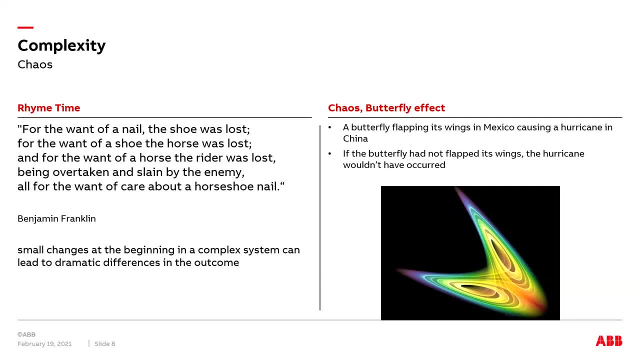 A dual and pendulum is a very simplest example for a chaotic system. Otherwise stock market, even the whole universe itself. Sometimes you could ask the question like if the whole universe was one system, then we should be able to put the whole universe into equations and then we should be able to predict what will happen to the whole universe or a period of time. 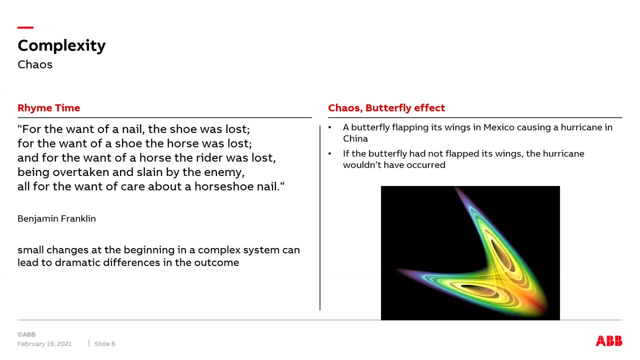 Like, if you look at from a maths point of view, you could say that, okay, like you, you could model your whole universe, but we are not even able to see, do a small weather prediction itself, What will happen over a period of time. 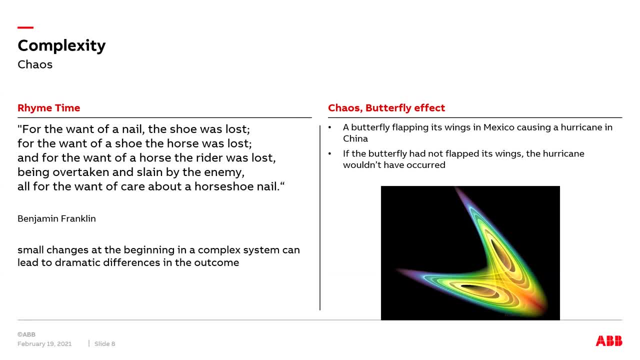 Yeah, Even the weather predictions themselves are approximations and it will be correct for a short interval of time, like tomorrow, one week. But then if you want to do weather predictions over a long period of time, like including things like bigger things, like whether an earthquake or tsunami happens, 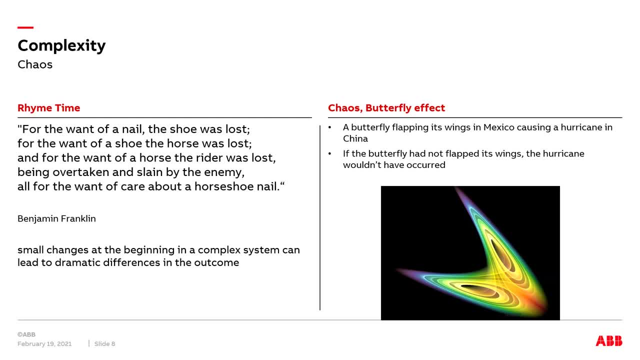 Ideally, you should be able to predict- because it is all- what the acting elements are, what is already there inside the universe today. There's nothing new that is acting. All are existing. There's nothing new. They are only interacting with each other. 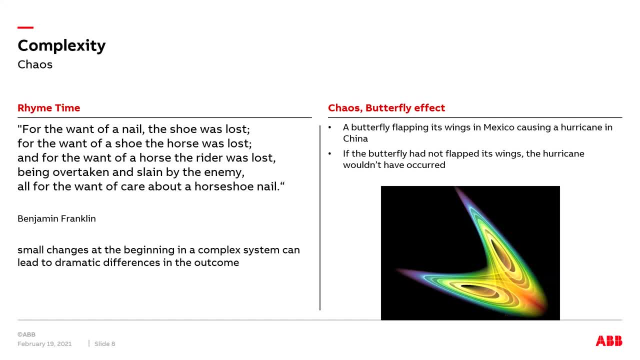 That is how everything else is happening, Even the human mind also. it is only the existing things or what else you are putting inside. It's interacting and something else is coming out. So there's nothing unknown in that sense of unknown, but you are not able to model them. 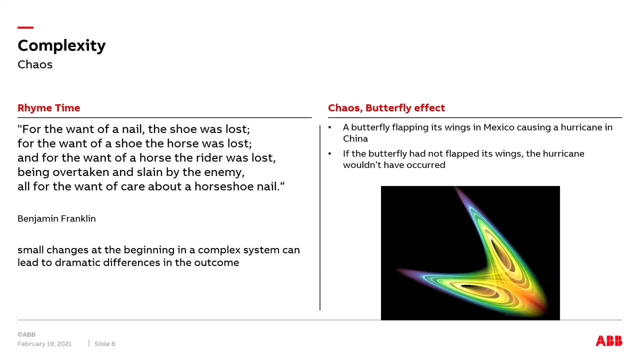 The reason is because of this chaos effect. If you have some small changes in the input, if you have not modeled that small item, then over a long period of time it can have huge effect. So it is something else that would happen. 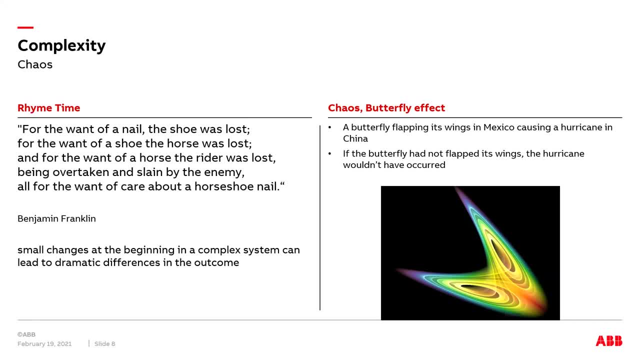 So this mistake is something which makes long time weather prediction No- Almost impossible to say what would happen. And Lawrence Lawrence is one person who had worked. It is a mathematician who has worked a lot of time into it. So you will see this, Lawrence attractors. 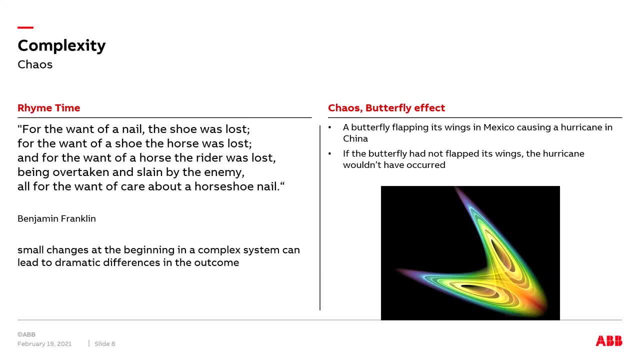 There are a lot of attractors which are, you will see it, in this chaos world, And when the attractor itself is a fractal means it is having a self similar pattern. when that attractor itself is a fractal, That is when you call them as a strange attractor. 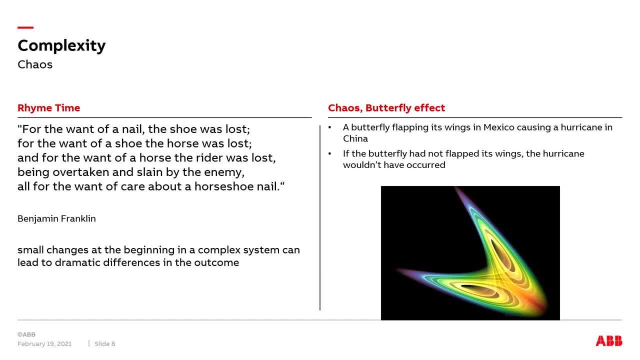 I think I'm introducing too many new terms, But then just to understand that these are the way of looking at it. And then about the I told about how, about looking at the whole universe as a system and then model it, and then we come out with it. 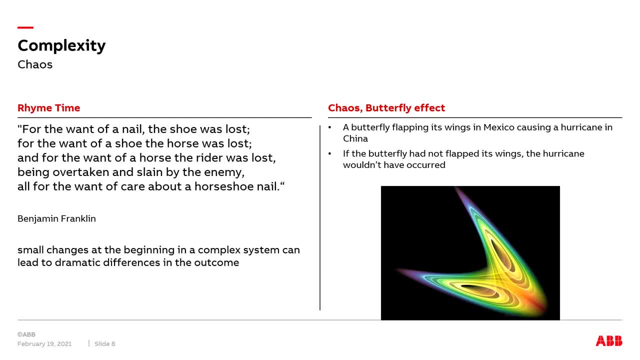 It's. it's a very weird, wild idea to talk about. Not practical, not possible to me, Can I? but then, yes, Can you just explain what is an attractor? Attractor is a system, a chaotic system, a chaotic system over a period of time. 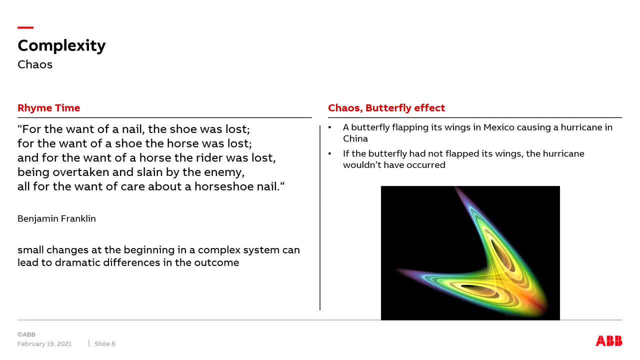 Yes, It will converge into one place. That is where you call us an attractor. where it converges to, that is where we call it as an attractor. A chaotic system will remain chaotic, But at some point it will get to do. you can identify patterns of emergence that would happen in the chaotic system, or a period of time. 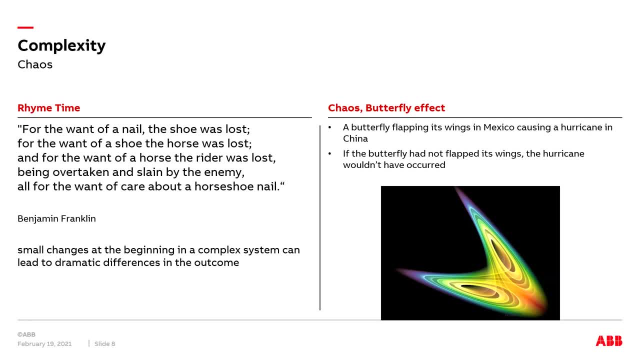 So emergence? you could look up even the term called the emergence in Wikipedia or somewhere. So this is a phenomenon that we call us emergence, like something which you have never anticipated, like properties, new which you never thought of come out. Some people like these are team building people or the soft skills traders, also by, to use terms like team synergy, like you may say that, okay, it is like one plus one, maybe more than two. 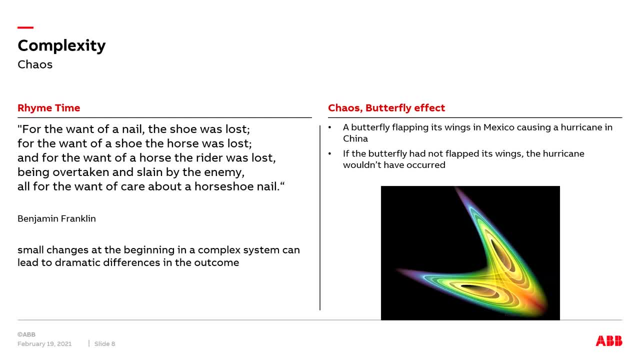 It's not the more than two, like over a period of time. if you apply this emergence philosophy, new things which you have never anticipated will come out. Did I tell you? Okay, okay, Sure, These are properties of Generally what we from chaotic systems. 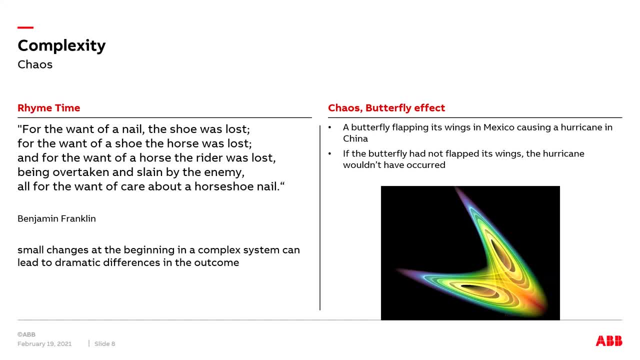 So then, to come out with this, this was something which I learned recently. if you look at, if you say that, the whole universe, you cannot do the modeling. If you look at us computer science engineers, we have a tendency to look at our as programmers, we have a tendency to look at: okay, we put it into a variable. if it is not possible to put it to an integer variable, why don't we put it into a real, real variable floating by the variable? 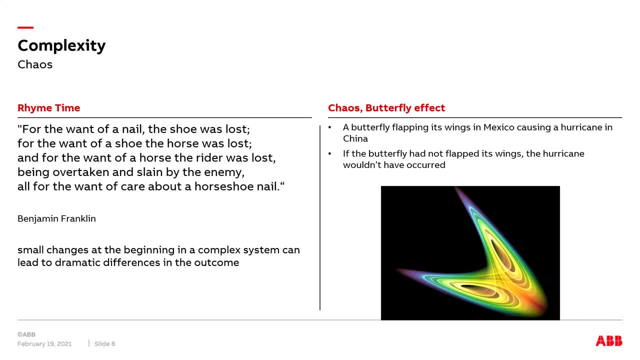 That can hold even fractional values, but then that is only limited precision that we can do. we cannot go and put 10.0000 at one or two or whatever. you can go infinitely there. So if you are really interested in understanding this, 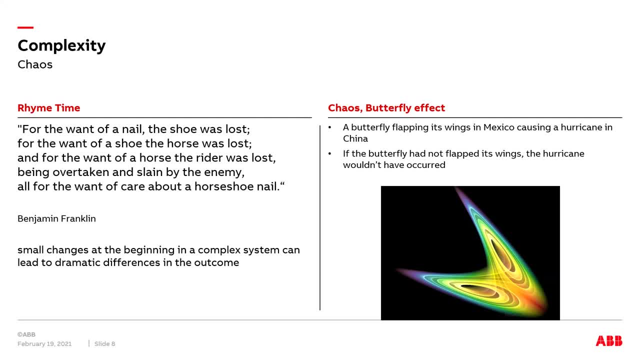 Real numbers. there is a principle which is there available- they are still in these university professors might talk about it- that we call it as a bss model of computation. That is the name of three scientists- some blum, somebody or The other. 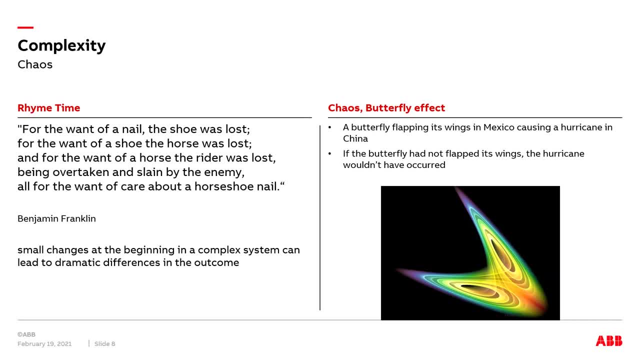 know this bss model of computation is: how can you do infinite precision, real numbers, because real numbers, unless you are able to do an infinite precision, your model has lost that a small values. so if you have lost the small values over a long time, you will lose it. 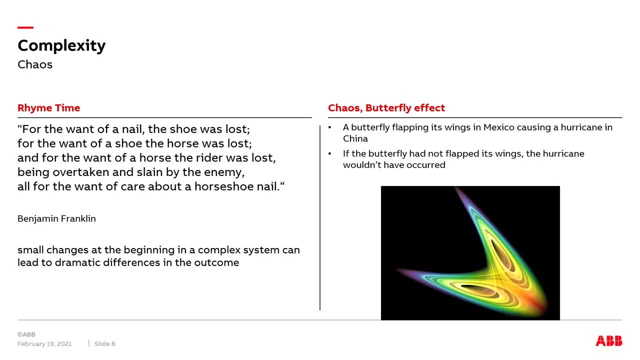 So this is what we are talking about from the concept of complexity, chaos, butterfly effect, these are all the concept around the This front front factors, But ultimately it is the same same concept you are talking. if you're talking of complexity, small changes in the beginning of a complex system can lead to dramatic difference in the outcome. 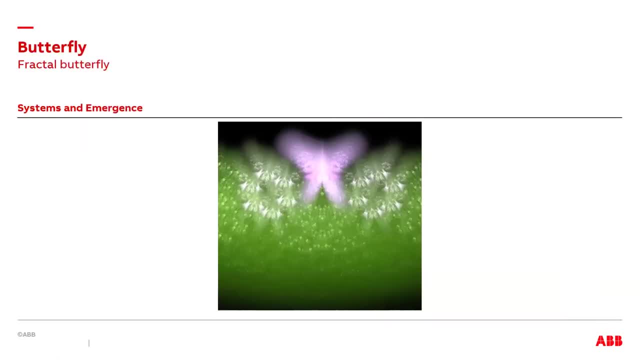 Sometimes this is some pictures which I have created. so systems and emergence, so new patterns will ever, sometimes what like? sometimes I also have a personal way to look at it- a little bit philosophical batter, Like when we are doing some action we think that, Okay, well, let me help that. 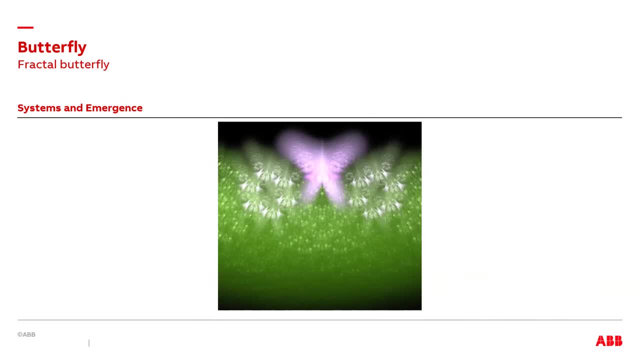 person. I don't know whether that is working or not. we do not know about us- happened actually, ultimately over a long time. what has happened? maybe you would have explained something to someone. even today i'm doing this session. I have no idea what would happen over a long period of time at the end of the session. so you may say it was nice or not so nice, or interesting or not so interesting. 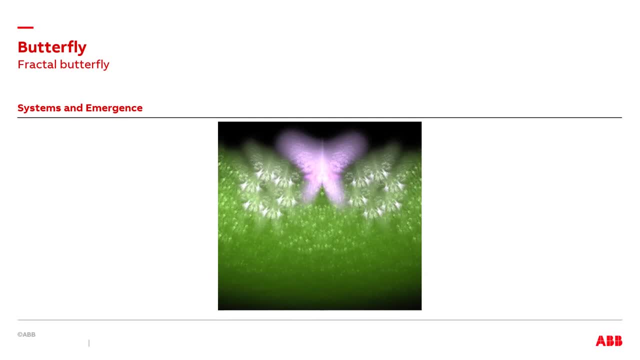 But then what leads to anybody to go further and do something like? we do not know. so you, whatever you were supposed to you, you just do it like and then you continue. the effect will happen over a long period of time time. Sometimes it takes away the discouragement of not seeing results immediately. 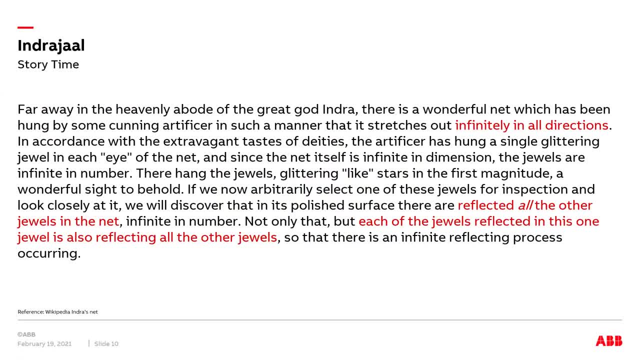 So that is all about, and now let us look back to mythology. I also have a habit of reading about these mythologies and fairy tales and all such kind of things. So if you see mythology, the only thing which I have come across in the mythological manner about fractals is 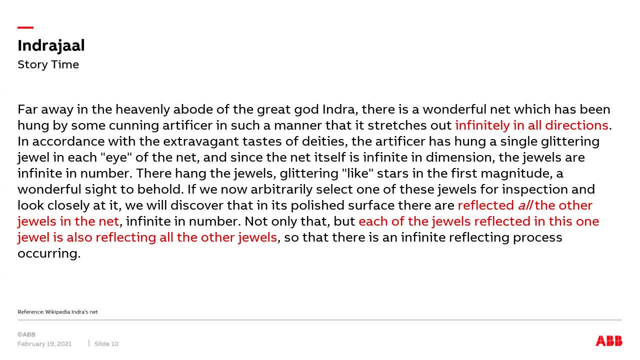 this is the only one item which I have come across. This is about that magic Indrajal that we're talking about. The term Indrajal is coming from a place, from that Indra. that Indra is there, right, Lord Indra, That Indra seem to have a net, So this is the best description. 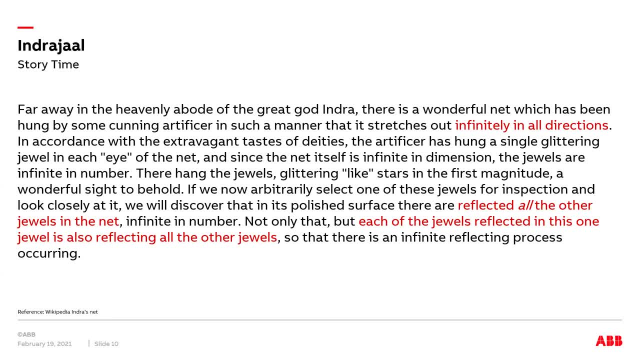 which I could get from in an English version for the Indrajal. So the way this is the description of the how that Indrajal net is, It's like it's telling that these are that net is made of pearls and those pearls reflect each other. 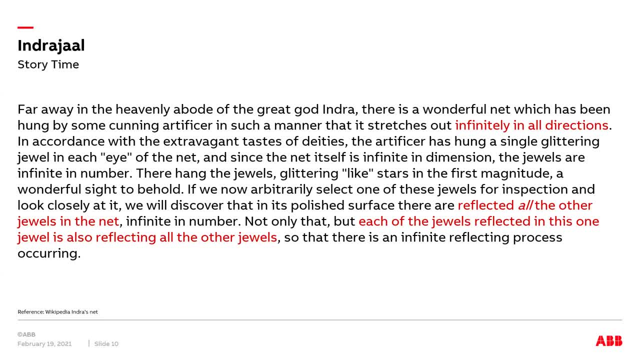 So what you will see is- I don't know this is a very long sentence, but still some of the lines I have highlighted and kept. So they are saying that they hang the jewels glittering like stars in the first magnitude. It is a wonderful sight to behold, Like if we now arbitrarily select one of these jewels. 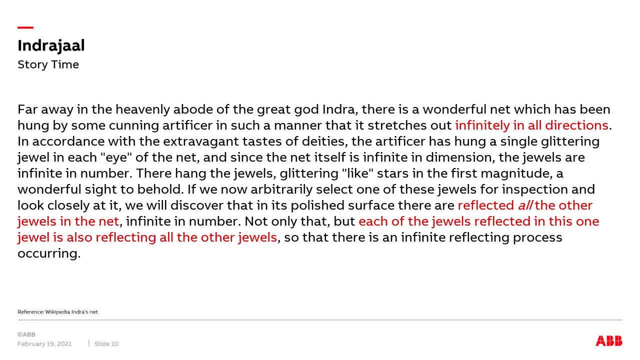 for inspection and look closely at it, we will discover that in its polished surface there are reflected all the other, all the other jewels in the net infinite number. Not only that, but each of the other jewels. there are actually not the same details, It is not even effected by the 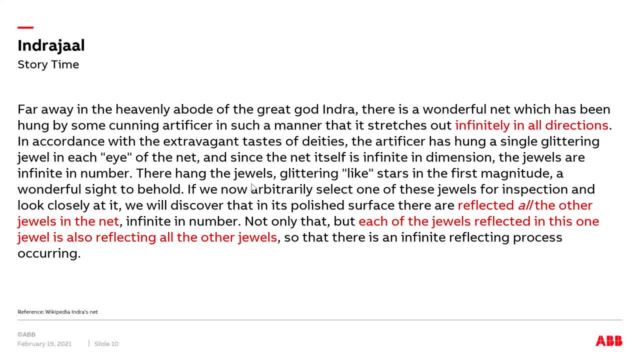 other. Well, this is the place from which that Maya Jalli is coming The like. so you cannot really comprehend what is happening because you are seeing one. but it is that the whole or is that the part? like we are not able to make out, because I do have an interest in stories. 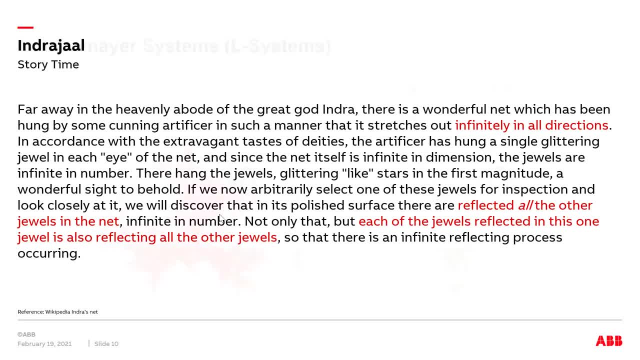 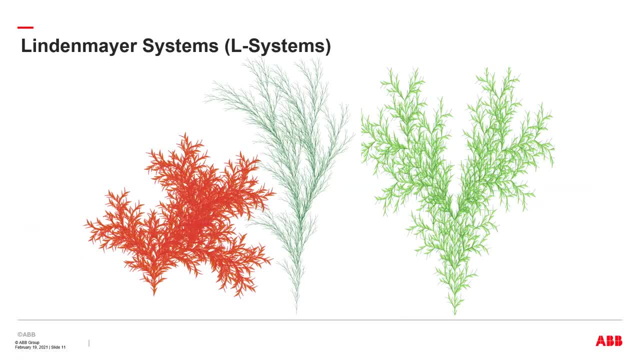 That is why I got into the story part lindenmayer systems. this lindenmayer systems is one which we see it in. this is the very simplest of the way to look at fractals. this is one person named lindenmayer. they have 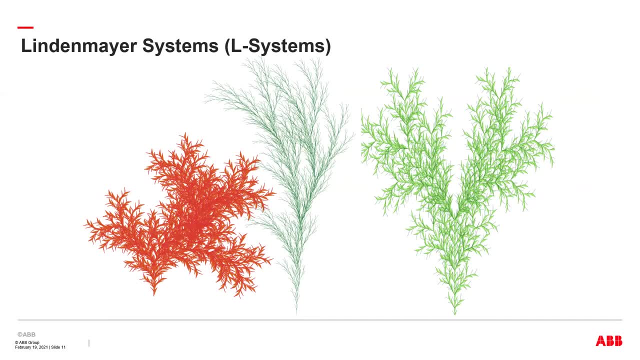 found out a model of the plant growth. this is a biologic biologist who have come with and put all these lindenmayer systems. this is all about plant growth so we can describe how a plant grows. it's a parallel rewriting system, so you write one structure, then you 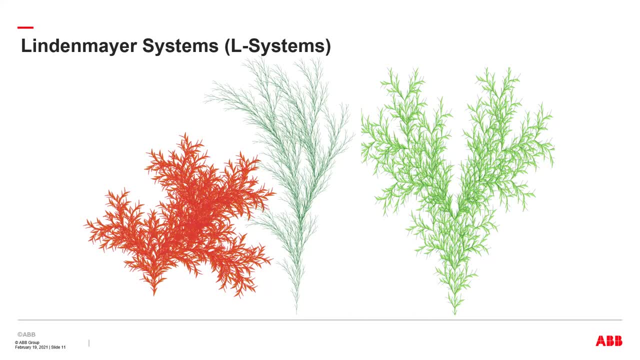 keep repeating the same structure again and again. like there are programs, these are done with the pictures which you see here. they are done with the lindenmayer system, plugins from this graphics program like inkscape. this is done in inkscape. yeah then. so they have this recursive nature. so it's like tree branch: you take one branch. 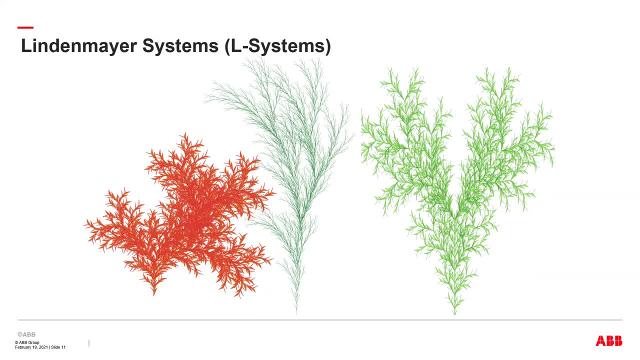 that branch, one part of that branch, gets replaced with an entire new branch. so this is where the self-similarity comes. these are fractal like forms. i don't like being a purist. i don't know whether to call it this. is not coming from the complexity- part of the fractal- but 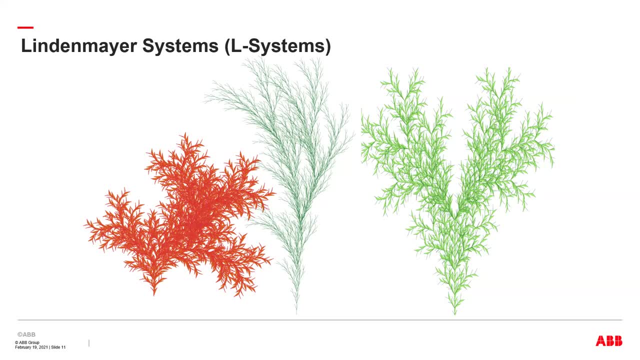 these are more of repeating the self-similar pattern. so fractal in itself is about self-similarity. so these trees are giving you a feel of how self-similar patterns come and how tree growth is modeled. so l system. these are popularly known as l systems, so if you look at somewhere and then see wikipedia, 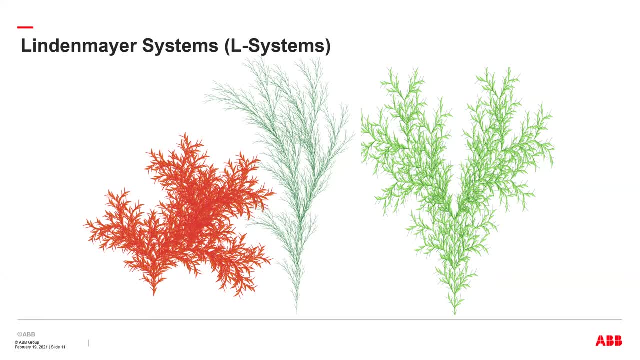 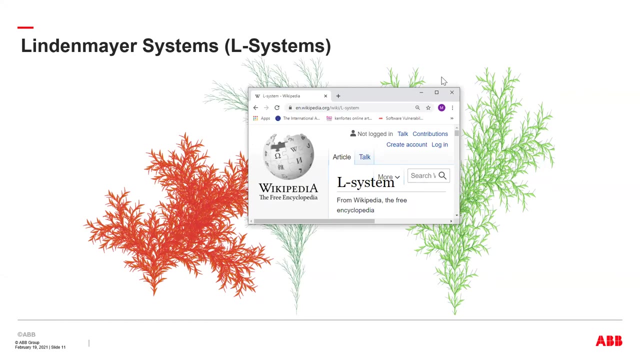 also, you can look at wikipedia l system. maybe i'll open it right away. so there's a grammar that they use for okay, so let's see, see. you see these kind of trees that you can grow by using this grammar. so what they do is they are replacing. 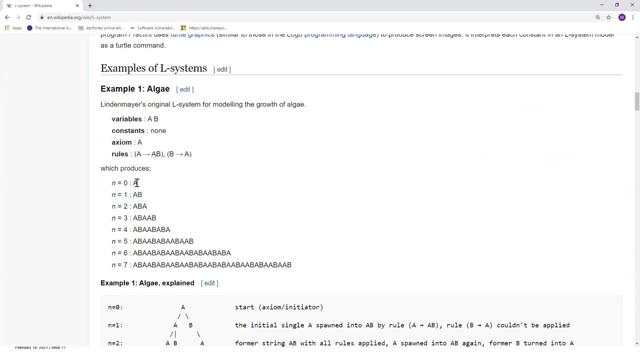 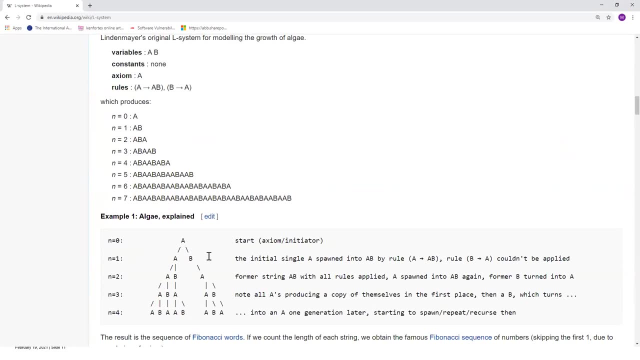 see these kind of patterns. you, you start from somewhere, so you have a, b, a, b a, then you keep replacing and then keep adding, so you will keep building this pattern. so over the time, what you keep building, you will get trees and patterns that you want and you can define. 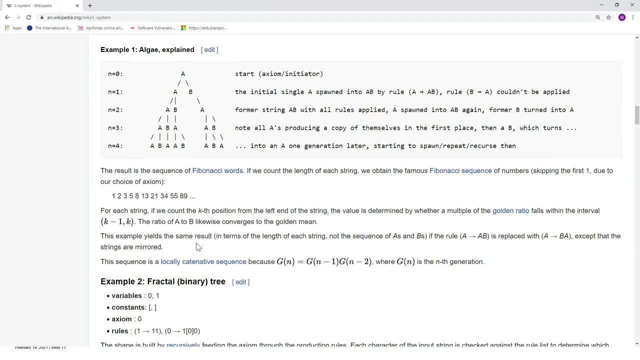 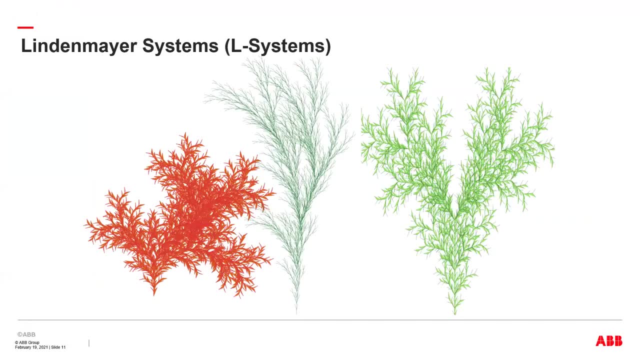 how you want, whether you want to do a blanky factor or whether you just want some polynomial way of doing. you can do many of these things. this is the biology part of it. how plant growth, this model. you can do many of these things. this is the biology part of it: how plant growth, this model. 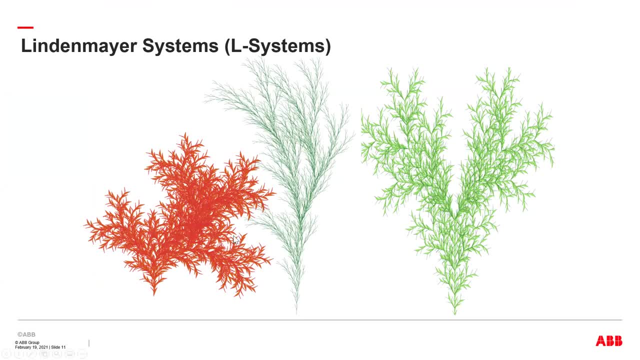 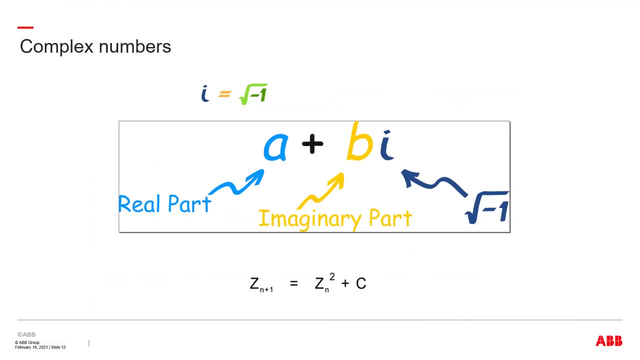 you can do many of these things. this is the biology part of it. how, plant growth, this model, very simple structures and the method behind is also very simple. and now let us get into this. complex numbers, how, these, the complexity and the complex numbers. this is coming from the complex number, only that complexity is coming that small changes. 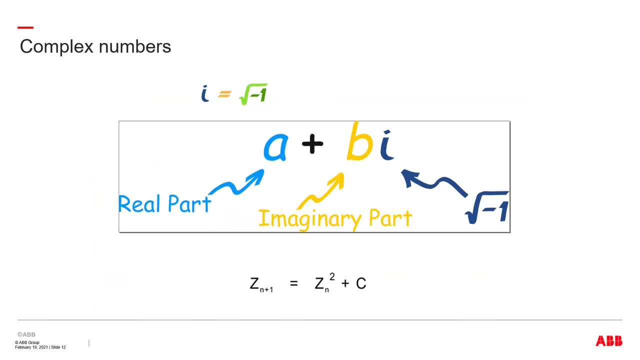 and large changes to the output. this whole concept is coming from complex numbers. i believe some of you, at least coming from some we have started educational background, will be understanding what is a complex number. so, in that what we are talking about, there is an imaginary part, what we call as uh, like the i, that is square root of minus one, which you cannot compute. 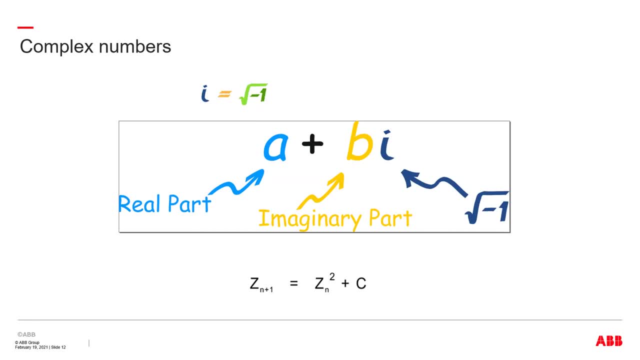 that square root of minus one is where all this complexity and complex number comes, in that you will have one real part and then we will also have an imaginary part, and the imaginary part is one which contains this square root of minus one. so this is the basic representation of a 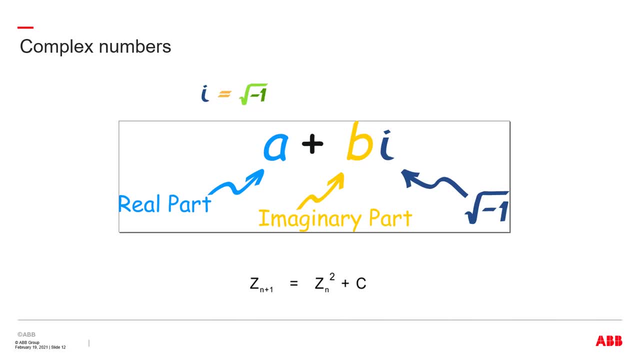 complex number like nothing new, many of you know, but this is what really gets you into these fractals. what will? what happens is a whole lot of magic comes into picture when you begin to iterate over these complex numbers. so when i wrote this cn, it means the n, c, n complex number. you, you take. 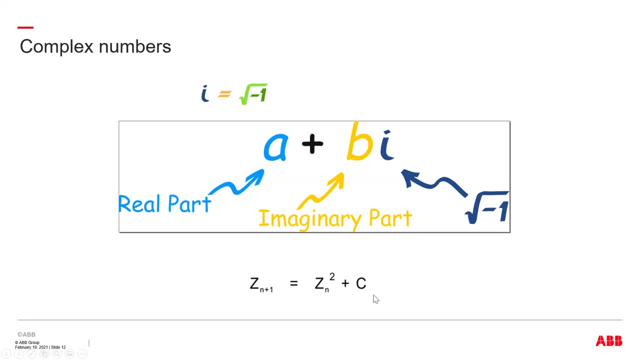 any number, say c 0 or c 1, so you square that number and you add a constant to it. the constant could be real or complex once again, and you get a new one and then you keep repeating. it's like a for loop. you just put a for loop and then you say: okay, if you say that this is the one complex. 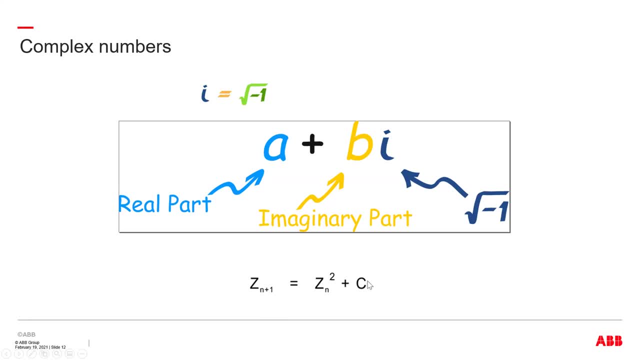 number, that complex number equal to previous complex number squared and then added one constant to it. that's what the iteration that we are talking about, the same iteration that we talk about in our program, the same for loop and while loop. so this is how we keep iterating. 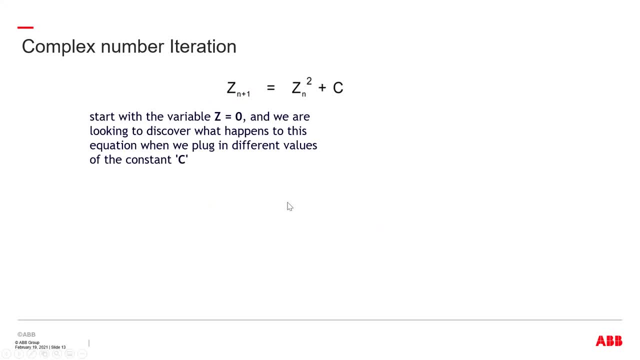 so now, when you keep doing this iteration, you can start with a variable, that is your complex number c. you can put a zero and then we are putting a constant to it. you square it, then you add a constant to it. that becomes your next number, then you continue. 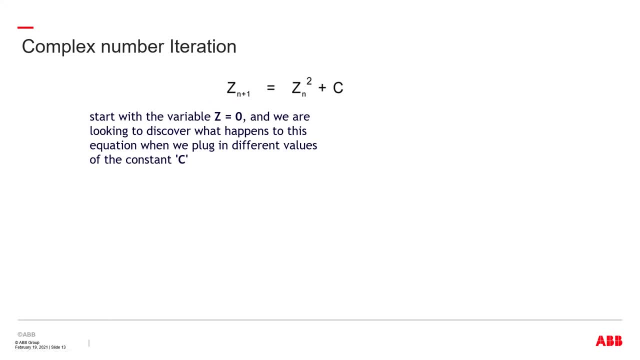 so this equation of iteration that will give you very beautiful patterns, that is a item which i am going to show you right now. so what? we will see some examples how they will get into if we plug in different values of c for this constant. so let us look at. 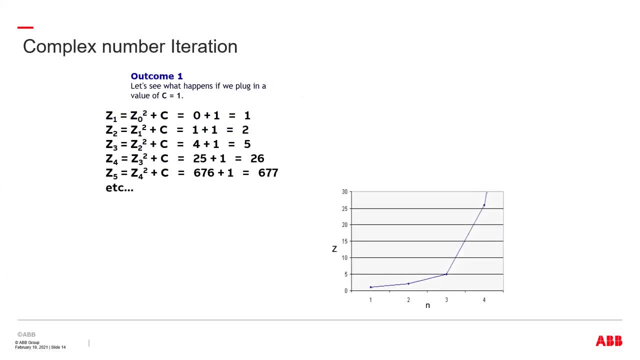 one outcome. this is nothing. you will not be surprised by seeing it. but then let's understand. it is the same principle. so you take the c 0 square plus c, so we will start with 0 for your complex number part, and for the constant part let us look one. 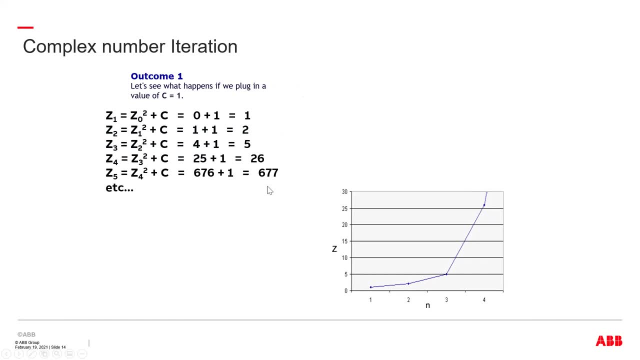 like here, the imaginary part is zero, it is fully a real world part that we are talking. it's all real numbers. so what will happen is: you do one plus one- you keep you square- and add, then you will get a two. you square and adding, you will get a five. you square and add, you will get. 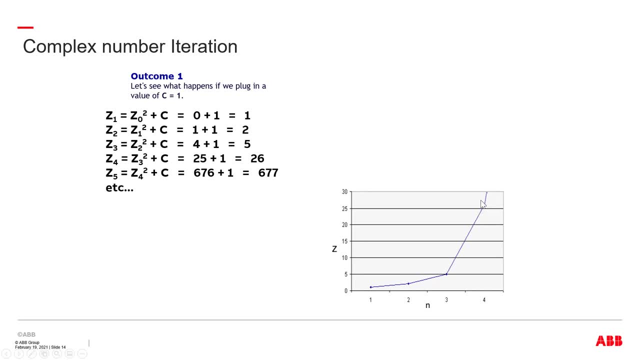 number, you square and add and you keep going. so what will happen is it will explode too quick, the the number grows too fast, and then they grow too fast and it will go out of your control. so you are not able to do anything because you are not able to compute, you are not able to. 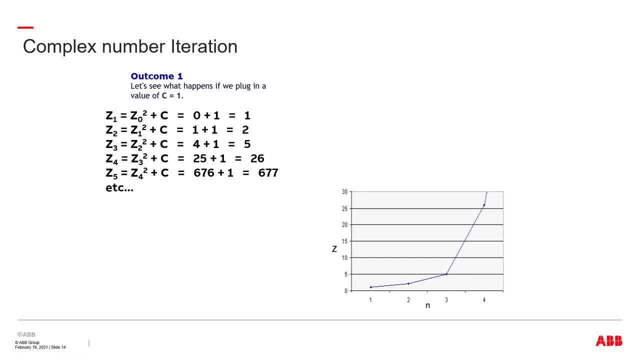 hold that number. if you are doing, say, 10 000 iterations over this, or say 100 000 iterations over it, then you can't hold it. it is all somewhere. that's what you will see if you are looking at. this is your starting condition. and now let us see one more starting condition. 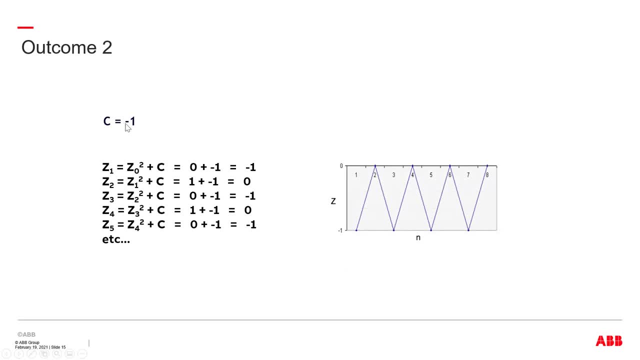 say we start with a minus one, you start the constant to be a minus one. then you say c, square plus c. so you zero plus minus one, minus one, see minus one. you keep square. and then you add, square, the previous value and then add once again the same constant, minus one. then you've got a zero. 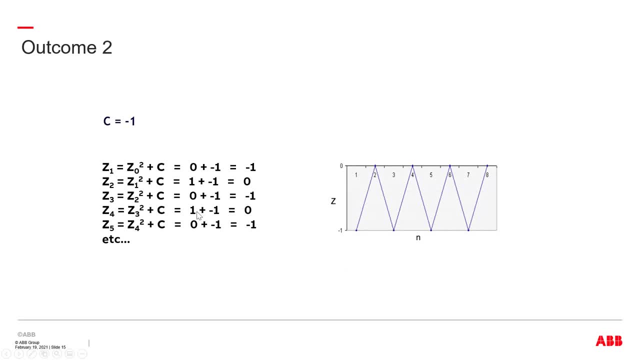 zero minus one, you got one, and then that minus one square is one again, and then another minus one, you've got zero. like you don't have to go too far. you see that the same thing is repeating, so it is just oscillating between two numbers. here it's just going between minus one, zero, and then that's all what is. 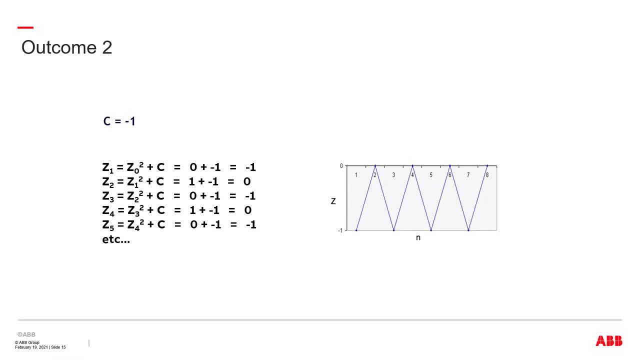 happening here. so this is your outcome if you start with minus one. i'm not telling any complicated mathematics, it is just basic. you square a number and add another constant to it, in fact, the whole world of these fractals and complex numbers. the equation is very simple like this. the beauty is 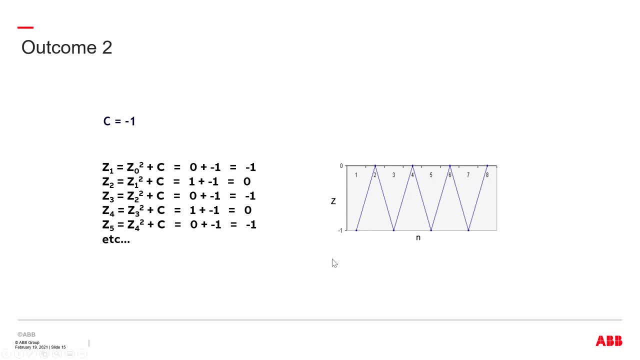 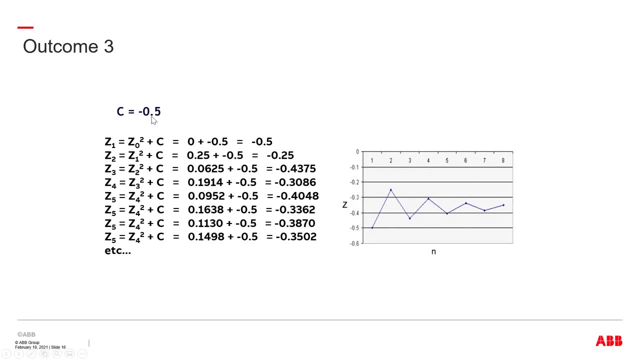 when you keep iterating and keep doing it again and again, and then this is another pattern which you will find it very interesting. so here you start. you start with a minus 0.5, a fractional value. then what you will see is the number keeps oscillating between some constant, but the value is keeping on coming down and coming down. 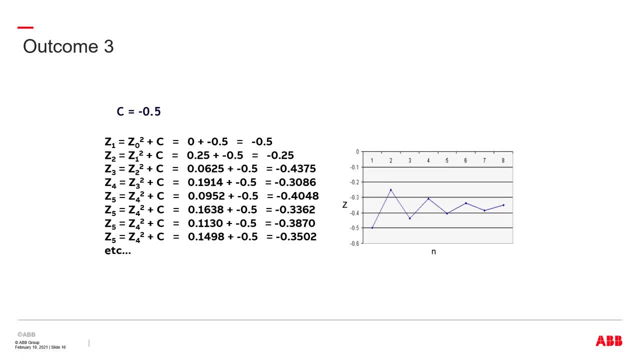 and here what this is, where your iterations becomes more beautiful. here what happens is the number keeps reducing, but it will never reach c 0. But then it is keeping on reducing. So your dimensions will keep reducing, but then it never reaches 0.. And how this fractal or that Mandelbrot set came into is: if you keep. 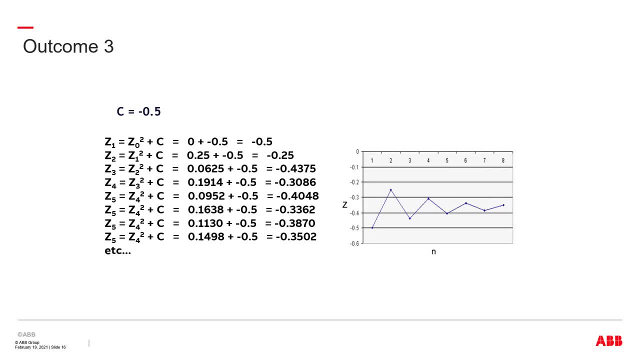 iterating this over a period of time. and if you keep plotting it like how you see it, the patterns will keep repeating itself Over a long period of iteration. they will repeat, But then it never reaches 0. It never disappears, but the pattern keeps repeating itself. So 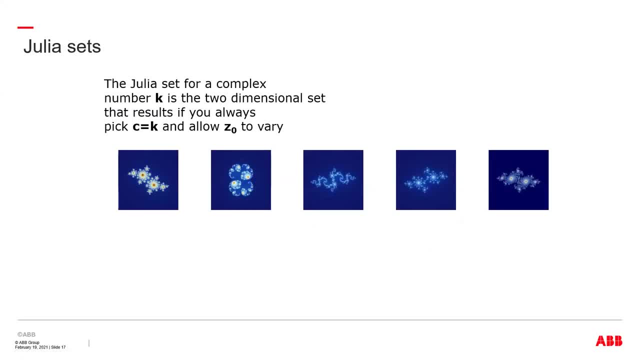 this is what we will see here. In the previous examples which I show, you will see two things. we will see here: Julia set and Mandelbrot set. I know some of you who are so much fascinated by digital signal processing and all. I think you would have some familiarity with Julia. 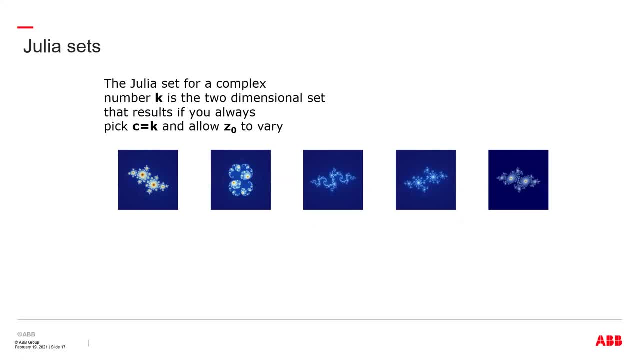 sets. So this Julia set is what you are seeing here, For the Julia set is one where, if you start with the C, if you allow it to be a constant K and then if you keep the C0 to vary from your starting point, that is where you will get a Julia set. 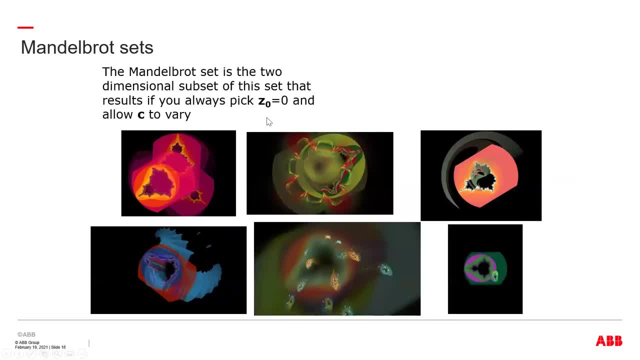 And the Mandelbrot set is also very similar. This is the Mandelbrot set picture, where you keep your C0 as 0, start with the complex part as 0, and then you allow your C to keep varying. 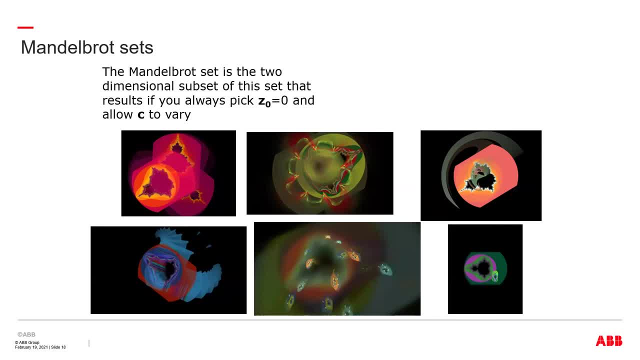 The variable which you are iterating over, you are putting starting point as 0, and you keep the constant part into another complex number, and then you keep doing. that is where you will get Mandelbrot set. So what you are seeing here is the various Mandelbrot set pictures I have created over time. 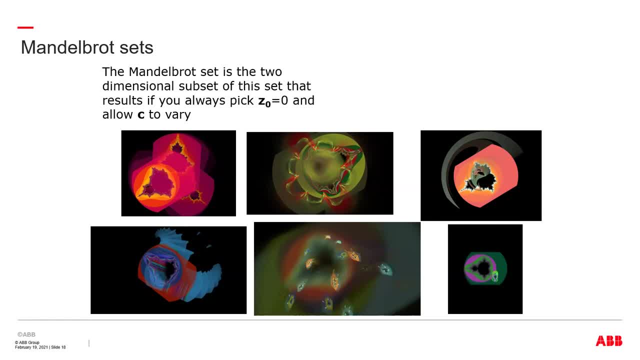 At some time when it was November- sometime is that Mandelbrot's birthday time- So at that time, out of fascination, I had created all these Mandelbrot ones. So this is based on your starting point. you will get varieties of these pictures. 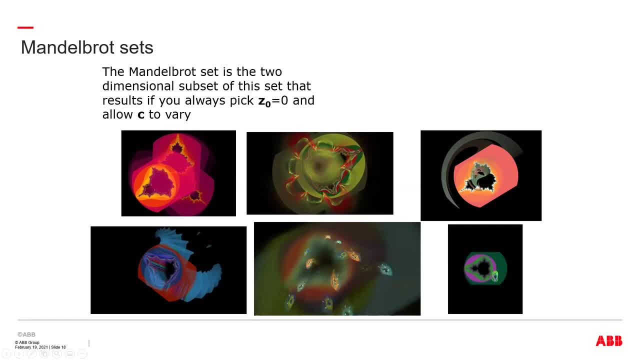 That's what You are seeing here With me, or confused. Hello, My audience is there, right? Yeah, Okay, so this is the Mandelbrot set, Thank you. So get these two terms. One is this: Julia set and the Mandelbrot set. They are very close by based on how we are starting and how we are doing it. 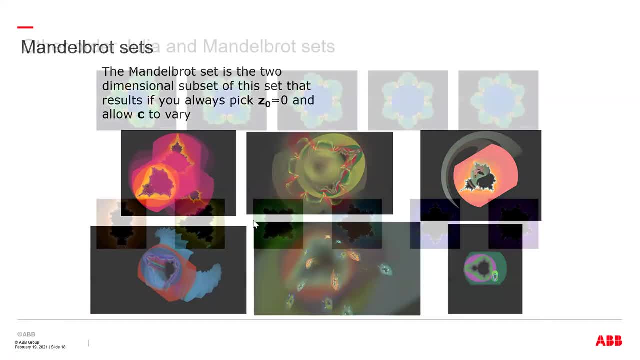 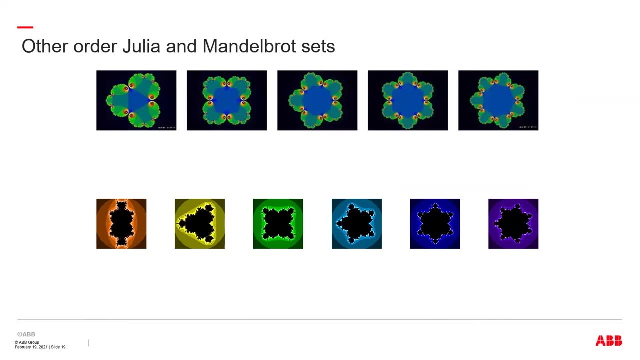 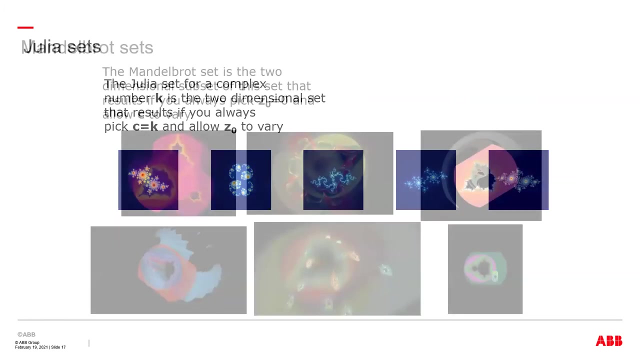 Okay, so same. Let us in questions. Many say: how did you create a ship pick Pardon? How did you create the ship Palin, Very shifted ship, Which is ship This one? Are you talking about a ship? Yes, 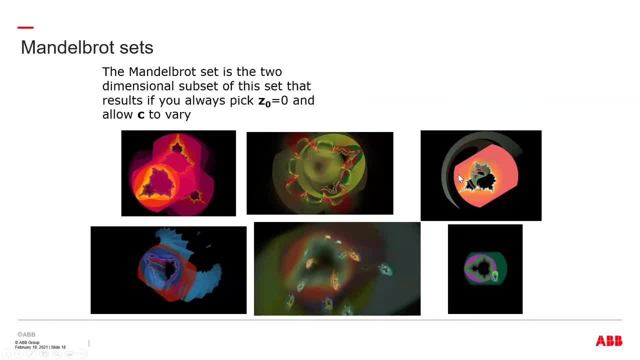 Yes, Yes, Yes, Yes, Yes, Yes one: the orange color should be fish. this one, this is also a model broad set picture. in fact, i'll show you some. yeah, no, no, no. from second row middle, this one: yeah, that is also a mandelbrot one. 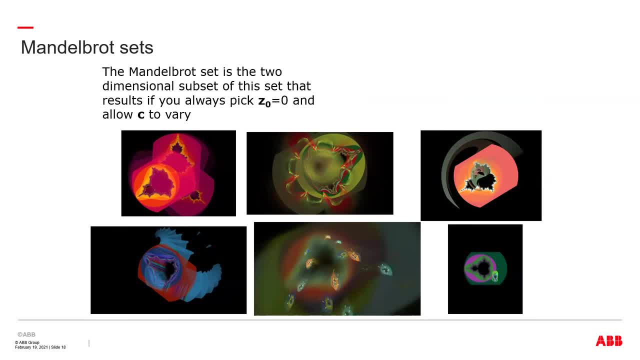 see, these are all varieties of mandelbrot pictures, only the same information. oh, this one i have done with a tool. there are op. you can write python code. if you are interested into python you will see enough of open source code. uh, for mandelbrot set. you can take it you. 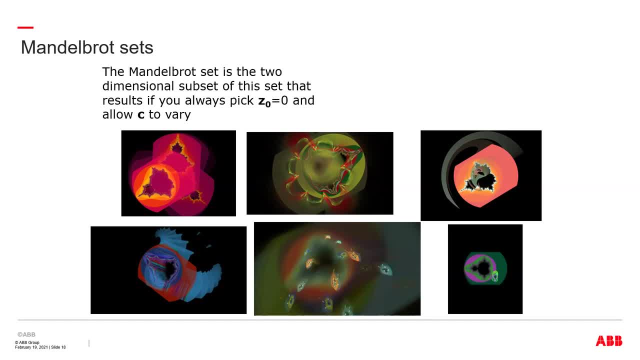 can play around, you can put in python and then you can see that i will have some programs written in python here. but these pictures i have created using a tool like the tool which you can feed in your starting point and the tool will do the iteration, like you can tell your equations into. 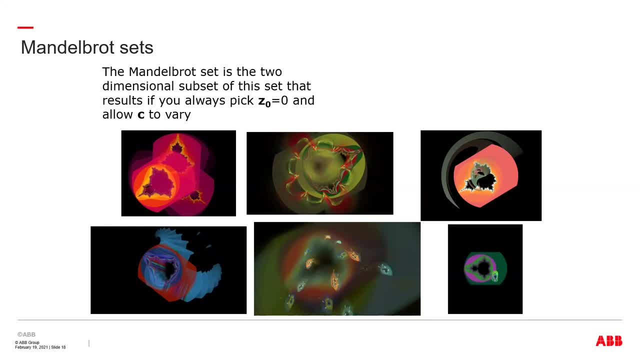 the tool and then do that. so very simple programs like for drawing mandelbrots. you will see them in the git or anywhere you just search for a mandelbrot set python program, you will see enough of them. like cocalc, cocalc is a sageman. there was a program called sage math, if you know. 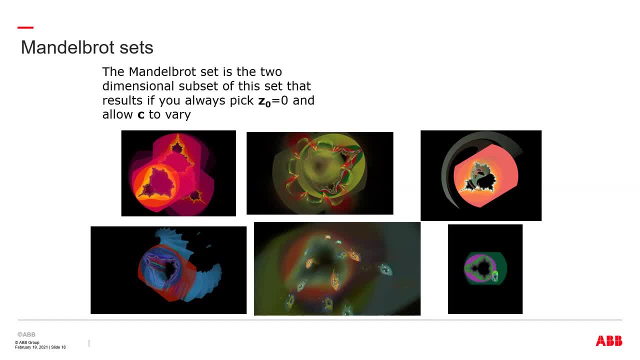 which was a cloud-based mathematics program which they have rebranded it to and they call as cocalc. that is also a place where i keep playing around so you can write the program will be hardly five, six slides- and then have some graphics plotting like how i had put it before. 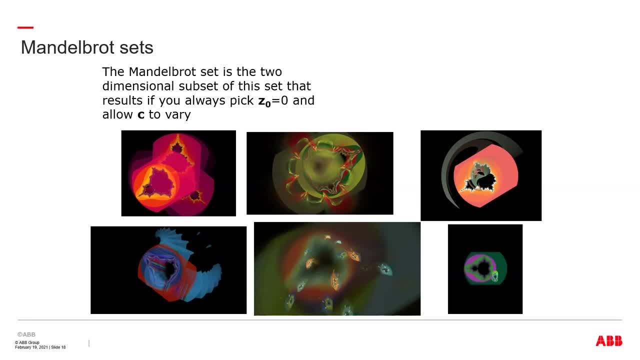 right, i put some turtle graphics, so get some graphics for plotting it, then you, you can draw any of these for creating these pictures. but i have used the tool and then done it. okay, uh, one more data actually i want to create from my image i want to convert into mandelbrot. 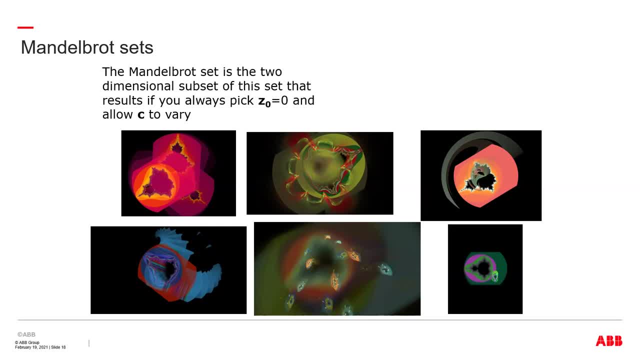 set. so, for example, yes, read it, tell me again: image to mandelbrot, uh, yeah, yeah, for a normal image, for example, there is a home. if i convert to mandelbrot, uh, i will get multiple homes like the one you see in middle, one multiple i will get. i got it, i got it. okay. see, yeah, you can do that also, in fact. 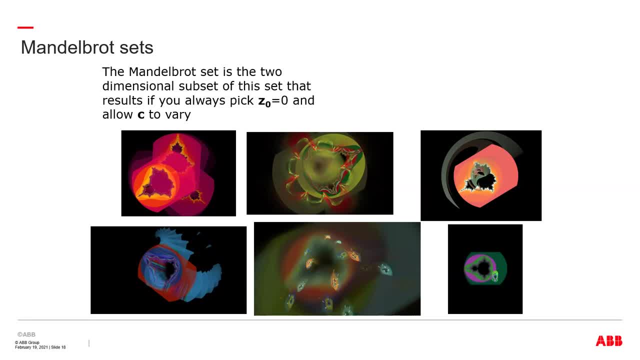 some of the pictures when i show you, you will get that. what you? so what you want to do is you want to take one picture and then you want to distribute that over a mandelbrot pattern. yes, you can do that. you can write some programs to do that, or even the program samples which i 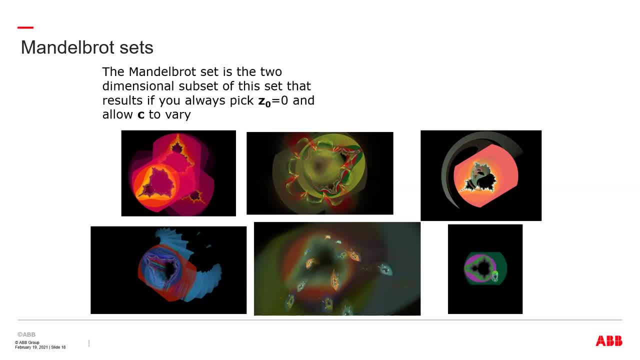 but you need to spend some time. okay, like because they you have to adjust that weight how it will look like? definitely you can do if it's easy. can you show a demo how you created that, this one, that middle one, second row, middle one, the tool, how you create it, how to create? right now, i don't 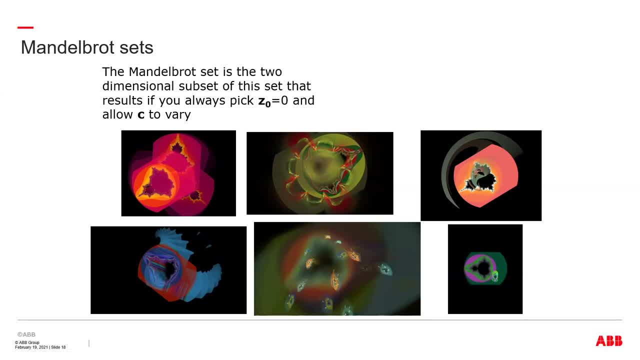 think i'm prepared to show that, but maybe we can. i'll show you the tools which i have used. then, yeah, i'll show you the tools, because i think that will take a little more thinking. right, i should have mentally been prepared to. i prepared those material and kept it ready where it is: the program, only one program i kept. 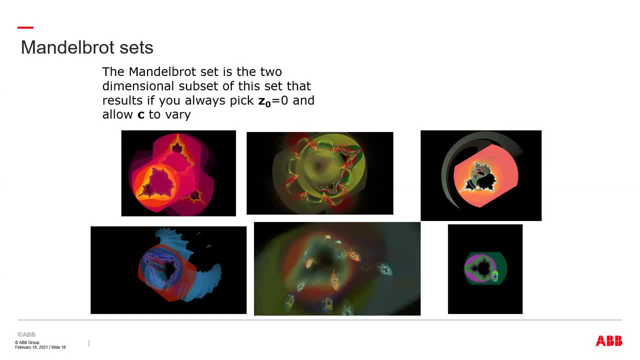 it there. i didn't keep so many programs ready in hand to for this session purpose, but just google around, git also- you will see enough of them. so you want to create a mandelbrot set, individual pieces containing all this. so why it is all different, different shapes. is it because it's varying that? 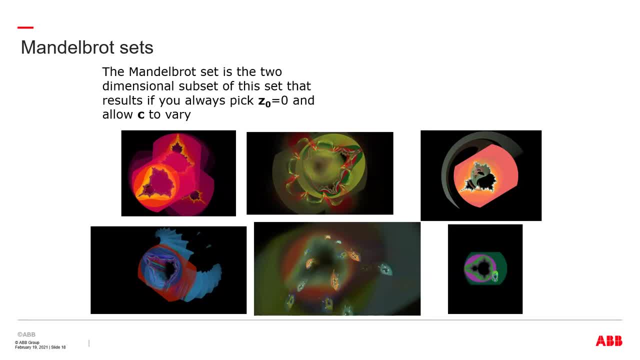 complex. it is very. one is complex, part is varying, and this is also. there is something that is called as a fractal flames. these ones are created using a fractal flame. i'll show you later as we go along. a flame is a way where you can mix a lot of fractal. 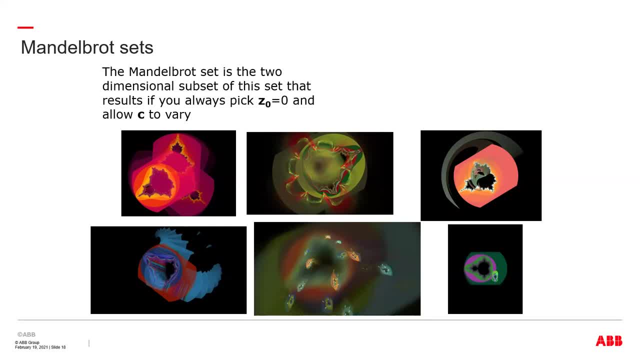 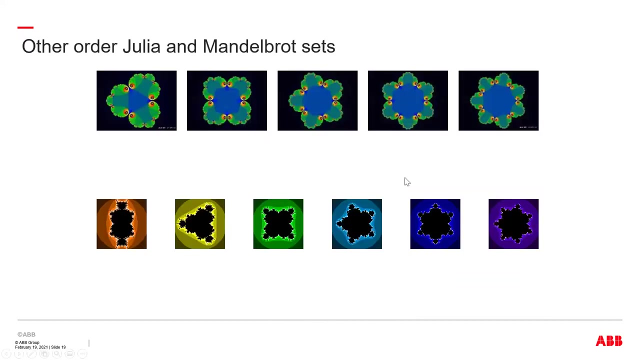 equation, make mix of transformations and then you can render them all together. but we'll come to that. there's an algorithm for that fractal flame. that algorithm i'll show you. hold your curiosity. you are asking too detailed, too early. go ahead. yeah. so these are the picture which i am showing here. see when i say higher order. 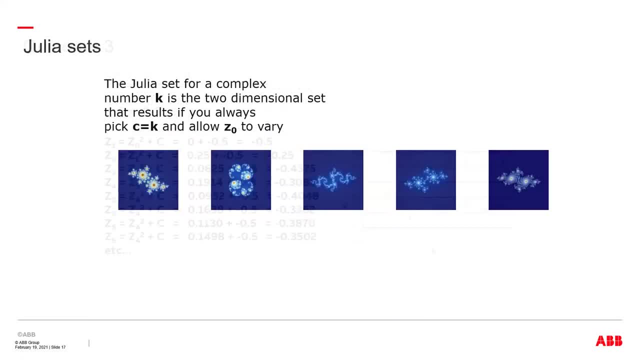 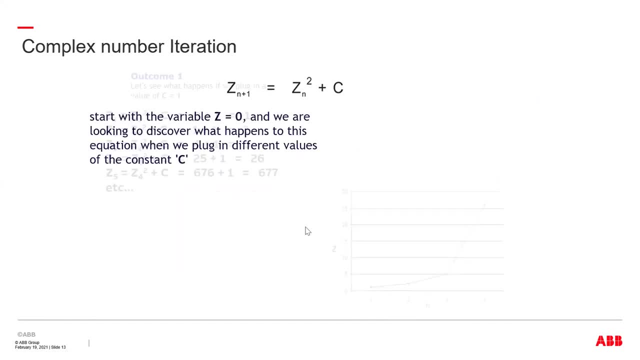 what i mean is: see, previously we told that we will square it. what we told is we will square that number, c square plus c. see, instead of doing a square, what if i do a cube? or if i do a fourth power or fifth power? so if you keep doing that, you will get. 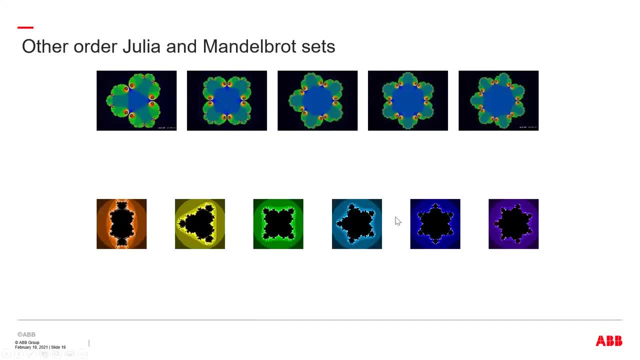 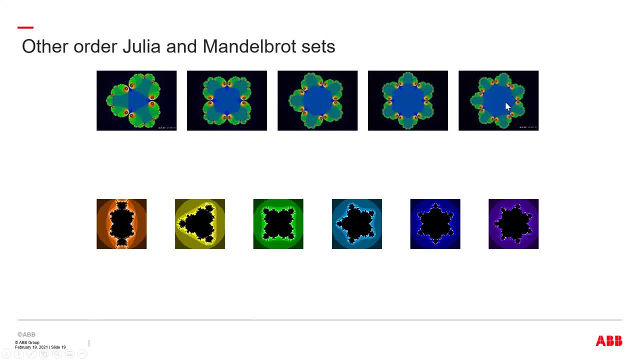 then you will get these kinds of higher order pictures. So that is where all those flowers pictures you see there, many of them are higher order Mandelbrot or higher order Julia. So these are like an order of three, order of four, order of five. that's what you are seeing. 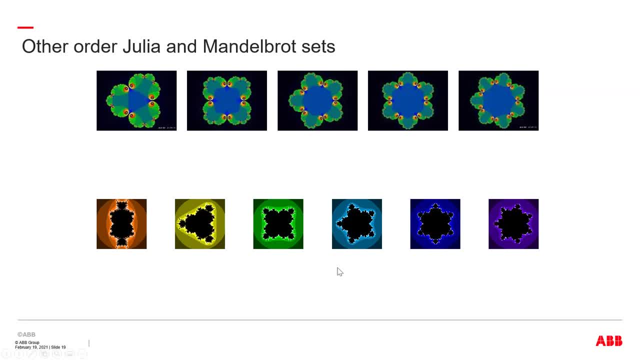 So like this, you can keep going with a higher order Julia or a higher order Mandelbrot. Okay, now let me listen to questions and anything else that we want, And programs: okay, I'll show you some program later, Ranjini. any more questions are there? 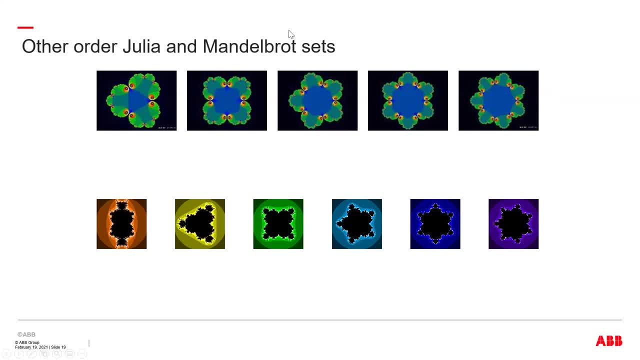 or should I look at the chat? I don't see any other questions on chat. Okay, let me give a pause. I'm waiting. I think we can continue. Continue, or should we take a small break and continue? or because we have planned for two hours? 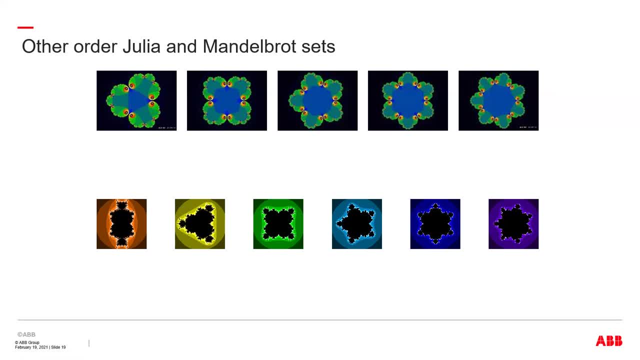 So should we have a small break and continue, or continue as it is? I'm asking a question. anything is okay with me. Yeah, I believe we can continue. Okay, then let us continue. Some are asking: what is a tool that you are using? 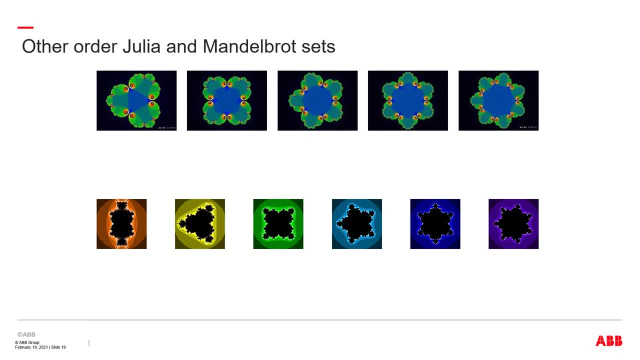 And then there is a share the slides, or is? the meeting is getting recorded, So I believe Ranjini will share it. Right, this will be posted in the Women Who Code YouTube channel. The recording will be available there. Okay, then let us look at other balance part. 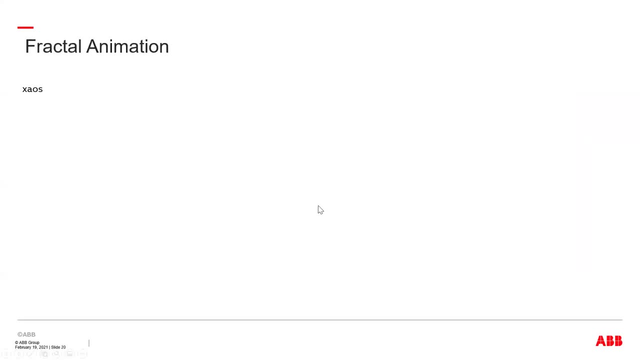 So this was a logical pause which I had put there, If at all. we want to do a break time, So let us do a fractal animation. This is just for a fun time that you can see. I use this. This is a program called Kiosk. 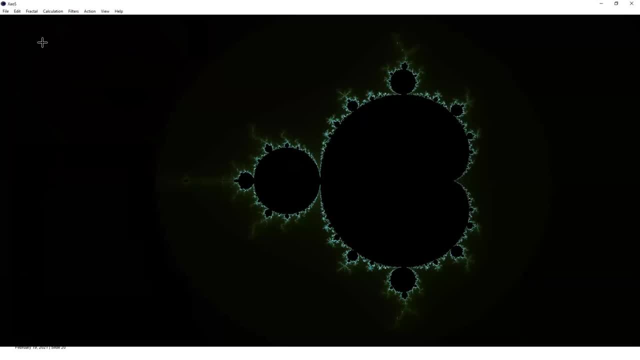 Okay, this is a program named Kiosk, So there are a lot of programs which you search around, you will get many of them. So this is a Zoom program which will get you to understand what like if you keep going inside again, and again, and again. 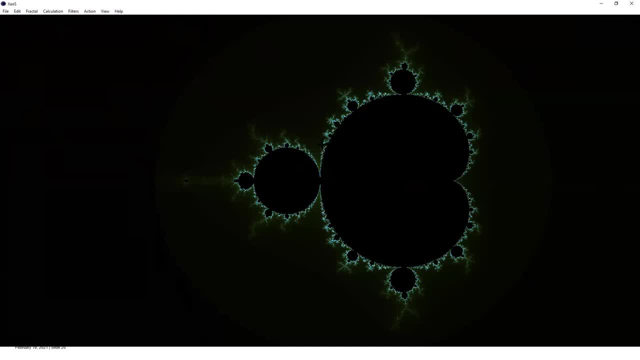 then you are repeating and the self-similarity, how it is coming. So if I just click inside, see if you can see a lot of patterns, are there? the whole picture looks the same. And if I go inside it's the same. 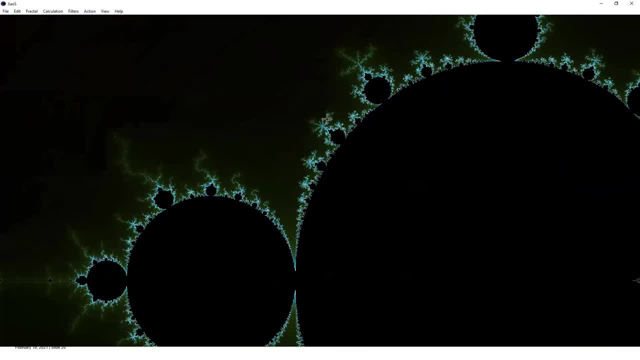 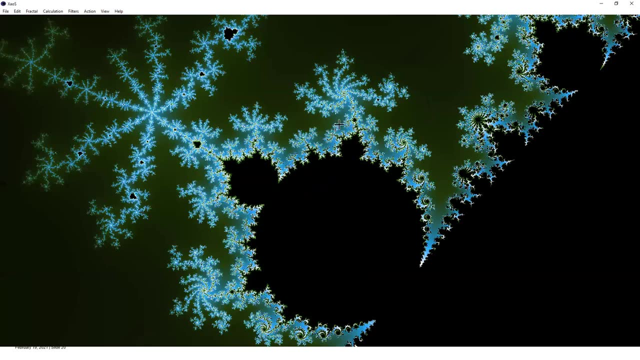 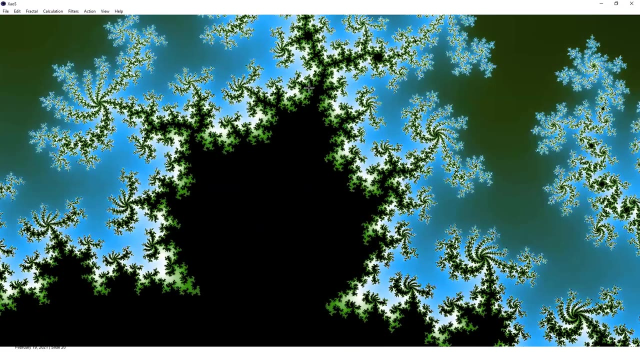 So if I go inside, inside and then explore certain places somewhere, ultimately you are getting into same patterns again. See what you started with. You are coming there again. Or maybe you look at these eyes of the picture somewhere. This is a very rudimentary program. 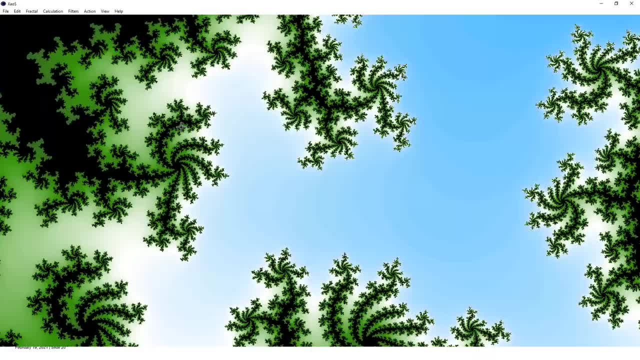 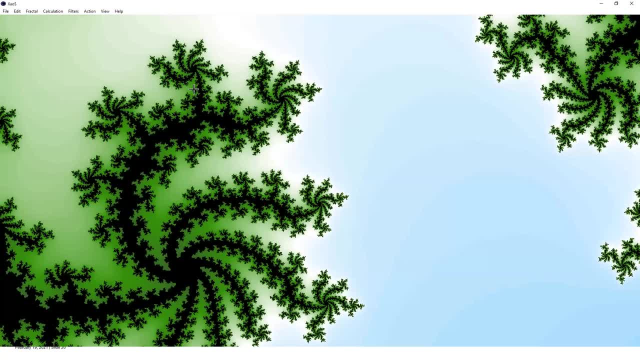 not very elaborate with respect to the graphics. This could hang and crash and all that is Kiosk program, but still, since it is a free program, I'm using it. See, you can see this, And there are very. the same pattern will continuously emerge. 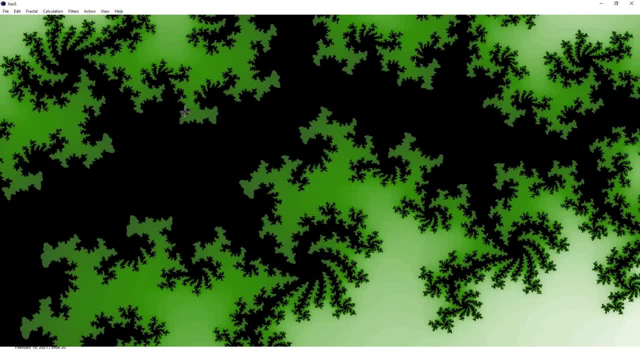 That's what we are seeing, So it will never end. You can keep going inside. Let me try some other pattern example. It's so stupid. I hope it'll be good, All right. So this is the interesting. There is a lot of in writing programs. 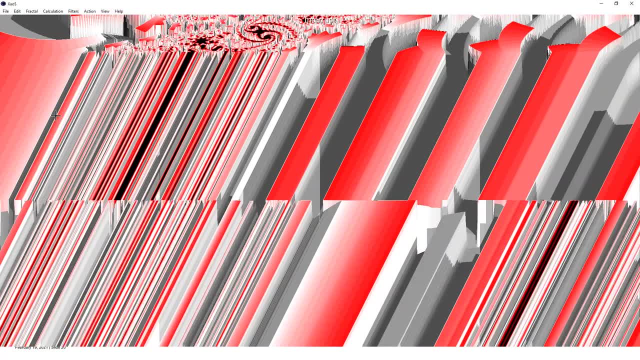 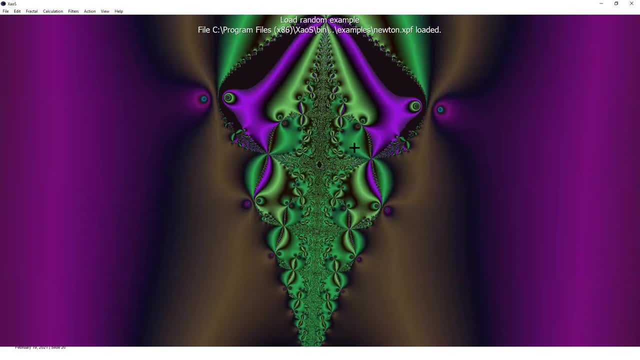 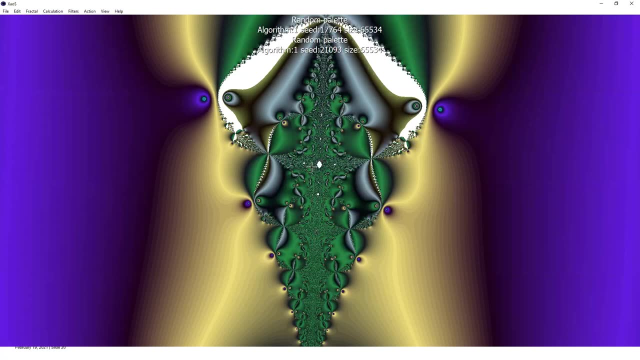 Okay, this is too much of a 3D. I'll get something which is simpler. Okay, these pictures you see. Okay, let's see this, This one also, if you go inside this. yeah, these individual patterns. 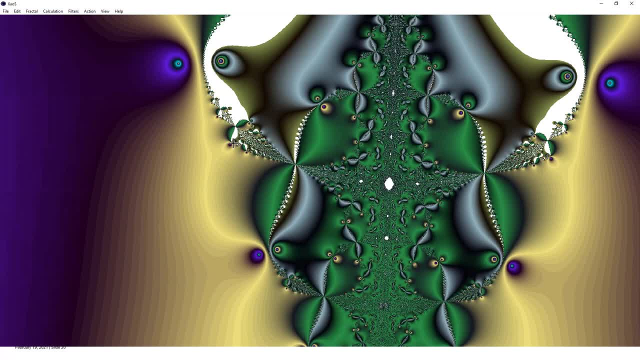 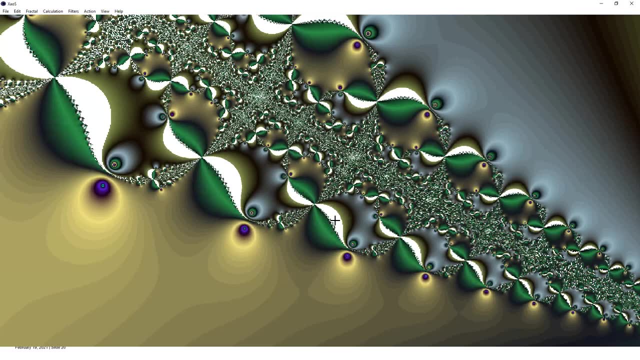 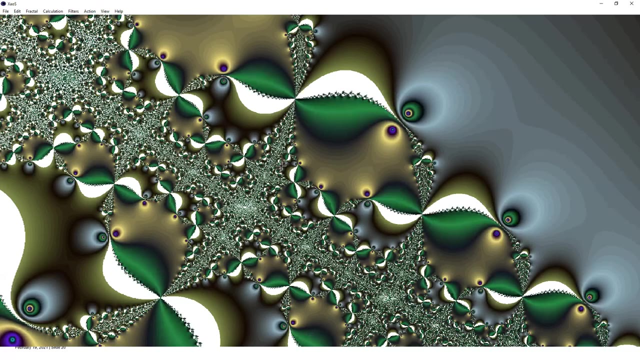 See this area, you will see it as the same structure, as a whole thing. So you can keep going inside And as you go inside you take it one area, one structure inside, you will keep seeing the same structure again. That is what we call ourselves similar patterns. 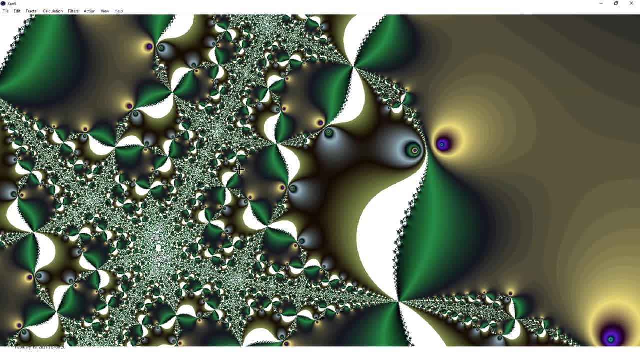 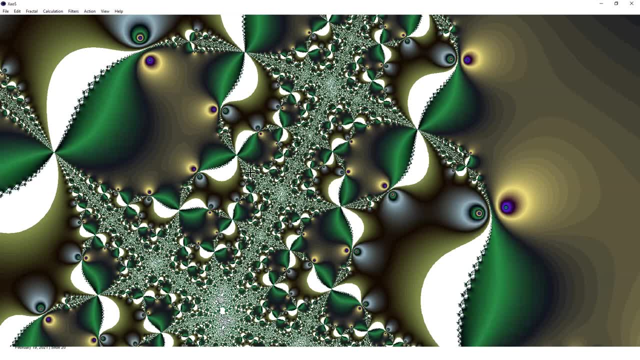 I have not written this program. Okay, But writing this program is not too much of a challenge, Like because it is the same same. I'm getting iterated again and again. So you walk inside again and again. you keep getting the same pattern again. 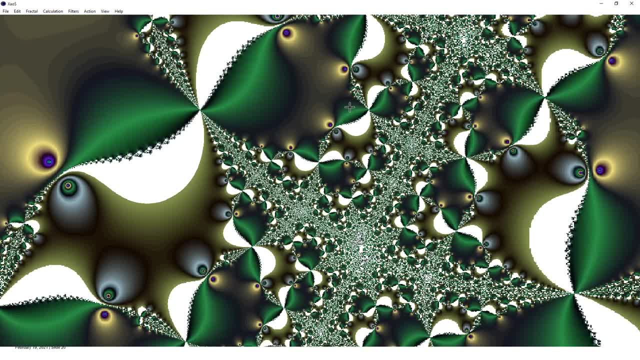 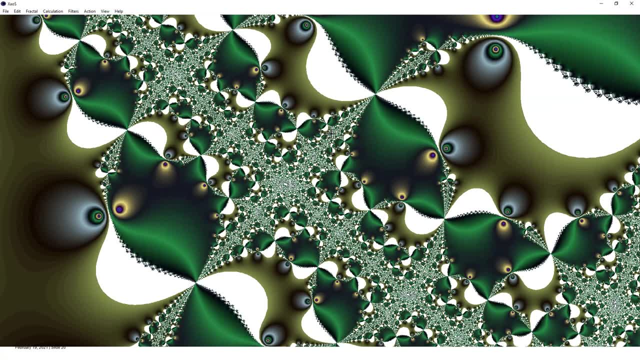 So this zoom is what make it really safe. You came here. Now you look at this pattern, You are again back at the same. So this is what that Indrajal picture that you were seeing. It looks like the same thing is reflected again and again. 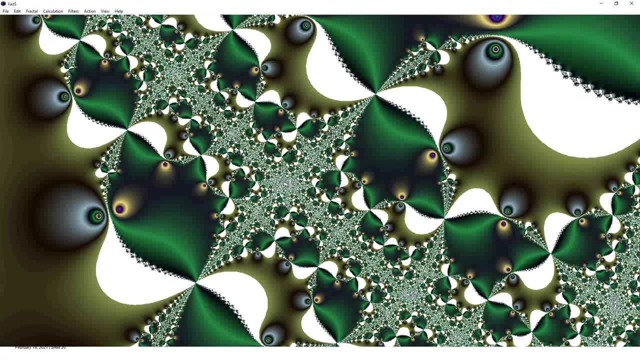 on an infinite reflection onto that pulse, that which they are talking about. So, in effect, what you will see is you do not know how far you have gone, Okay, Okay, How far you have gone into it, And even if you keep going, infinitely inside. 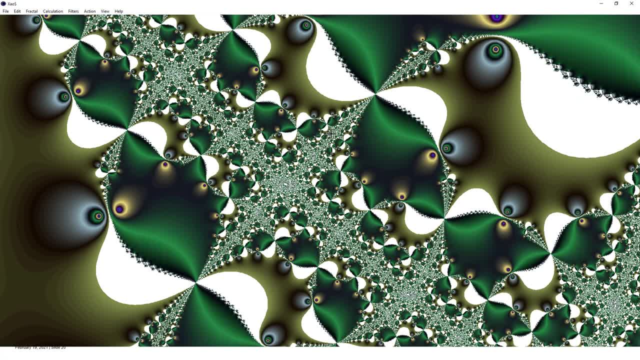 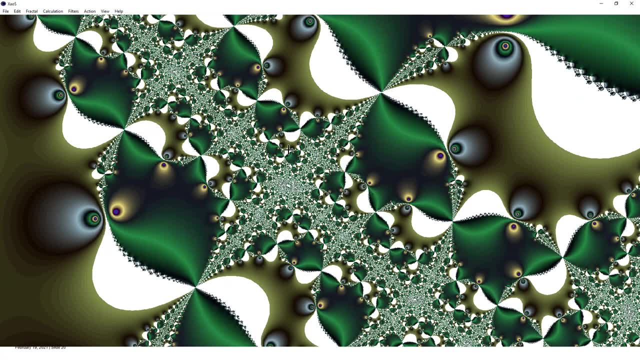 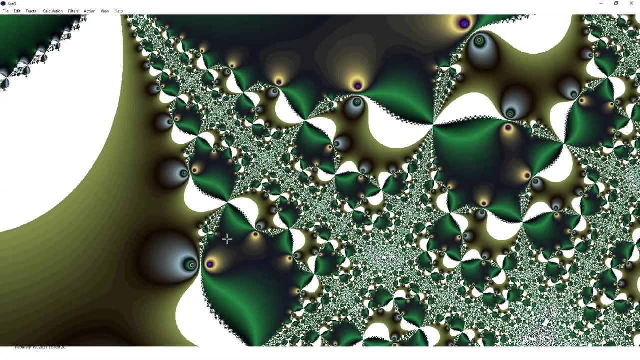 you will get into the same place and you do not know where you have reached. That is where that Maya Jal and Indrajal is coming in. See, I'm retracting and then coming back into where we went into. Okay, So these people have given some sample programs. 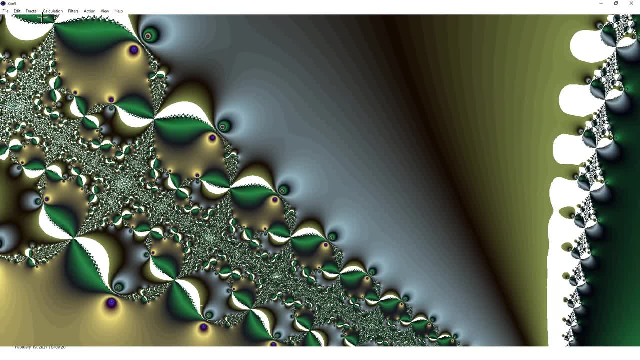 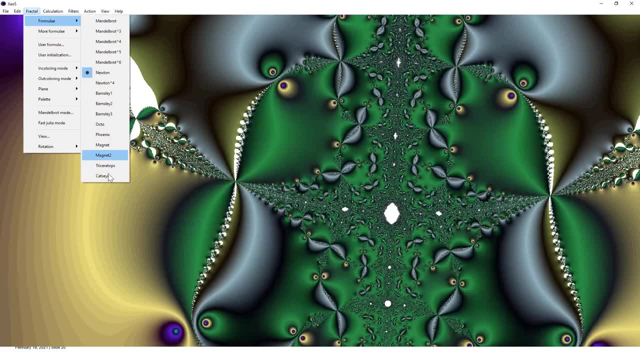 You don't have to depend on this sample program. You can also pick some equations of your own. This one also gives this calculation filters. You can put your own equations here, this formula and all that. right, They have some standard ones, but you could also create your own user formula. 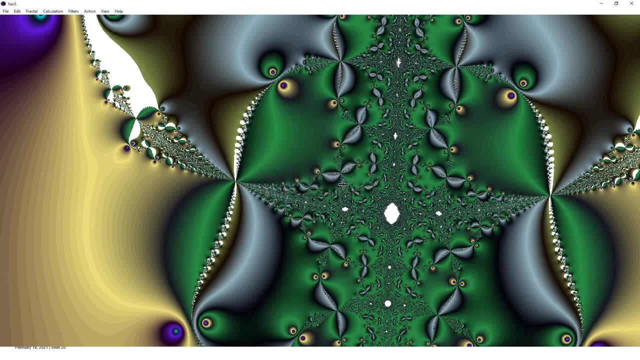 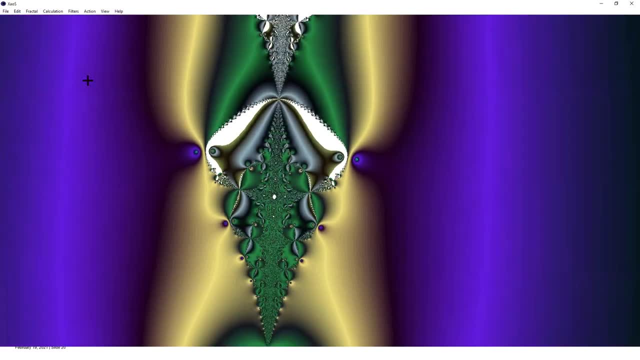 and then do what you want to do. You can put how you want to make it your own, But be careful. if you are not a little bit careful it could even get into infinity and then divide by zero and all that you can get into. 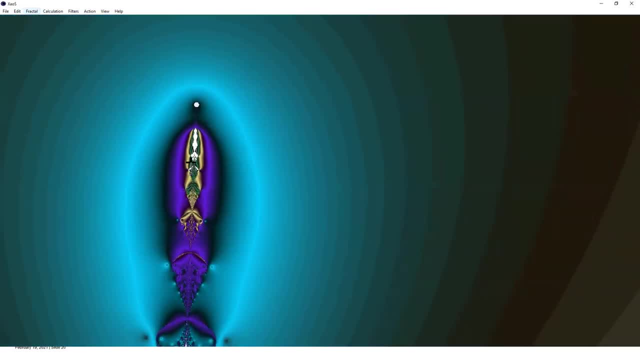 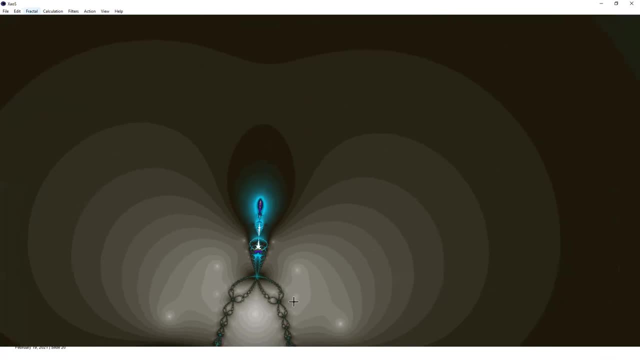 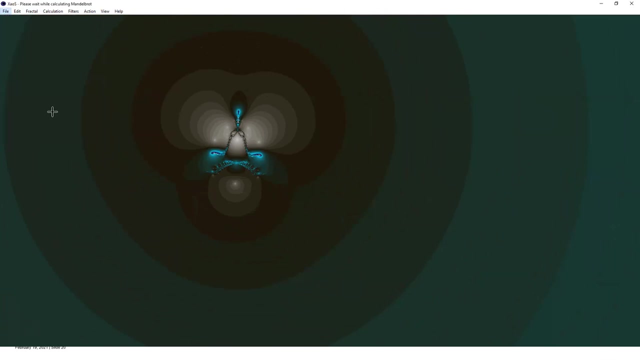 See, now I'm retracting back from where we were. Okay, Okay, Okay. Ultimately we'll come back into the same. We'll see some other example. This is just fun time to play around. This was again your same Mandelbrot. 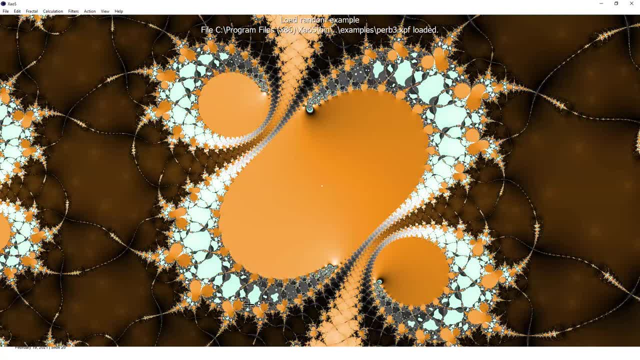 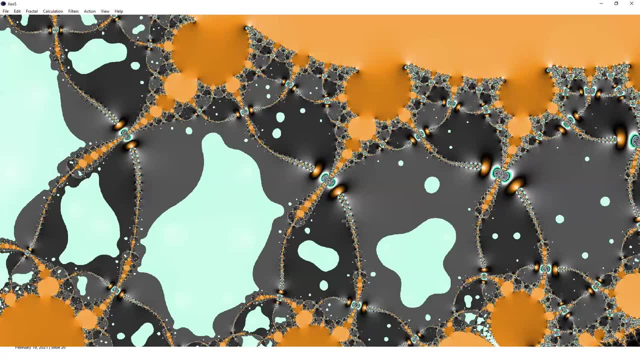 So this is another picture. If you go inside again, you will see the same, but it's the same pattern repeating. That's the whole concept of the whole fractal itself. These are beautiful, very colorful ones. No, I just tried different colors. 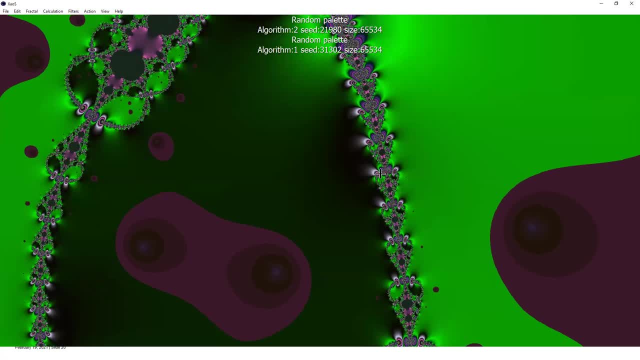 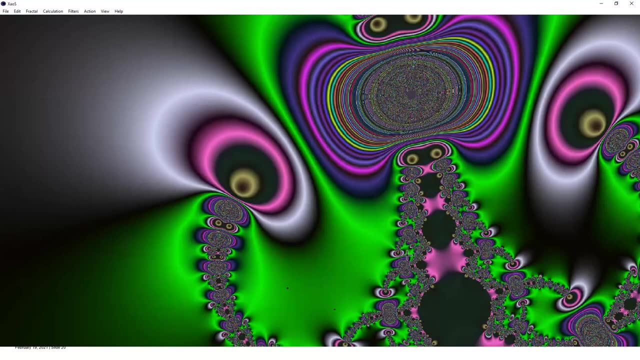 Green, dark green, I don't know what colors you like. Usually I like bright colors, so that it is easy and interesting to see. This is this is what I was telling about the concept of infinity and self-similarity. So if you walk in, you will see the same pattern. 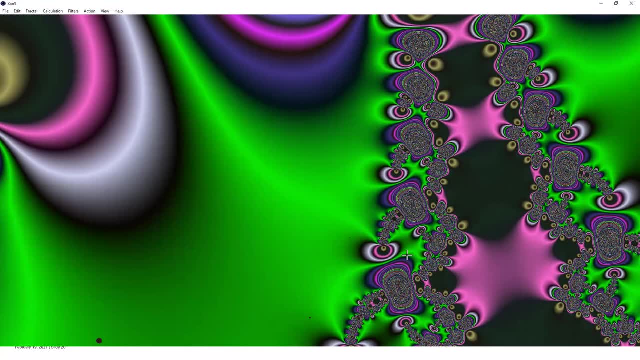 If you walk into one building or if you walk into that infinity, you keep walking. If you come back again, you are coming back, but there is no, not an end. I thought I will show you some samples. It's kind of a maze. 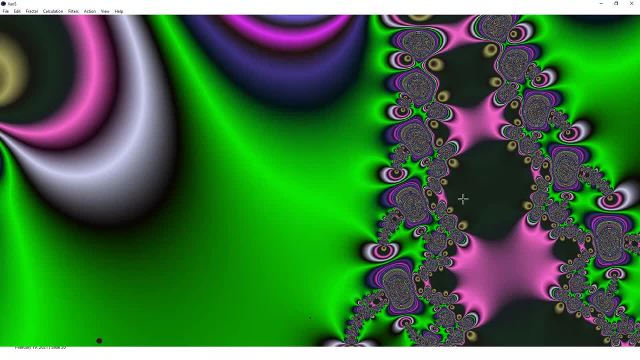 It's maze. Yeah, Maze is like maze. to buy is a maze means you can get lost, like we have to go through some specific paths. Yeah, This kind of a maze, Maybe you should pick it. The location is not known, We are going going, going somewhere, going going, and it is infinity. 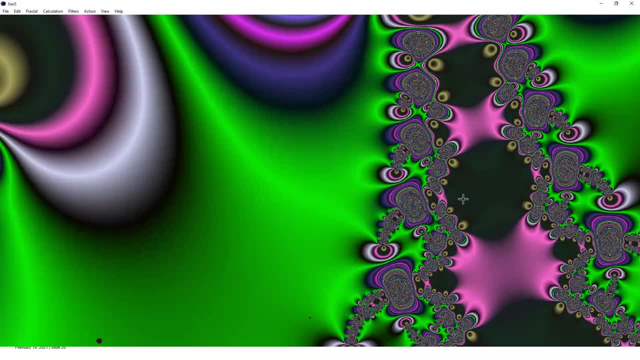 Yes, Because it is the same same thing that repeats after a while: Yeah, Yeah, Yeah. So how many steps you have walked? You do not know. Yeah, Yeah, Correct, You don't know where you are. basically, You don't know where you are. 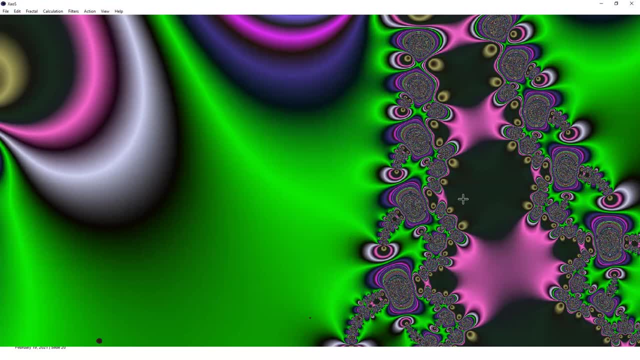 Yeah, That's why I thought it is kind of a maze but it's a beautiful structure. This is coming. But you saw that equation right. It is just take a complex number, square it and add a square, Yeah, And add one constant to it. 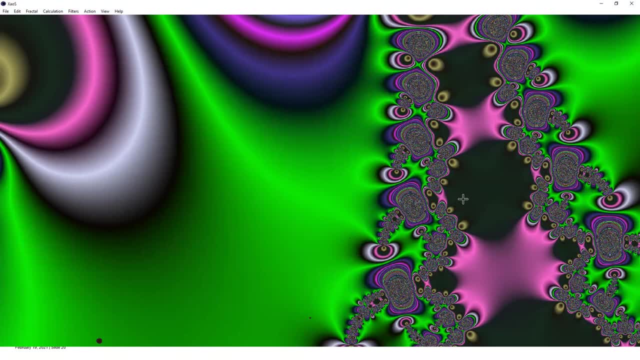 Yes, That is all that is there. Yeah, Yeah, It's quite a complex number, And add one constant to it. I didn't imagine that this small equation can do this much wonder. Yeah, That's what the. I also got fascinated into all this. 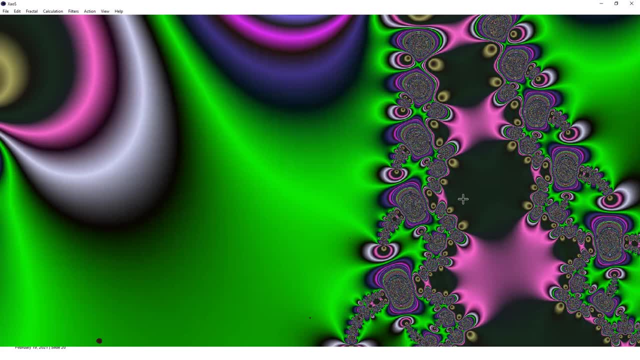 Like we are, like we have studied all our engineering mathematics, and we have studied all of them. So many mathematics, equations, And the equation doesn't fit in our book page and it will still go, Whereas here it is. You don't have to write it. 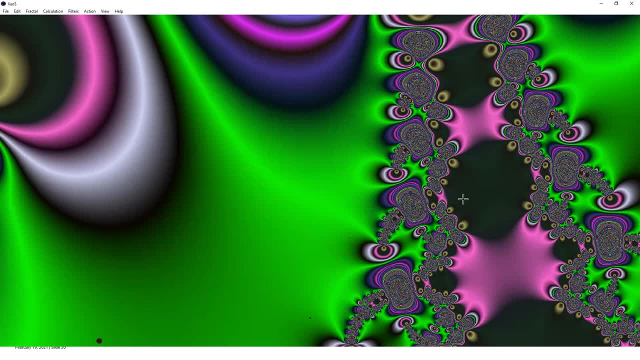 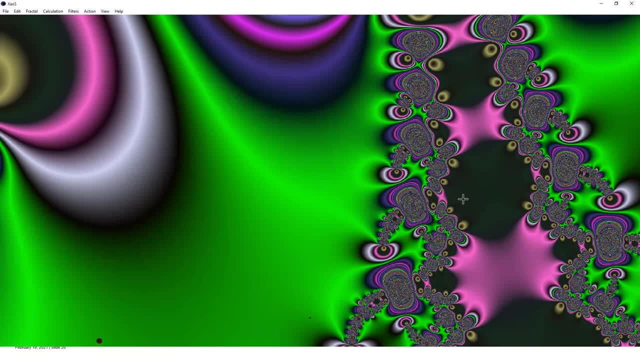 fit under very short, short light, but then you get lots of beautiful, infinite patterns out of it. Yes, Yes, It's very nice. It's very nice. Some of you who are part of my WhatsApp groups that don't have seen some pictures and patterns. 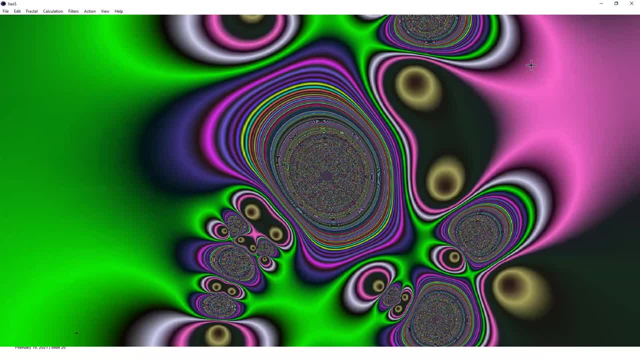 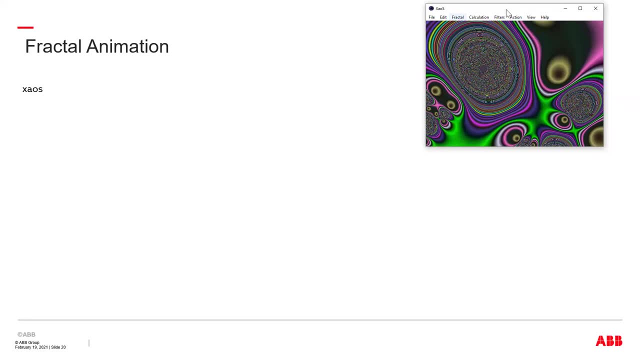 These are coming from all these earlier. Okay, So let us stop this playing around with the chaos program. If you're interested, You can take a look at the install this project. Yeah, then you can have a feel. they have enough of samples, or you can write your own. see, this is. 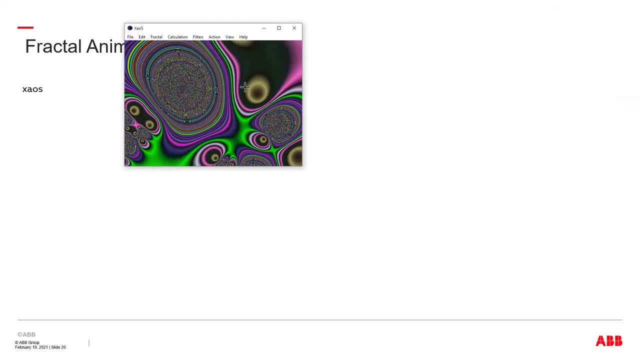 what i was telling when some of you were asking: do i write the program? usually in my early days when i was interested into all this, i used to write programs. but then over a time the charm of more than writing program it got into like playing around with that equation. so these days 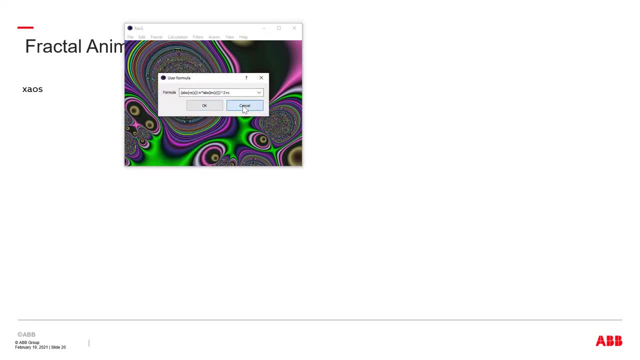 what i do is i take this, then i try to adjust formulas based on what i want to do and then visualize more, because that is faster. only so much time i can spend. see, i also have my full-time days work, so that is one reason that i write only small programs. 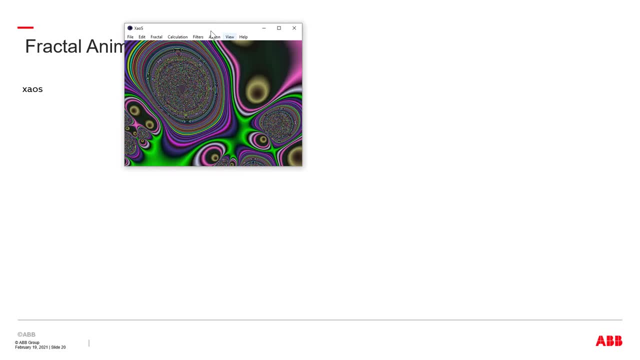 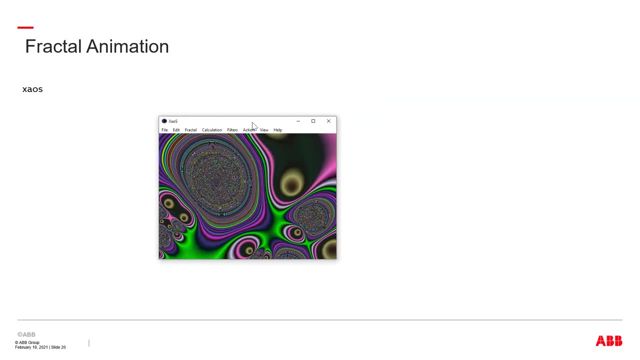 not huge programs? uh, one doubt. so in case of image, image is um array of numbers, pixel values. so each pixel value should i convert into complex number or no? no, no, no, no see, you get, there is a. i'll show you an algorithm later. see, whatever i showed there, the coloring. you get that x and y right in a complex number. 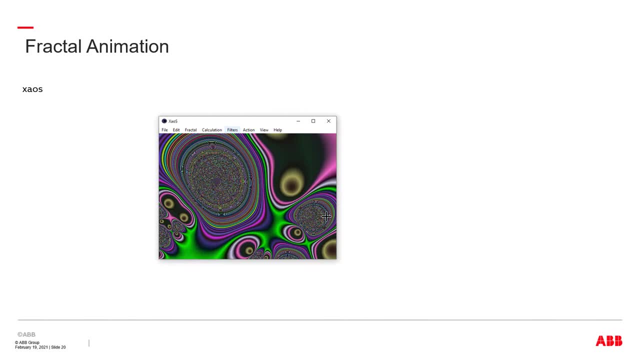 you. you have an a and b right that represent a point in a complex plane. if you take a complex plane you have, you can represent the real part under the imaginary part as a point in a complex plane, right? okay, so you can take that point. that is a way it is. there is a coloring algorithm very 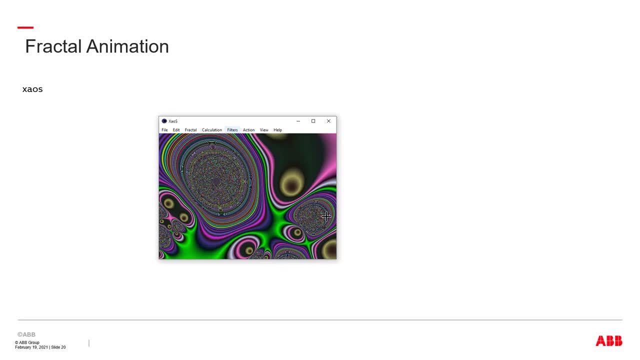 specifically. in fact, these numbers, they are called prisoners and escapees. that is a way these numbers are called. the escapee numbers are the ones which will keep increasing. they become fat and fat and they go off to infinity. like previously, i showed that squaring and adding. 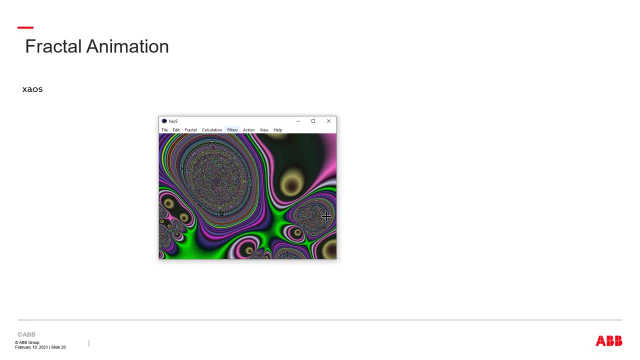 that equation part. so the those numbers are the ones which we call as escapees. they escape to infinity too quick. and the prisoner numbers are the ones which we call as the number. they stay confined, they never reach to zero and they don't go and then go outside at the same time they are. 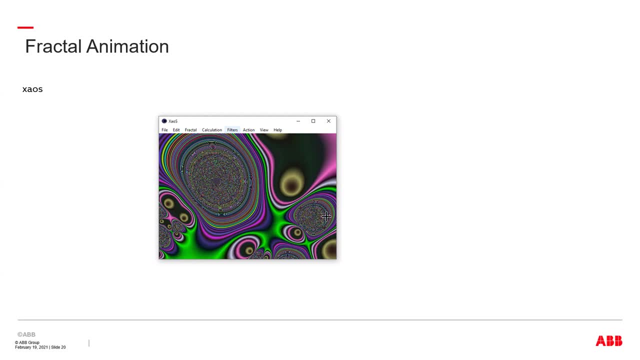 confined, they don't reach zero and they don't escape to infinity. those numbers are the ones which you are known as prisoner numbers like i didn't want to get into that level of detail right now. that's why i stopped. those are called escapees and prisoners. so, based on the coloring algorithm, 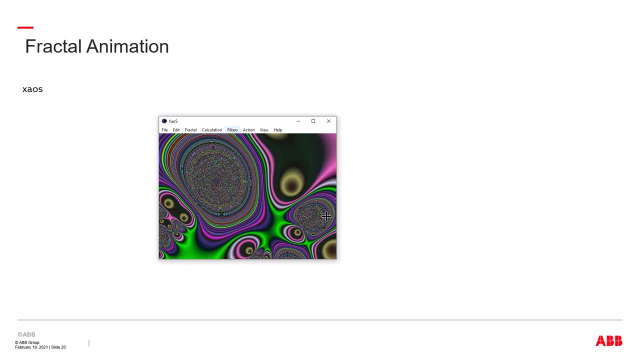 there are multiple coloring algorithms, the one simplest of coloring algorithms. what you could use use is you take a set of colors as your color palette and then you can color it based on. usually, what is done is: what is the tendency of that number to escape into infinity, or what is its? 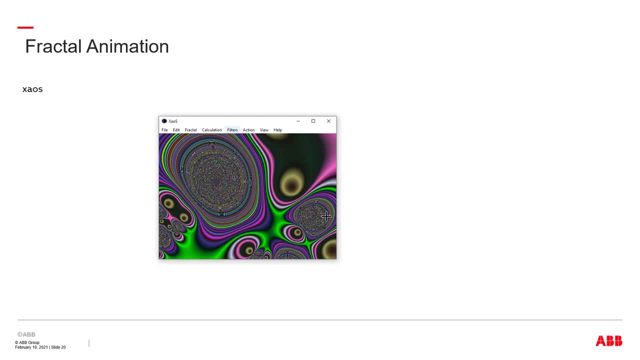 pace of escape. so if it escapes fast, at that pace, you start changing your colors from your coloring palette. so that is a coloring algorithm that you can use for coloring these pictures. you pick from a palette and then do it. okay, thank you. is there any online tool i can we see this escape into prisoner? 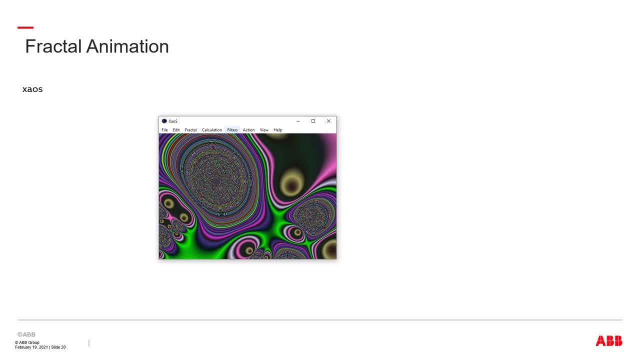 uh, see you, i think you will have to read, see, like what i showed, the complex number, right, if the number becomes like, if the real number, if the real part become, if you score, certain patterns of numbers will become escapees, certain patterns will stay. they get confined, like i showed you. 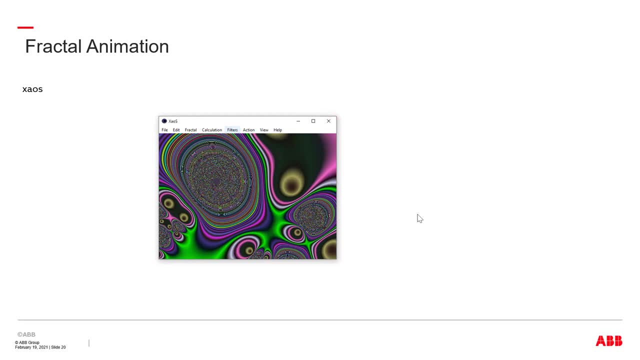 before right in our previous equation, some examples, some numbers. when you keep squaring and adding, they keep growing, growing. some of them oscillate between zero and minus one, whereas some of them you emerge into a pattern. they have a tendency to come closer to zero, but they never. 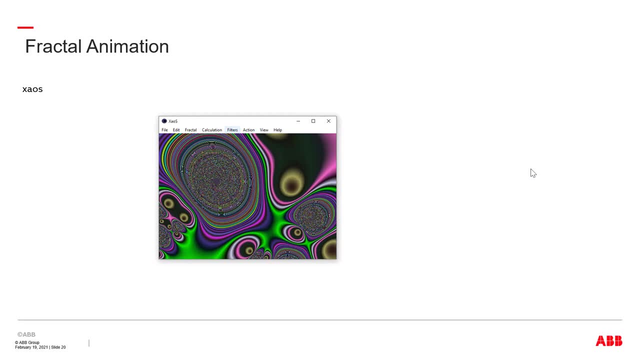 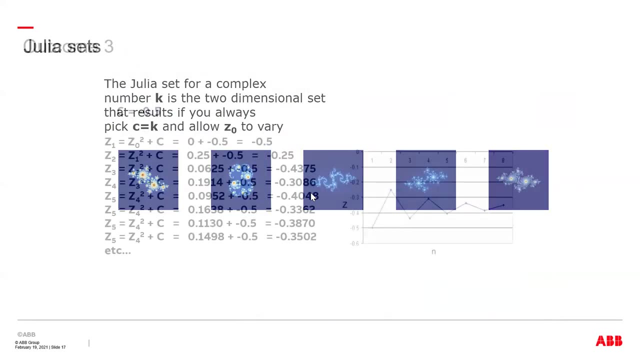 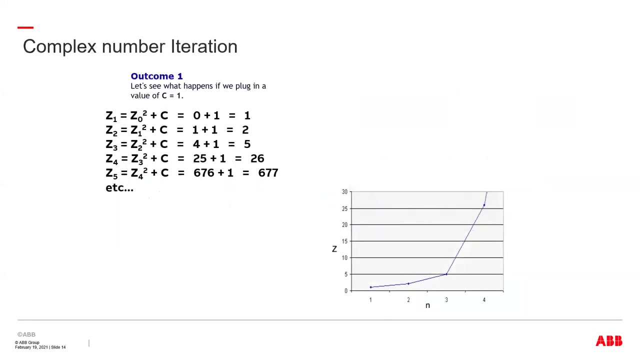 reach zero. just before i showed those squared numbers, squaring and adding. yes, i think i showed those numbers right. these ones, this will stay, these are on the periphery, these ones are the ones which are going too far, so they they escape. and this one, they stay confined but they don't reach. 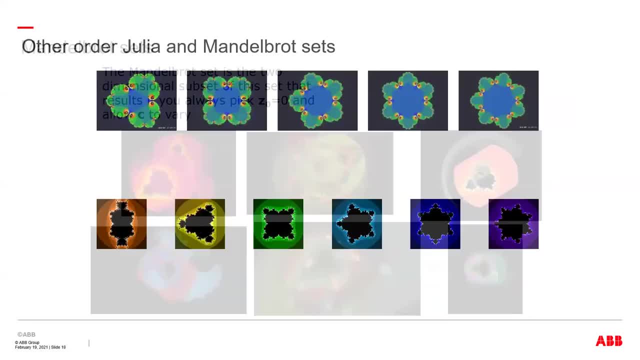 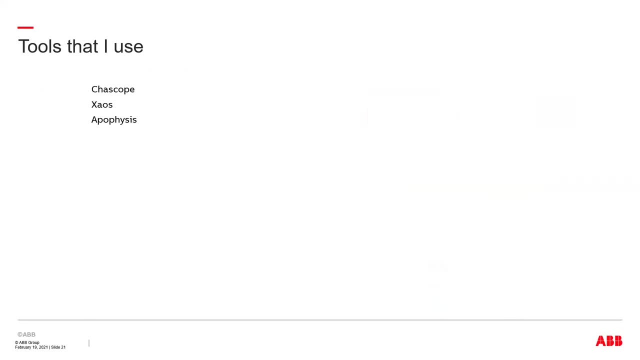 zero. that is where they call us prisoners. get this effect. uh, which numbers we should select? no, you can start from any, any complex number. you can start from anywhere. in fact, if you start from a complex number, you will actually reach there. i was showing those real numbers for an example to understand. 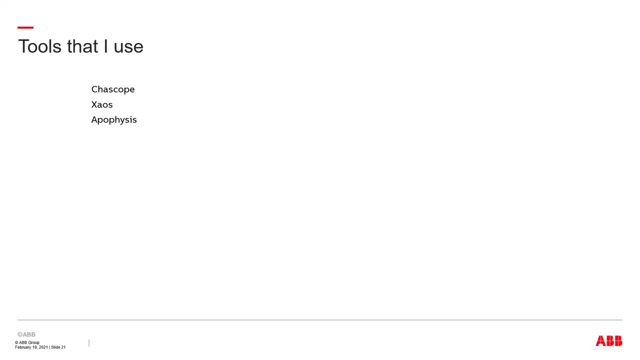 what are the properties of that complex number? that can happen and if you start from anywhere, you will get different effects. you will get different effects. so if you ask, where should i start, that's right in the starting point- will give you different patterns. that's what the whole concept of chaos- small change in input condition can give you. large 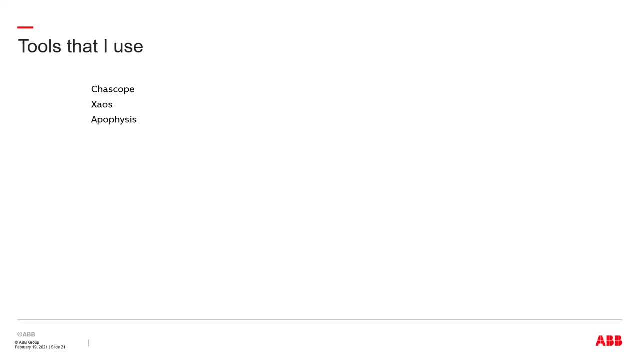 change in the outcome. the concept of chaos itself is there. so if you ask for where should i start, you start from anywhere. based on from where you start, you will get different effects. did i answer you? ah, yes, thank you. yes, thank you. This session is meant only as an introduction, to introduce the concept of all these. 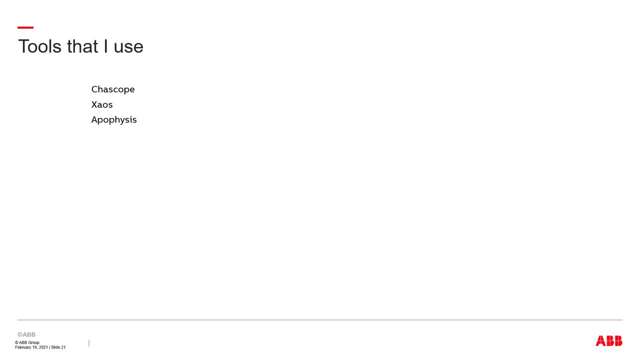 Okay, the tools. I use some more of tools than what is listed here. I use some other program called Mandelbulber and which are like these Mandelbrot sets. There are very specific tools. They are very slow in executing. That is why I didn't put it here, because unless your laptop is quite fast in executing, then you may find a problem. It will be very slow. 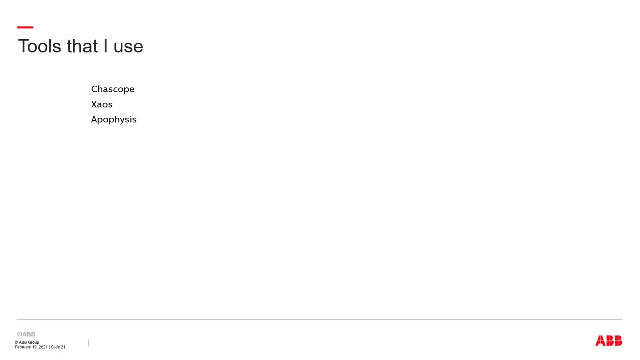 But these are some of the tools that I use. This Kioscope- Kioscope is talking about that, attractors, which I was talking about Then. Kios is a zoom in program that I showed. Apophysis is a fractal flame rendering program. 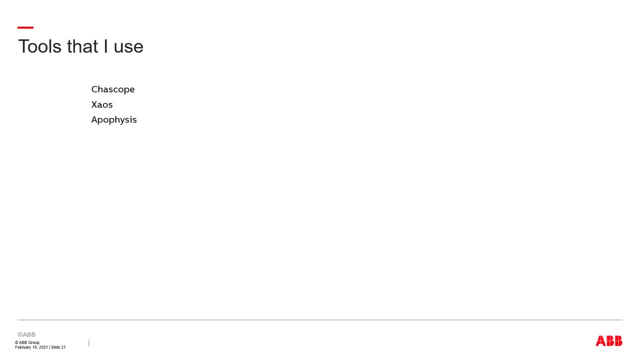 And there are also paid programs like Ultra Fractal, So you could search around for any kind of fractal rendering program. You will see many of them. You could choose what you find fascinating. Like I got stuck with Apophysics, That is something which I somehow generally found it interesting. 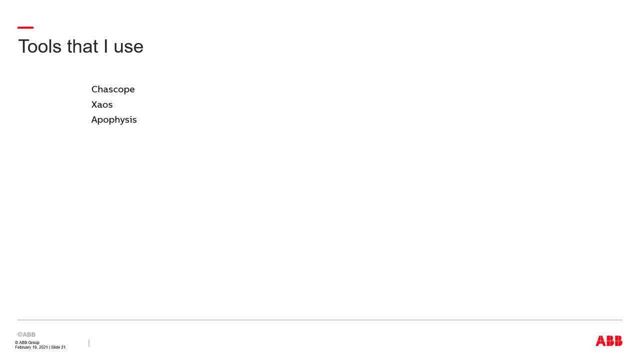 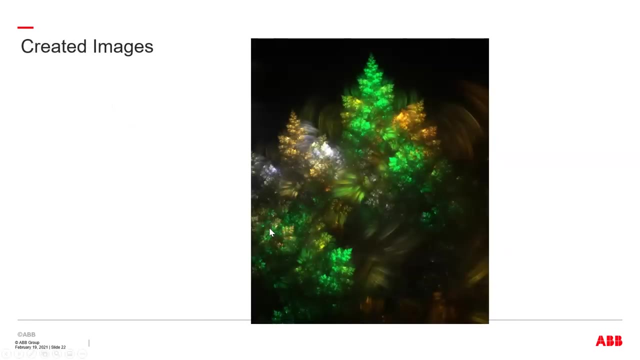 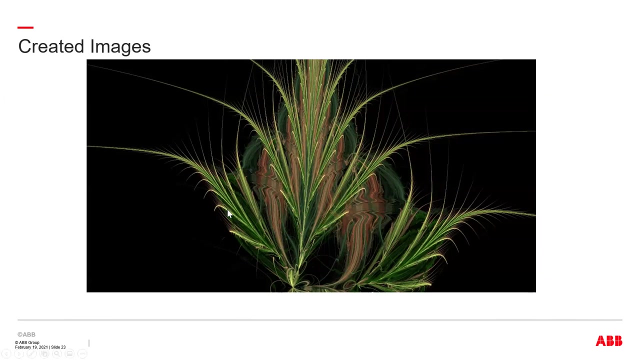 But I then it is personal taste- I'll show some pictures which I have created, So maybe we'll see some of them. I put some pictures here. See, this is one which image which I have created. I thought, okay, why not a show off some images which I've created along with this session? So these are some one picture which I had created, This is another. This all has the same pattern. If you see, the cell similarity is seen. 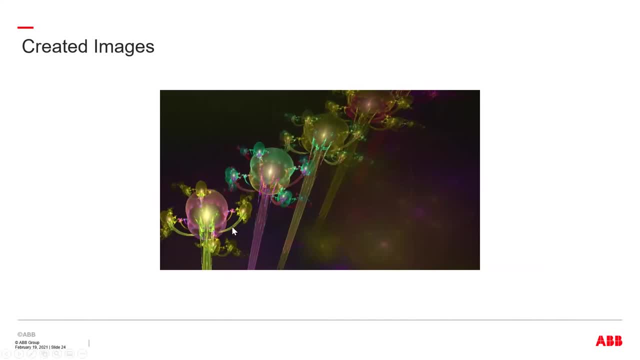 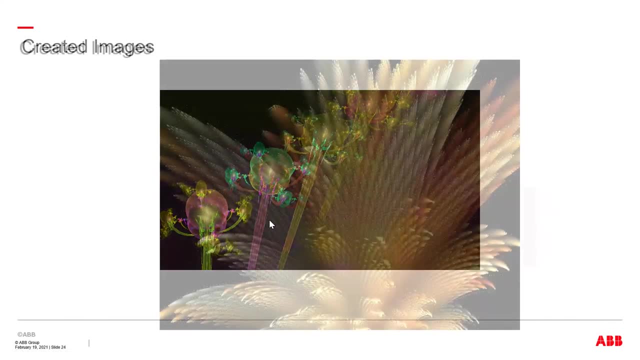 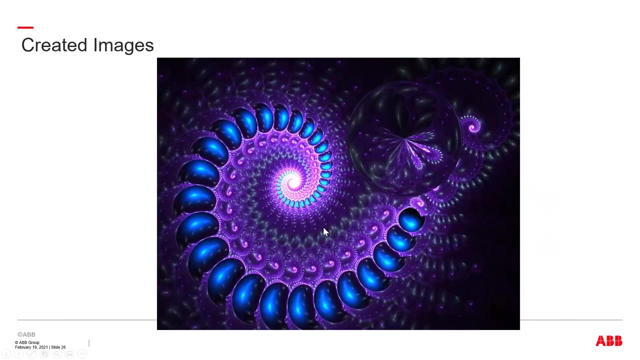 And then this is another one which is created Like, if you look at this one branch, the one branch again has the same structure. If you see carefully, that's what you will see. Time pass, creation. And this one: I still like the color combination of this, that blue and purple. 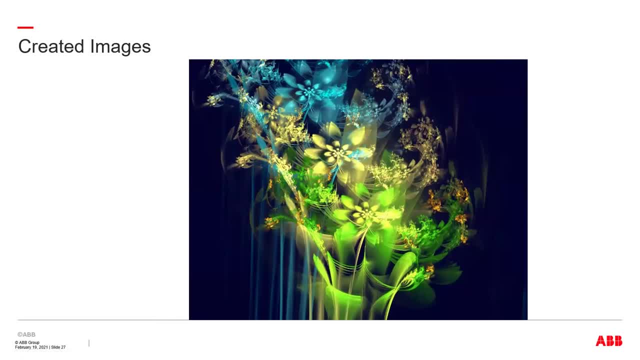 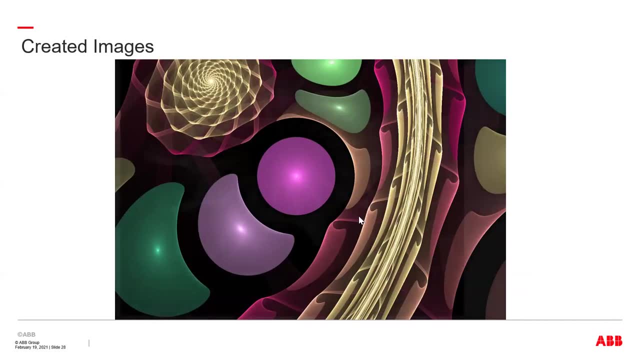 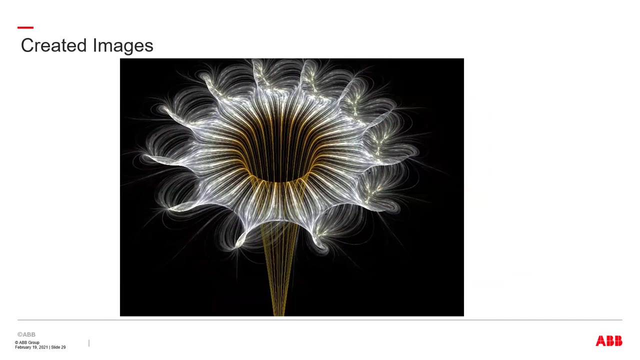 And this is something which okay here. bouquet of flowers And these are from samples from the apophysis. These are rendered here And this is another flower. I like this flower Somehow, Because I get that feel of that step and the flower. 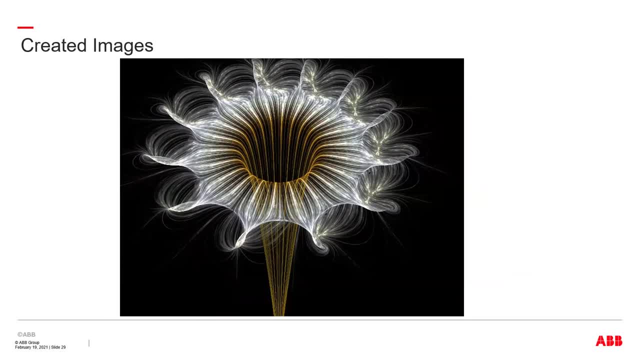 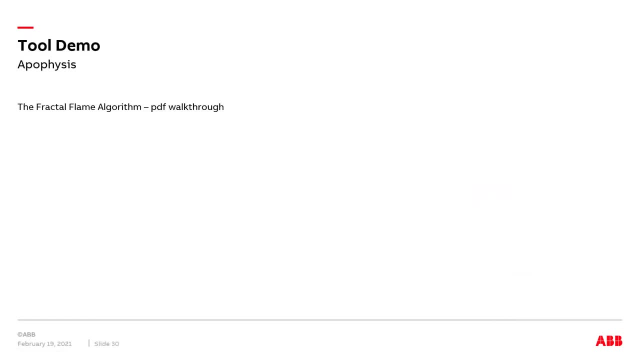 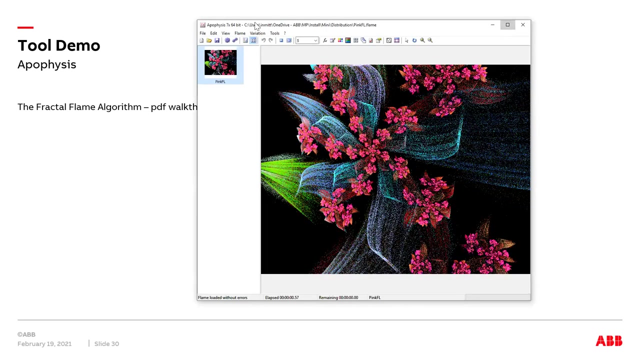 Like a bell flower, Yeah, so, whatever it be. So this is some other flower which I keep creating. And then there is tool. Maybe I should show you the tool which I'm talking about, Like what I did do as I opened and I kept some program which are ready, Okay, so this is a program which is called apophysis, which I keep using. So if you select the, what kind of a? 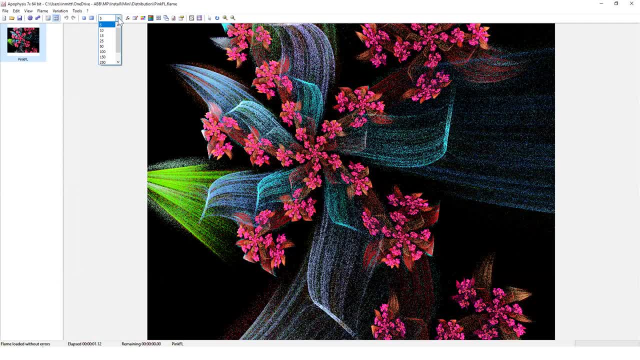 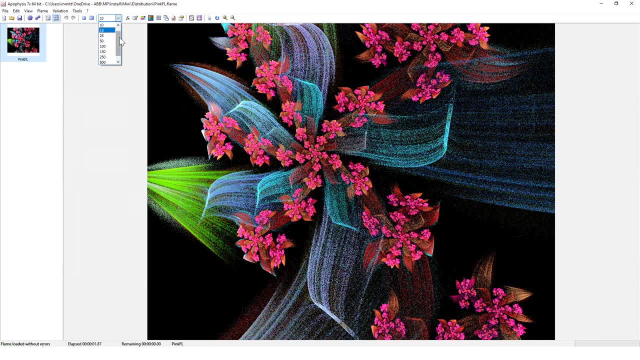 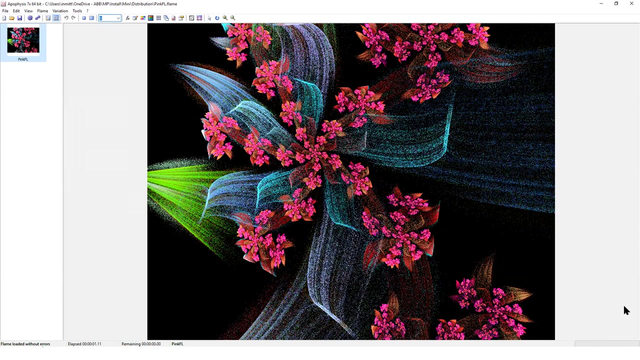 The density you want for Showing here. you can select the 500, because the more you go the picture becomes more and more clear, But then it will be slow. So, just for getting a preview, You put something small for your rendering, Otherwise it the rendering- takes time because it's a iteration. right, you keep doing it This. I just wanted to show some example. Okay, 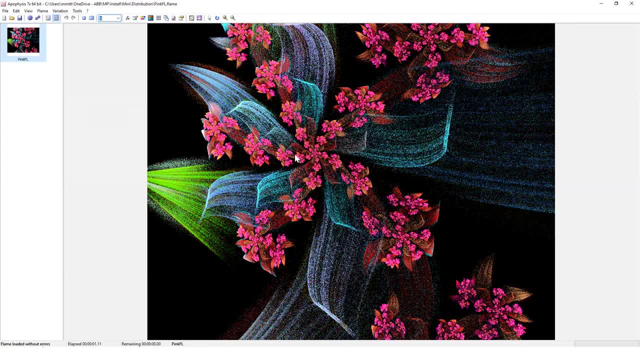 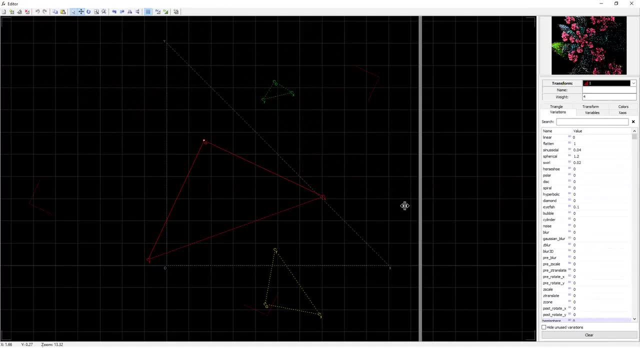 So what you could do is, in this fractal flame, rendering this a flame rendering program. So this F that it is showing that is the editor of the flame. So you can come here. These triangles are just representation. The triangle doesn't mean anything as such. Okay, 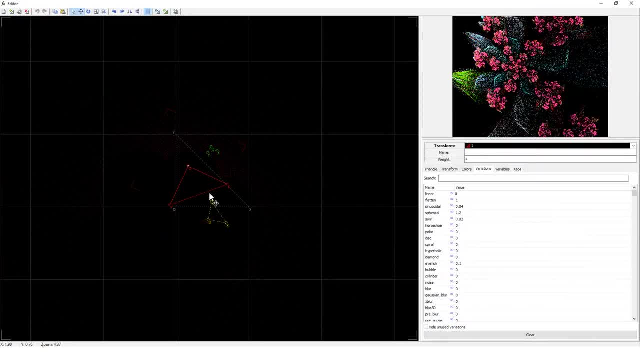 So they are. These are all various variations that you can use. you put some variation red one. You can put various weights to it. Over time you will get a feel of what these variations will give. these are Julia bubble for our goal. that I'll show. I'll tell you all this. These are all variations that you can put on to these. 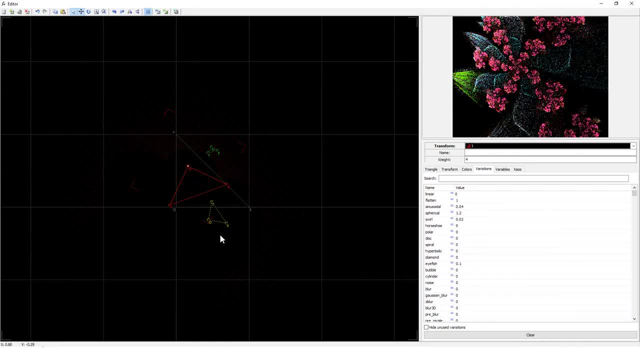 Your individual Flames, These. these are called flame but triangles. You can add multiples of flame and then add some properties to it. Then take this, another, some multiples of them You can create. it's not, it will take some patients. Okay, Don't think that the moment you start off with that You will get good results. 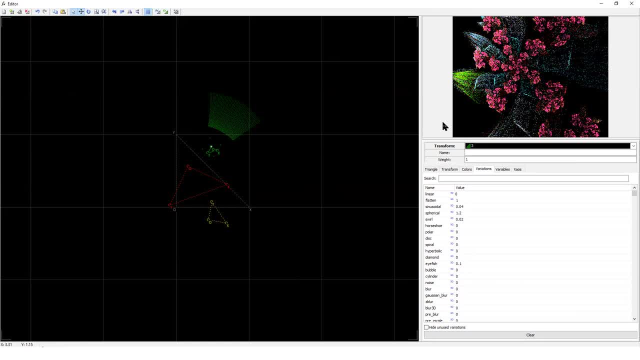 Beautiful flowers and all that. you will get some random, like you don't understand anything. you will just get some bundle of pixels which will not make any head or tail out of it. You just get to because it's all to do with chaos. So, over a period of time- but the highest has hidden patterns of this: beautiful flowers and gardens and all that. 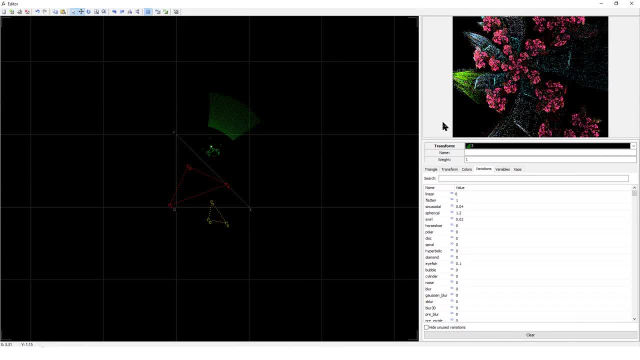 It will take some patients. If you are interested, that spend time. you keep playing around with it. at some point you will get it. It's not that Okay, let me start a flower. I sit down and I get it. Enjoy the process. at some point you will feel happy about something, then stop it. That's what I usually do, like. usually I don't have a target of this, what I want to make, or something. 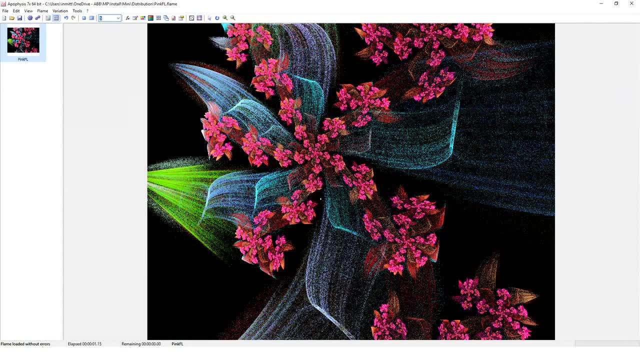 Like I keep playing around. when I find something attractive, I keep it there. Otherwise, okay, leave it and continue, discard it. and occasionally I also play around with random, so you can create a random batch. You make some random. you may find something from the randomness also. 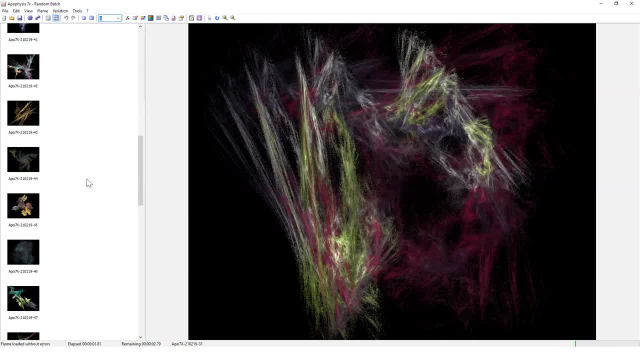 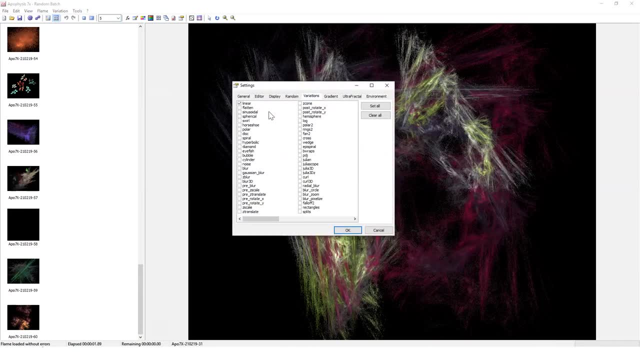 In fact, this whole thing is All about randomness. randomness is something which you will like it, And then you could come to these tools and the settings that you could import some variations from wherever you want. linear is a basic that you may want and Julian- Julian is all that the Julia said which I was talking about- These are all variations of that. 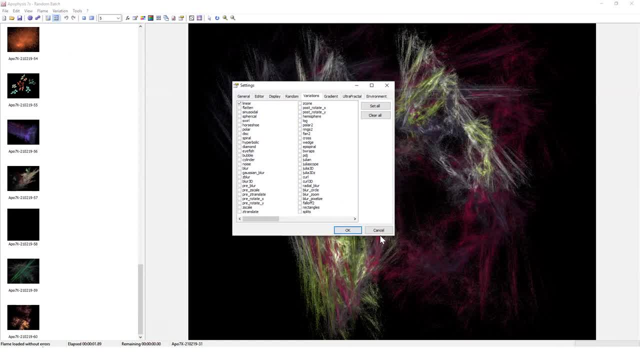 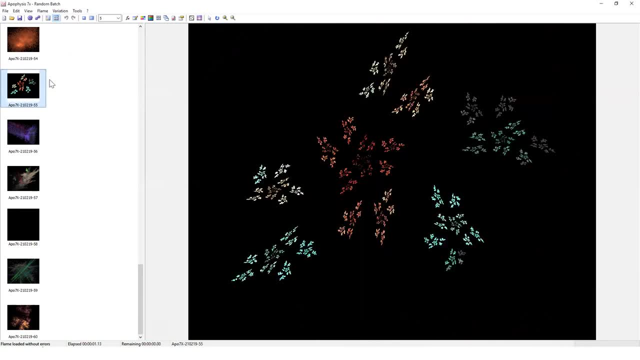 So pick these kinds of things. you can select some, pick some random, do whatever you want. some butterfly transformation you can do. But Play it takes some time and patience and like. it's not about like how, in the same way of looking at the chaos theory that we were talking about, 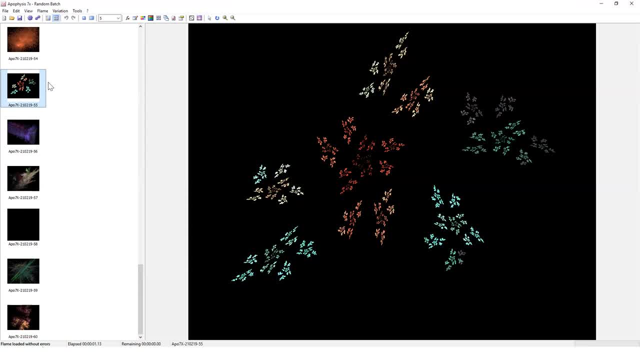 Like you can predict the outcome. that is a whole understanding of the complexity and chaos theory based on where you start. If your changes very small, your outcome could be totally different. So if you think that you have, this is the outcome I want, and then you want to reverse work, 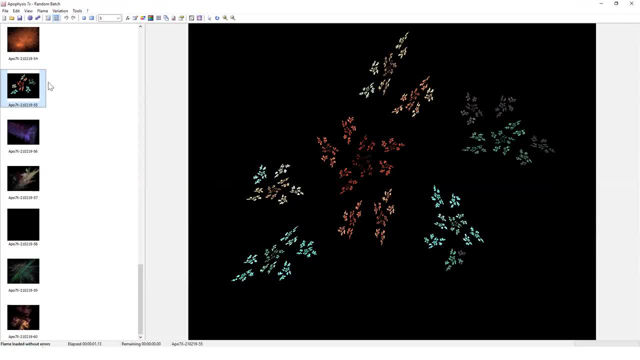 That may be more challenging than you start from where and then you go along with it. So you have to reach to some outcome, Because the whole concept of complexity and chaos theory itself is that, Like sometimes people say right, don't look for your results and will do your work, It is the same way. you keep doing. at some point you will get it. 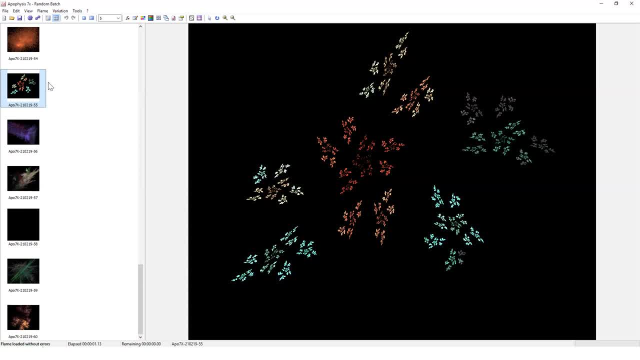 Beautiful there and over time you will get experience and you will know what to do. But then it is never that okay, like you keep a target in mind and then you keep working towards it, like that's not the ideal way to work on this. But then it is never that okay, like you keep a target in mind and then you keep working towards it, like that's not the ideal way to work on this. 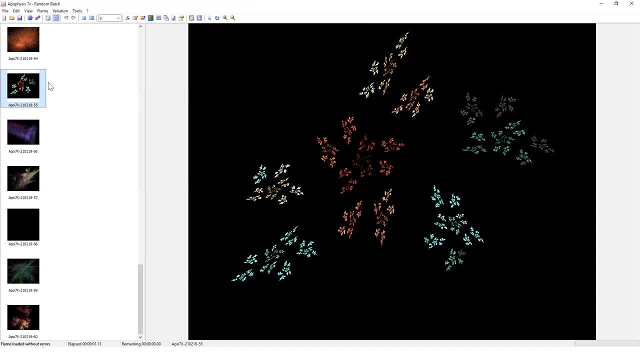 Anything else, Any questions? One group of patterns can be removed from the result. You can, But the thing is they are all interfering with each other, Like how I was telling. right, like the moment you remove one, you may not get what you have in mind. you may get something totally different. You can remove, see. 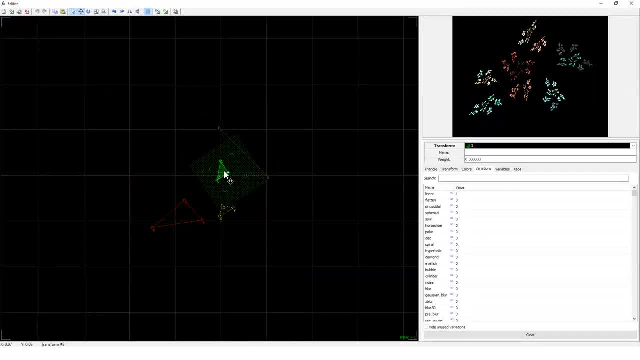 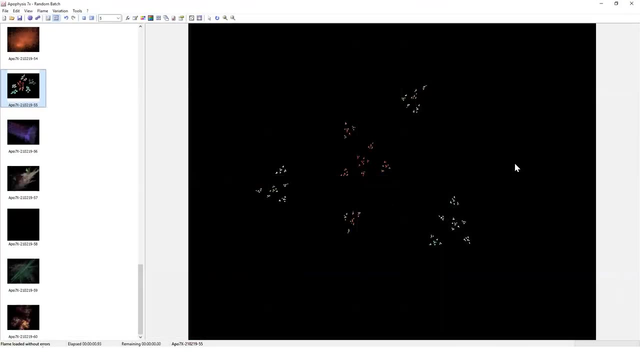 I like say: you take this, you come here, These are random, Okay, I just took random, So you take this, you remove them, You get something else. But then These are all linear, So you may get very similar to similar, but then The moment you remove something, It's not like one thing you remove, because they all interact with each other. That is what the whole concept of system and complexity itself- They interact with each other- to give you. 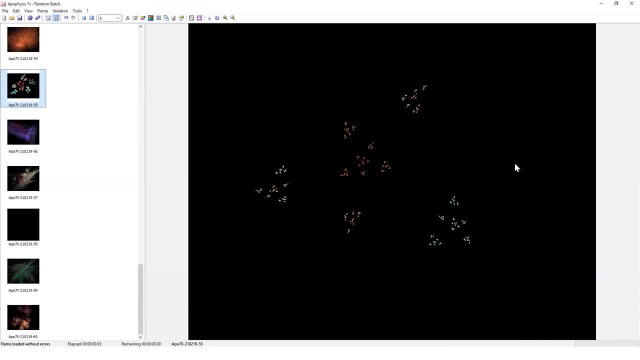 Not think of Even this complexity. iteration is also the same. Like when you remove one small effect, the same butterfly effect. Like if the butterfly had not flapped its wings, the hurricane would have occurred. like If you talk about A butterfly at a hurricane. you won't be able to see that relation so quickly. 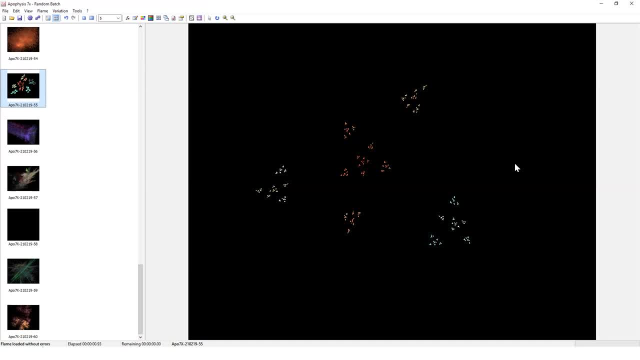 Yeah, Like they are too far relations right? butterfly and hurricane, Yes, yes, But now if you think in a complexity terms, then you can comprehend. Okay, that's more. butterfly flapping the wings would have created some arrow abrasions That would have got propagated. maybe that air vibration with other effects got amplified and then it would have caused your hurricane. 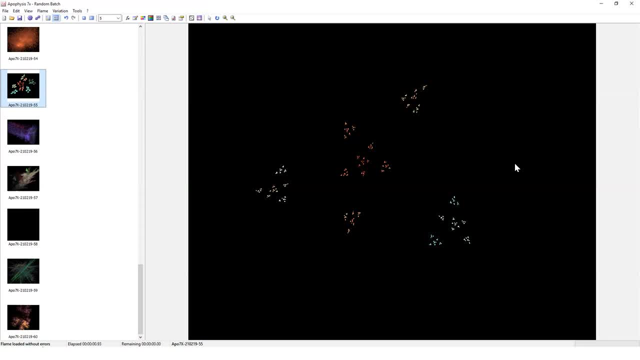 So it's not that one item that cost all your effects. Yeah, that's what Even in our life is also. very times It's like that: one small thing which we did. if we had not done it, probably that large output wouldn't have happened. 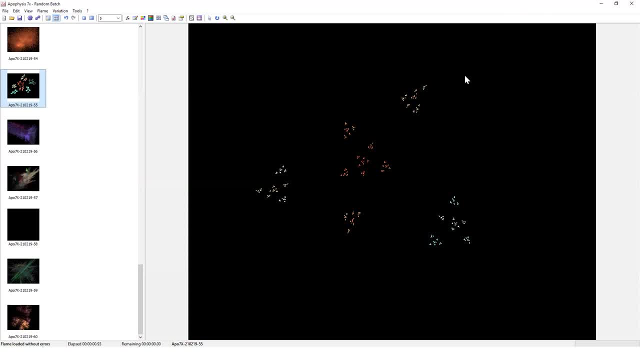 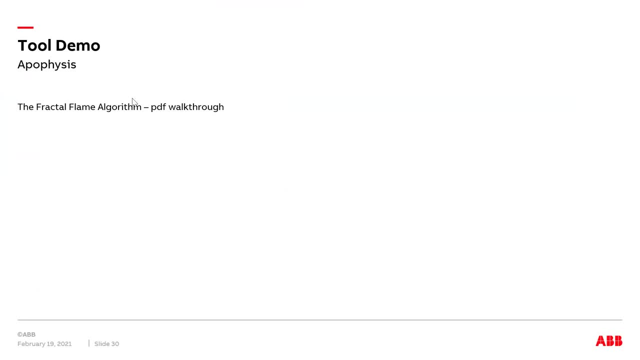 It takes you along. That's the way to easier to look at it. Okay, And now I think I want to show you that the story behind that is the flame algorithm paper. So there is a paper. This is what This flame like, how much. 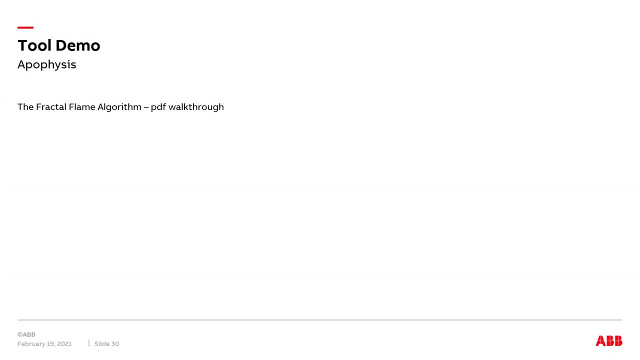 Yeah, And that is the question I posted. Could you please open that link and see? actually, I wonder how to know how to map the pictures, color into fractal color Now, fractal image. See, there is a coloring algorithm. That's what I showed you before. 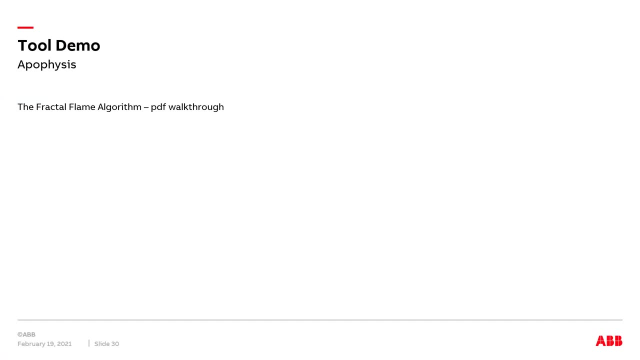 How, how, No, no. Mona Lisa picture. Rectal image. Okay, let's read. I probably I'm not Understanding what you're asking, but let us. That is a picture of Mona Lisa. I won't And this one: 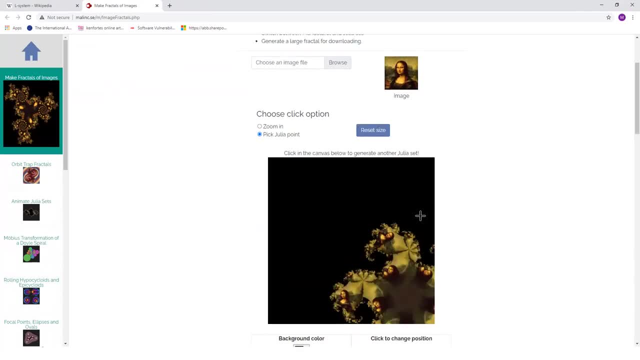 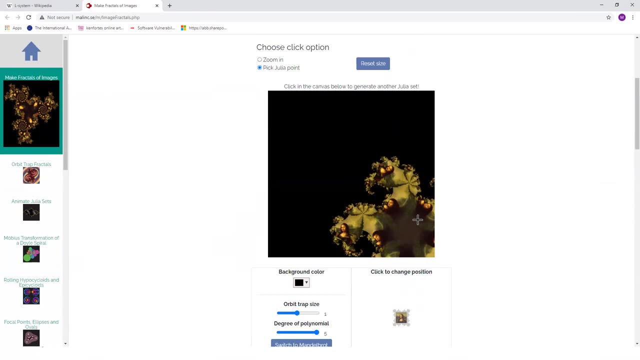 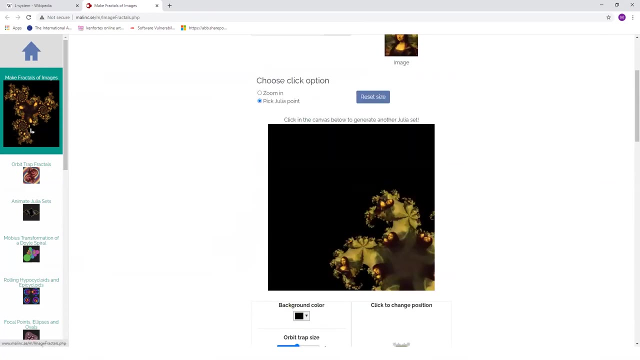 That is the above imager. she's wearing a brown gown, The same color. how it is coming here back? You told they are taking x and y coordinate, So See what you are seeing here. this- this may not be model brought, but this could be a variation of Julia. 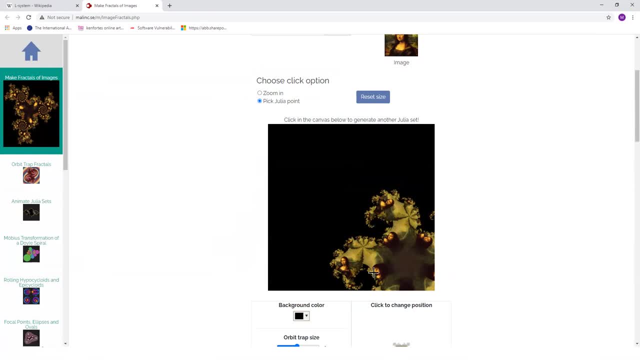 what I showed you. Okay, So this one is. what they are doing is, instead of looking at it as a point, like I had a picture there somewhere, the whole eyes, one of an animal's body full of eyes- I had a picture somewhere there around. See, what they are doing is- it is a mix of graphics, See. 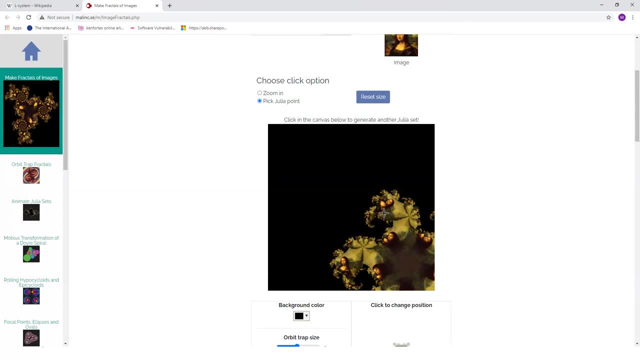 usually like I'm a purist. See, that is one reason which I did not get into this. There are a lot of people who do This. could also be with you: take one picture and you use that as a point and then doing it. I am more of a purist person, So all the time what I am doing is just raw fractals. 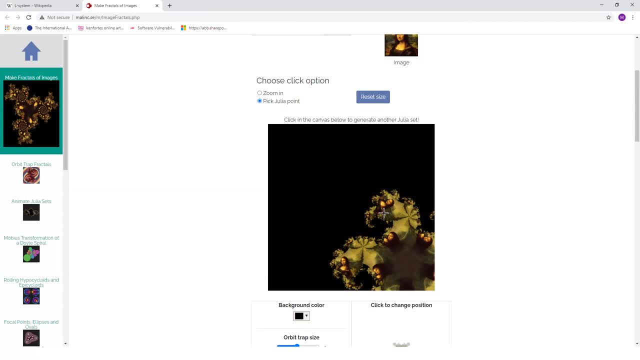 There are a lot of people who take fractal images and they blend it with other Photoshop kind of Photoshop, GIMP kind of things. But here from the picture, what it looks like is they have taken a fractal iteration and then, instead of drawing that one point there, they put the whole monolith. 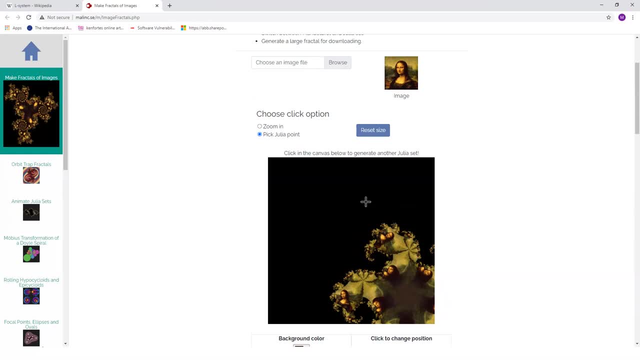 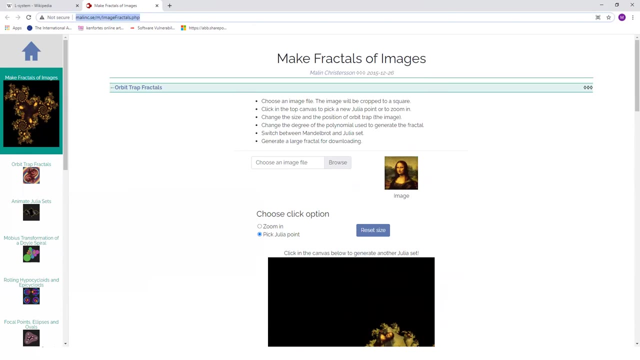 out there and must have scaled out. That's what it looks like. Okay, Now I got what you were trying to ask at the very beginning. I'll have a look at this program. Anyway, interesting, Yeah, but I think I'm too much of a purist person So maybe I didn't get into this. 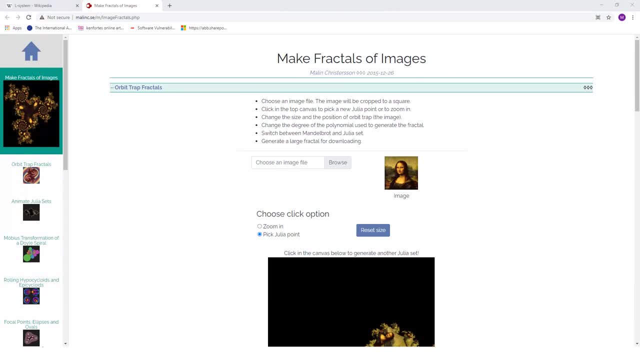 In fact, I was staying away from looking at mixing Photoshop and GIMP with these pure equations All the time, like I was staying with the pure equations. I think you can leave your contact somewhere in the window or somewhere, Or you. 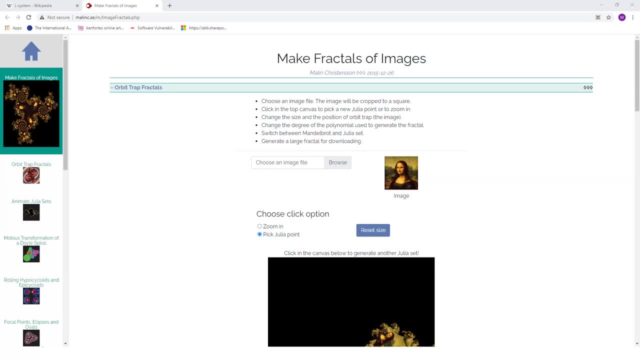 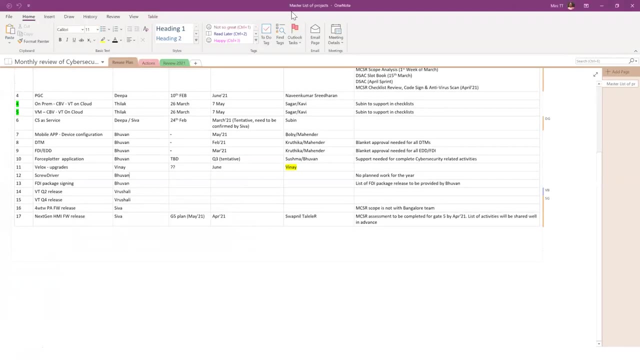 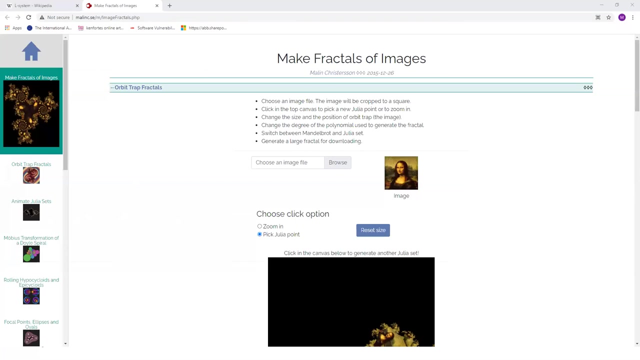 could pick my name from somewhere there and then we'll have a look later after these sessions. Sure, Thank you, And give me one minute to let me keep an order of into my system for your reference link. That's my one note. I'm just taking a time for putting my reference now. 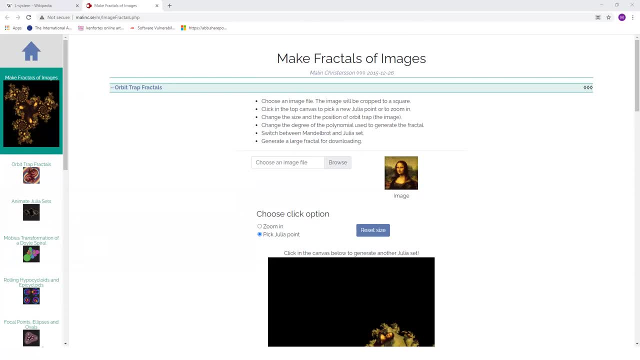 Yeah, but probably it is time that I also change a little bit out of my purist mode, Like somehow I feel that I should not be doing that, But mixing two things like this picture as well as this. I have seen a variety of people who do what they do. is they take some kind of picture? 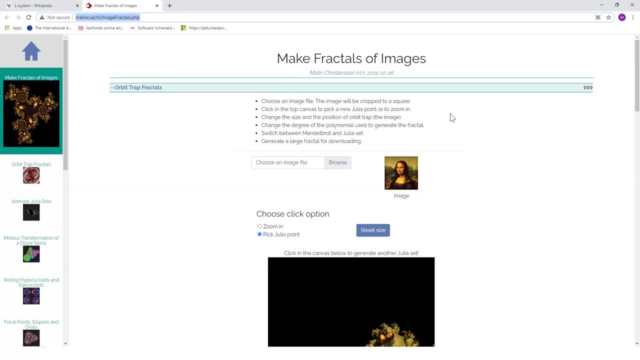 This is one way. do the other way, like take a picture and put the fractal pattern onto the picture, This one does: take a picture and put the picture onto the fractal. Let me come back to our place. Okay, this, this is it. 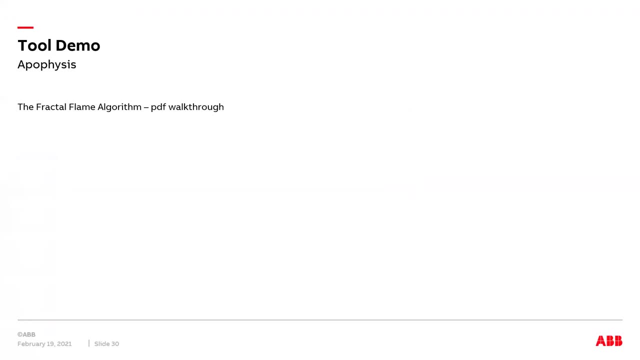 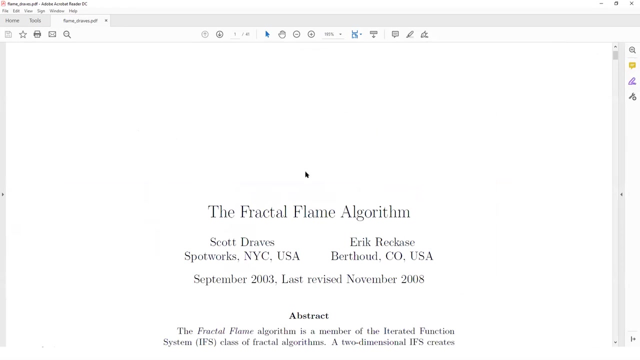 is the algorithm which I was talking about, The fractal flame algorithm. This one, I'm only introducing you to it. I'm not explaining the algorithm, but I would suggest that you read it at some time for your leisure. This is the one who also runs a website called. 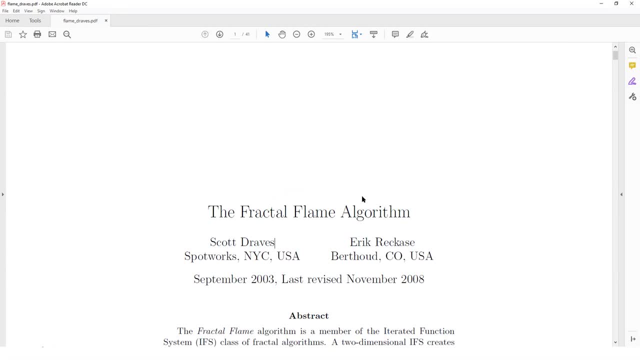 Electric Sheep, So you could look at that website of Electric Sheep. But then the base is coming from this flame algorithm Like apophysis and ultra fractal and all that are flame algorithms. So what they do is they call these variations or transformations, and 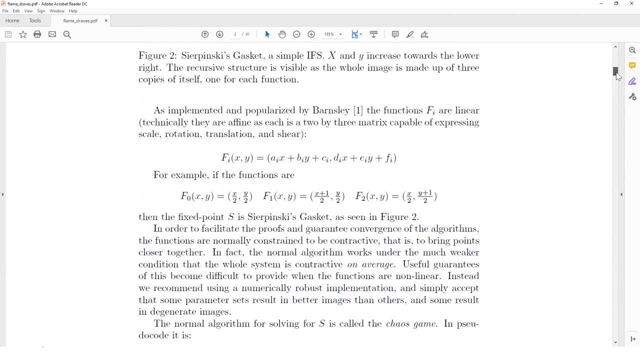 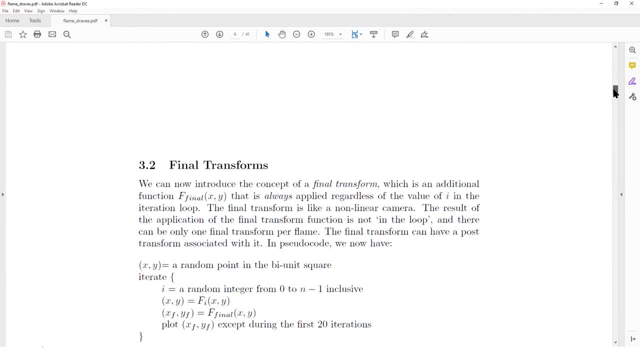 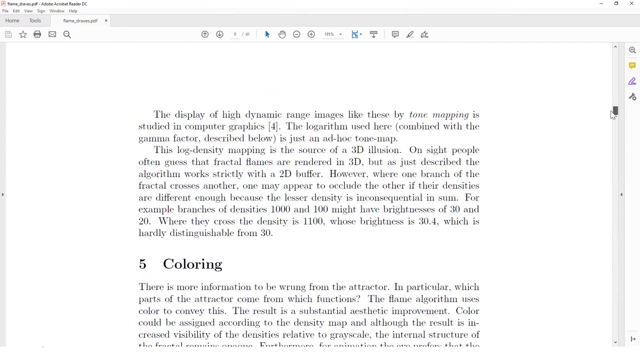 then mix all these variations or transformation into a single one. Like I don't get into equations, but I would just tell you the concept. So he explains lots of transforms here. Each of these transforms. what does it give you? You can put coloring, The coloring algorithm. 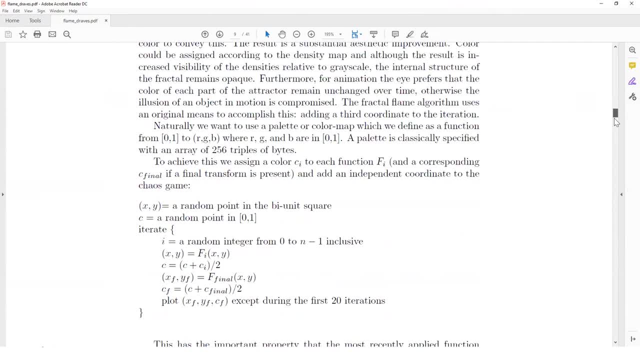 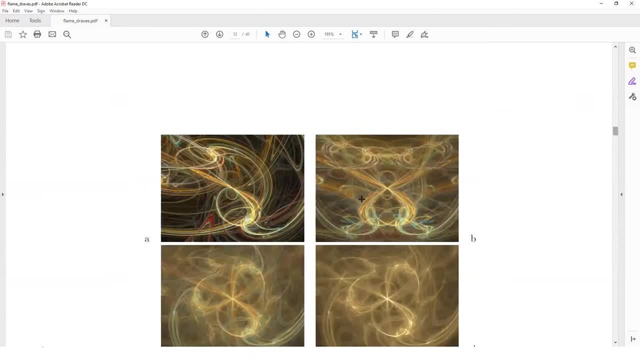 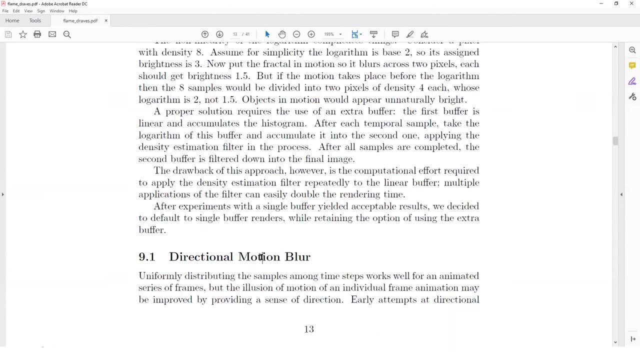 is explained here. Color or the density you can put. each of those transform can have different amount of weight attached to it. So here they will explain some of these transforms which can be used: Motion blur, These are all property that you can attempt to do it, But this paper 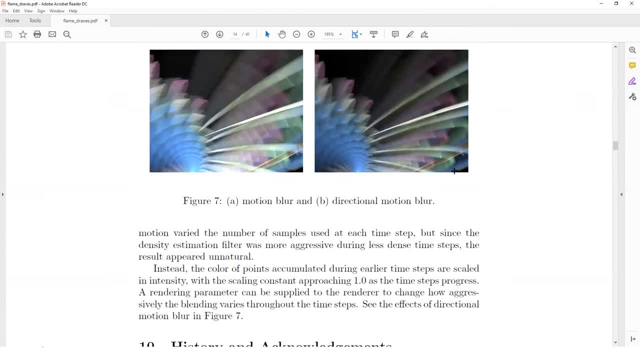 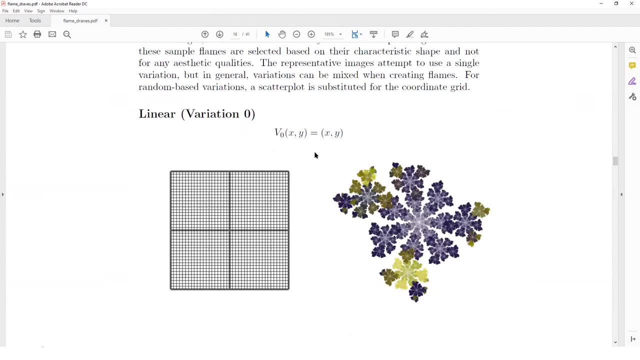 is something which I would suggest you read it if you have a lot of interest on how to do this. Where were the paper? Had those pictures? Okay. Catalog Variation, catalogs: Okay, This is a linear variation, But then in apophysis or ultra fractal, you will get lots of variations, Like you will. 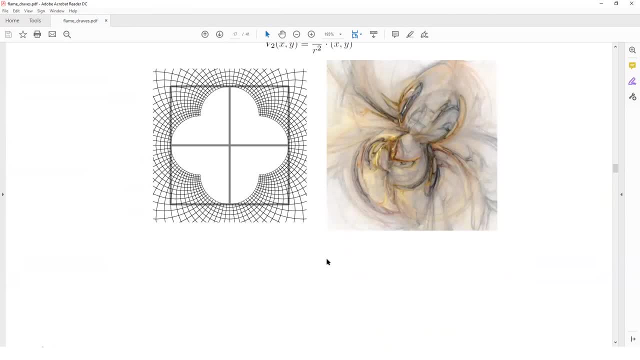 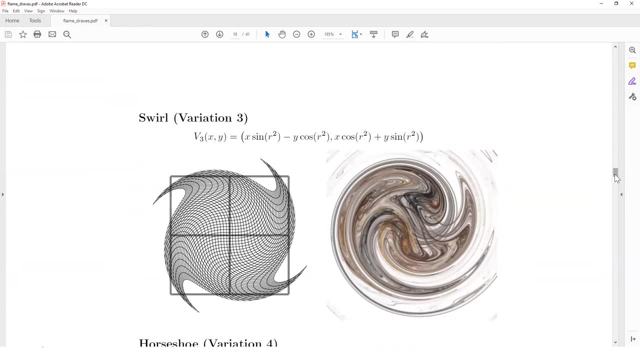 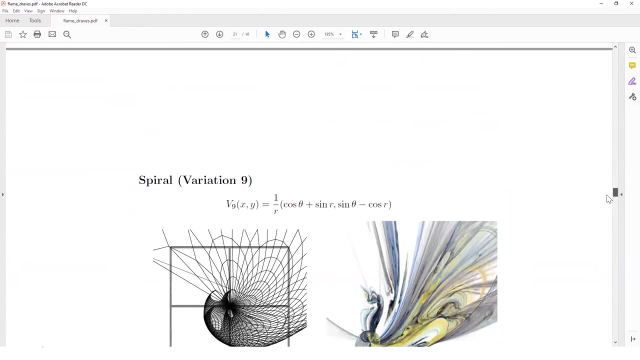 see it in the open source world. Many of them you could pick up. These are different variations. Then you can pick a mix and match of variations, apply the weight and then apply them differently so that you can create a whole variety of patterns. In fact, the apophysis program that 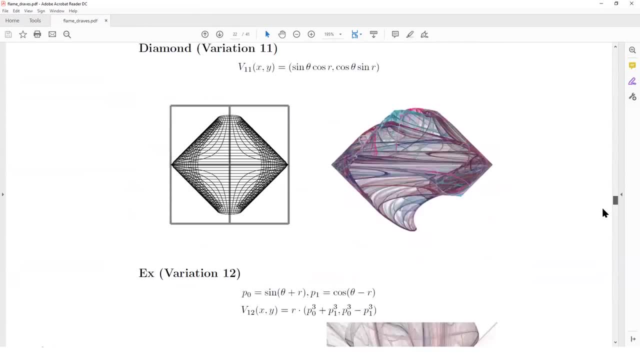 is doing this work. only, This is a flame rendering program. Pick all these flames and then do it. So they are explaining some basic variations. So they are explaining some basic variations. So they are explaining some basic variations, But this is a very heavyDaylight. 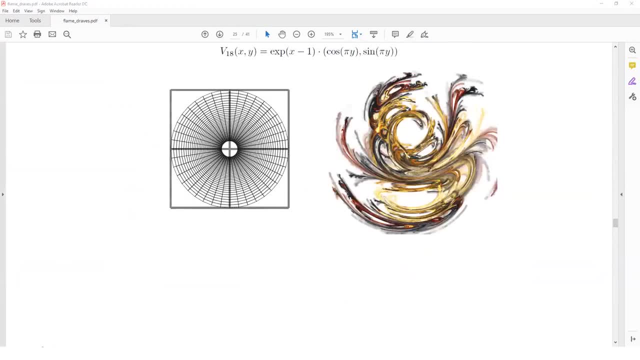 But if you are looking at querying or flame rendering or flames, what do you get it? I think I was showing that apophysis program right, I just picked some flowers here. Okay, These are, Julia. actually The way you are distributing. 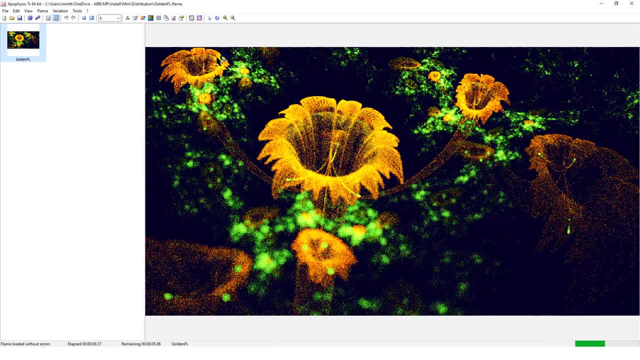 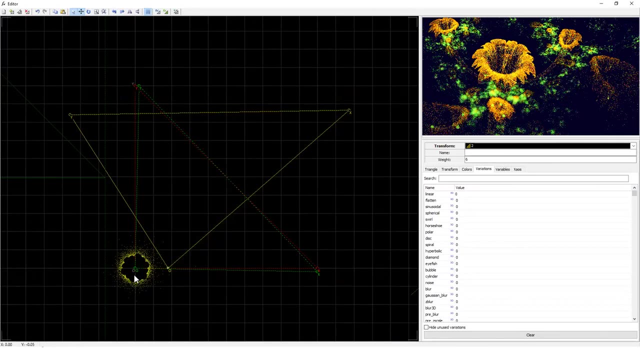 and seeing. it is Julia, But it is a very heavy one to render And what will you get? You have that, You have that, You have this. These are the ones that I made. These are the ones that- And one more reason why I say how patients is this- is usually slow in rendering. So if you come here, then if you click on them, they will show you what is that. this is Julia is there. That's what you see here. 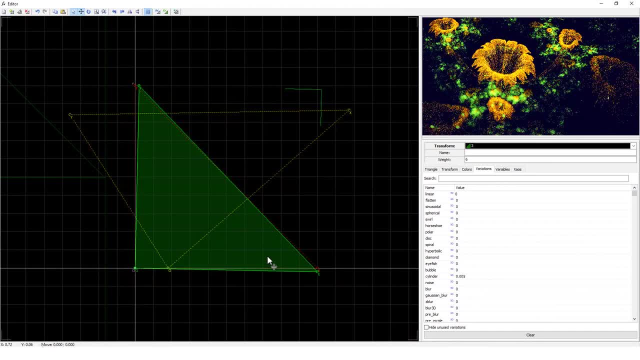 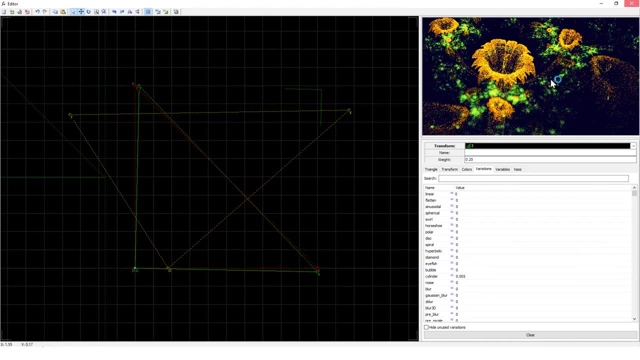 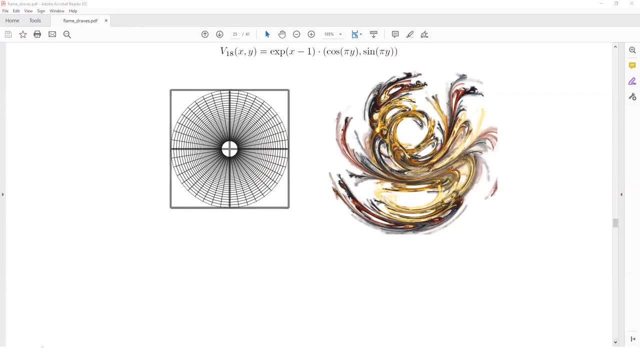 It's C, con and Julia, similar to the green one, green one, the That individual transforms, which they are talking about in that fractal flame rendering program. So if you get to this flame rendering algorithm, then then you will get what the apophysis, or ultra fractal, is doing behind. These are some samples of 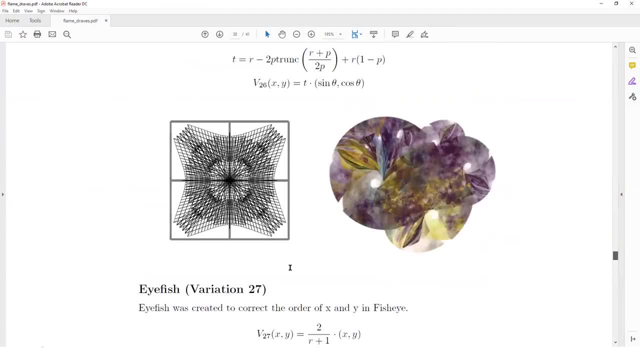 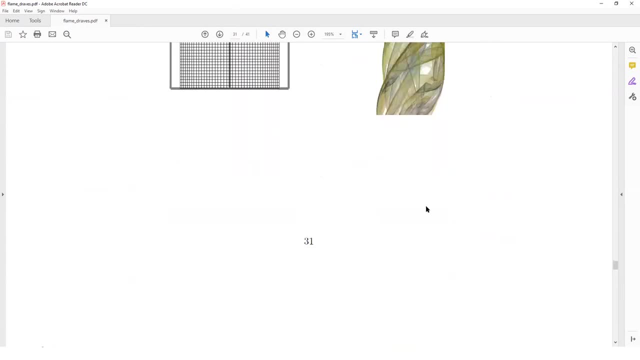 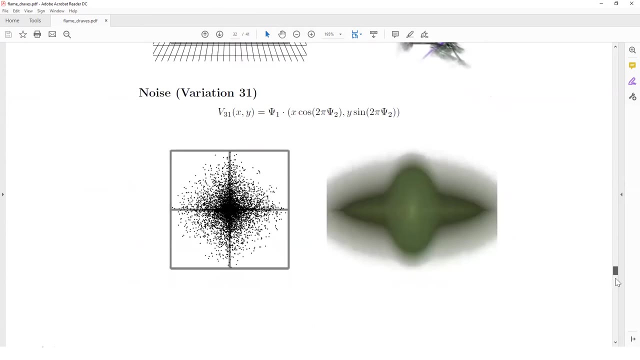 Variations which they have, you and they're all different. different equation: How do you transform one X and Y into another X and Y by applying various, various transforms. here Some are with the constant summer, with, Like some trigonometry equations are applied based on creativity. People are creating lots of. 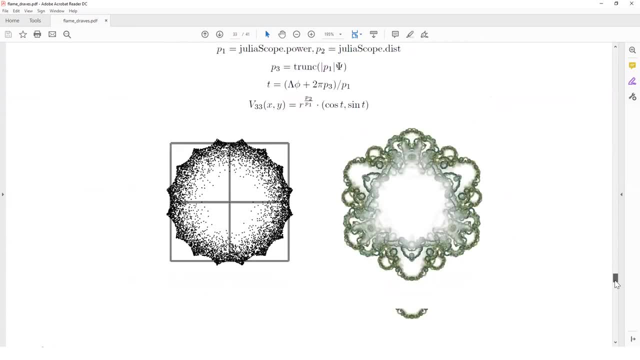 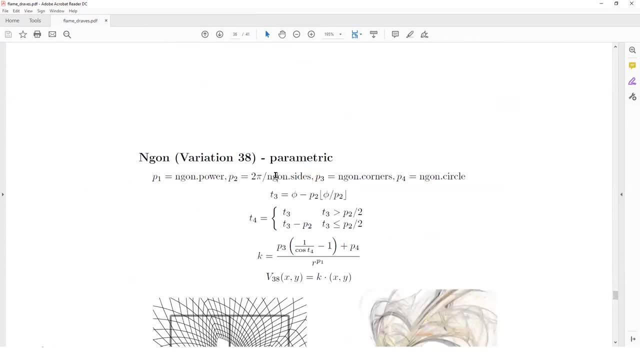 Lots of, Lots of Patterns like this. Okay, there's nothing like you should look at one or anything. So this is a score dress paper which is called the fractal flames. That's what Explains these kind of variations, and who has come out with that algorithm? electric sheep is the website by what they do is they are actually borrowing computing power. you can download the install that electric sheep, then they'll do some work in the background. 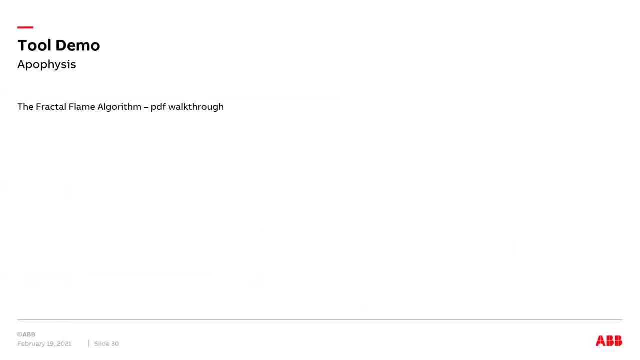 But It's come back. Any quick question or shall we go further? Hello, Silence, Okay, You can proceed. Then why do you want to do all this? That is your next question and in general, there is this: aesthetics that is associated with this and design these fractals. 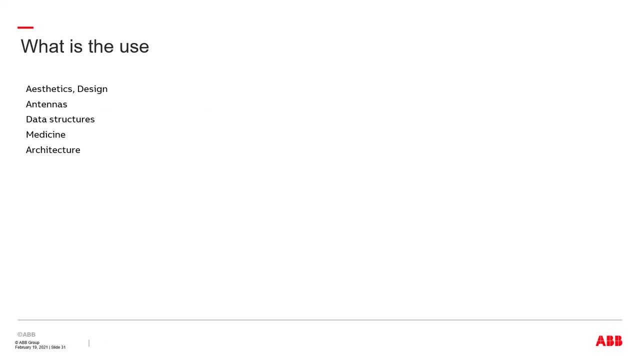 are also used by a lot of movie makers. if you see this- barbie movies or disney movies and all that- there are people who use that for creating artificial forest and artificial flowers and those kind of things. the movie makers do this for fractals, for creating those sceneries artificial. 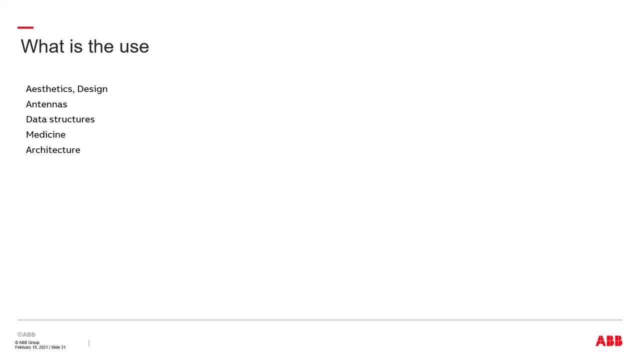 sceneries. that is one way people use. designs means: if you see there are, if you look at in youtube, you will see some designs which are created, which are inspired by fractals, and then antenna design. antenna design- why people use this is, uh, i think that is nisha nisha's favorite topic. nisha was in the 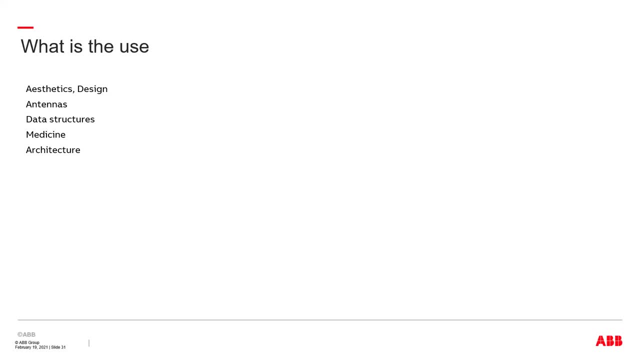 in the meeting antenna has this? uh, people wanted to have a lot of surface area and that is when you will be having this signal capture capacity. so for that, some people use this fractal pattern, so that your surface area becomes more, and data structures you can use this. 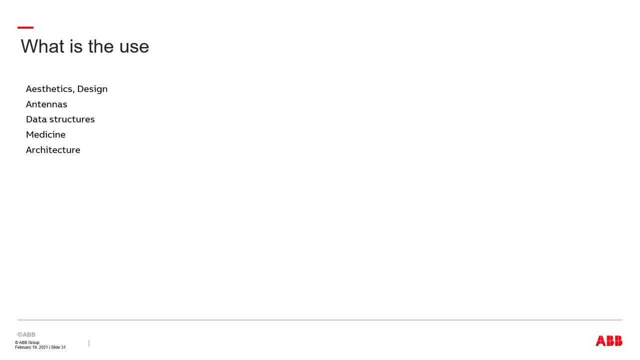 and maybe there is medicinal usage, on how people may want to follow the path of various things in the medicine, like maybe knowing that biology and the human- uh, a lot of the human structure is fractal patterns and architecture. there are also some people who design this architecture. 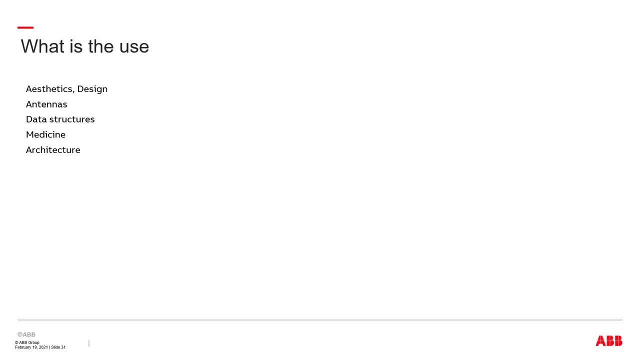 i mean this building architecture kind of things based on inspired by fractal patterns. there was a very beautiful video of this architecture inspired by fractal patterns and then zoom. this is one friend of mine who is made this zoom, so i had told him that, okay, i will play this video during my session. okay, 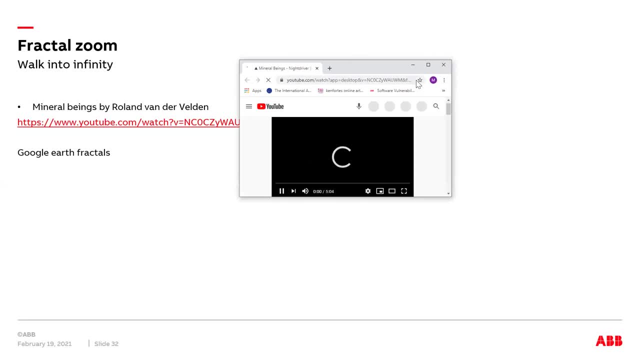 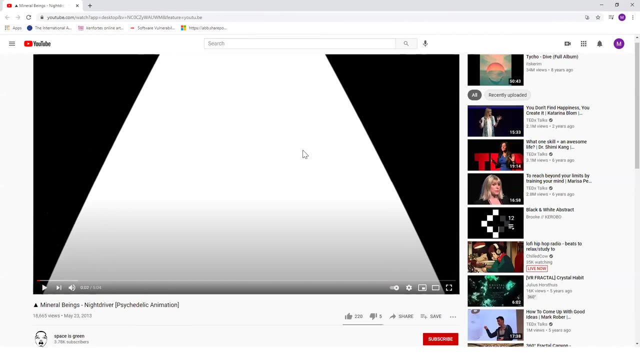 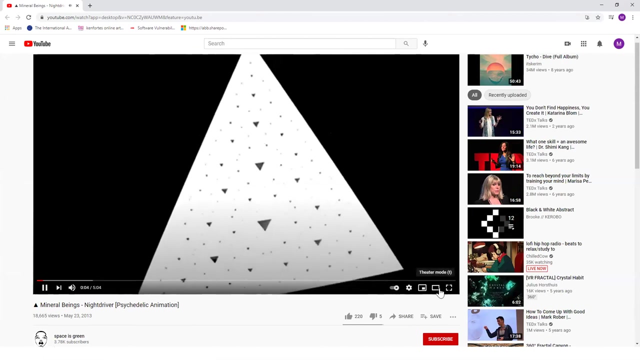 so i will show this. one youtube video is my. is the audio also shared, or is there something i should do for that? hello uh rengini or someone. can you please confirm whether the audio from the picture is also there there? okay, then let me play. just enjoy watching. it's just for a relaxing time, okay. 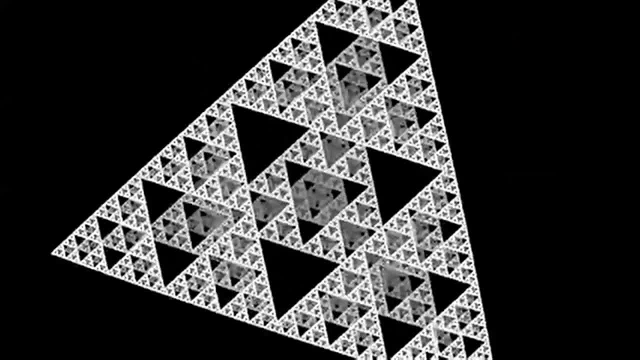 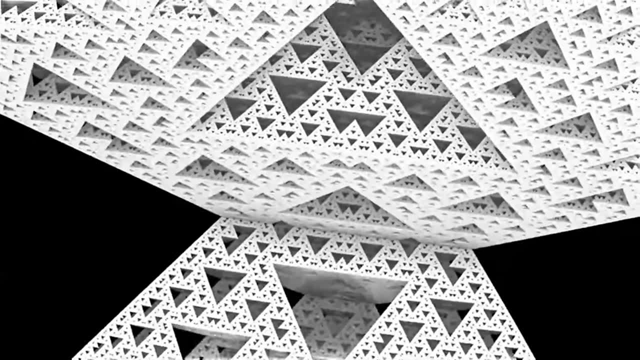 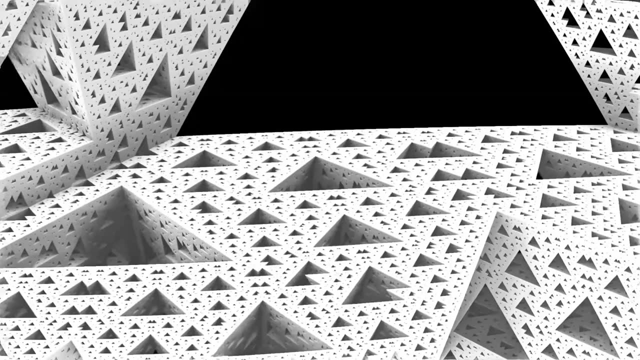 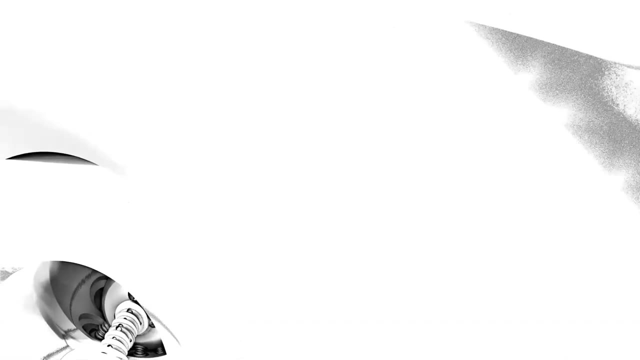 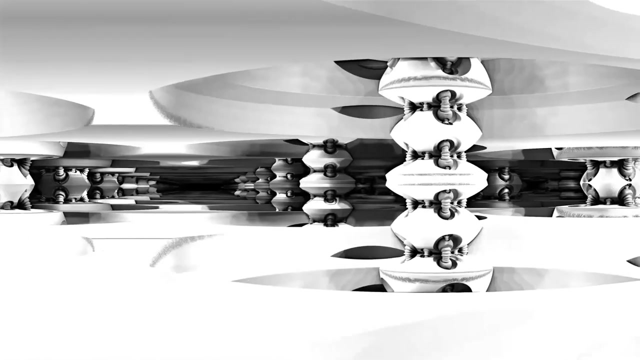 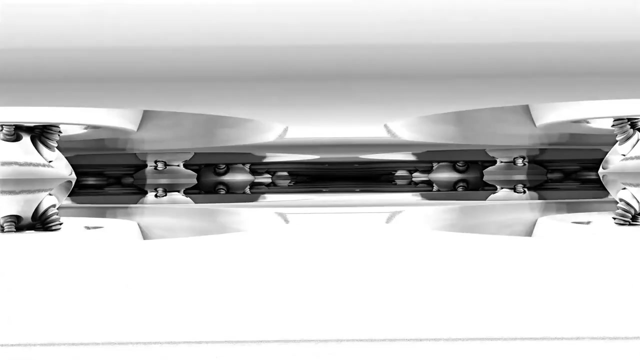 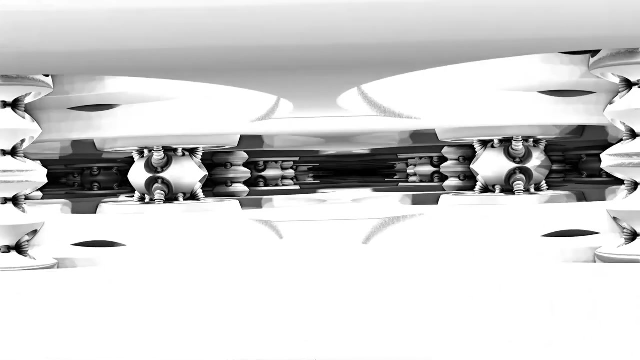 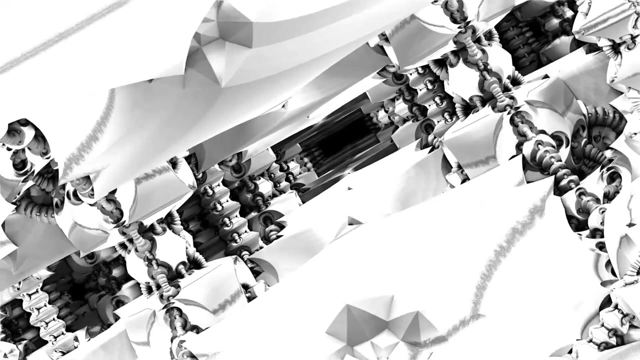 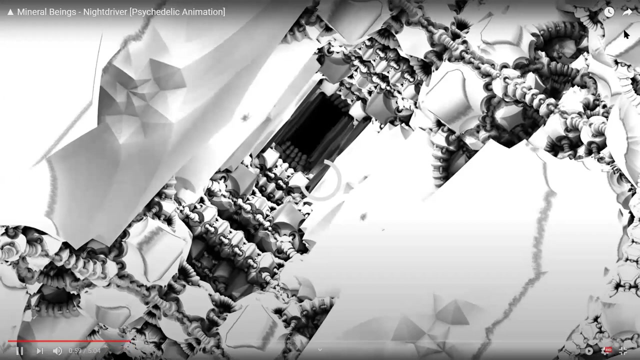 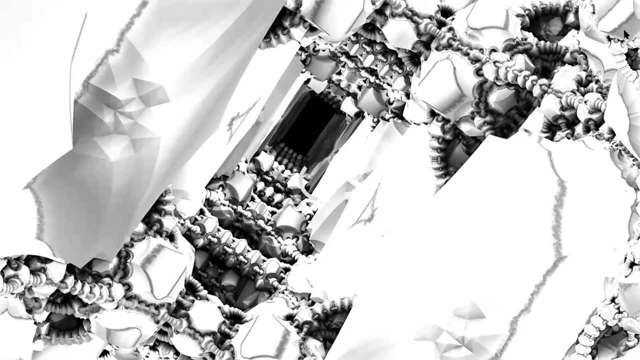 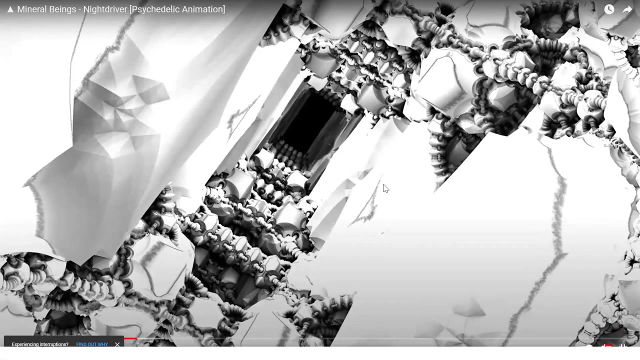 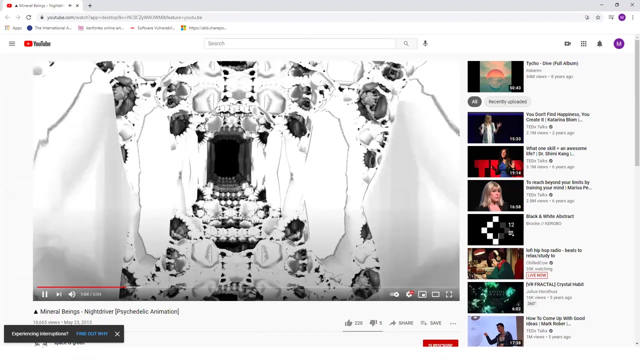 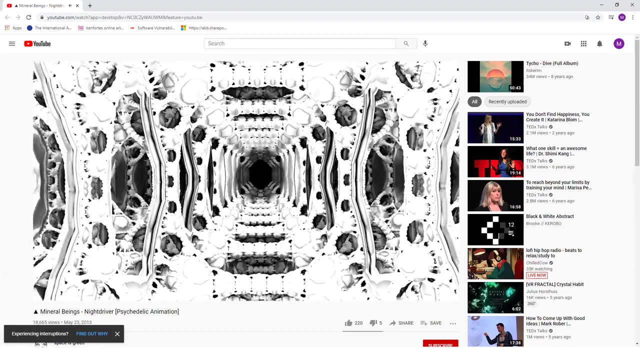 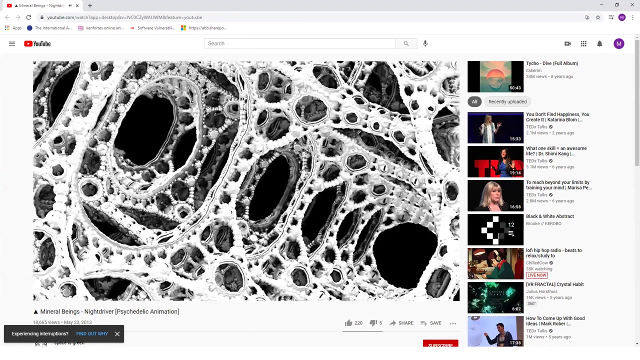 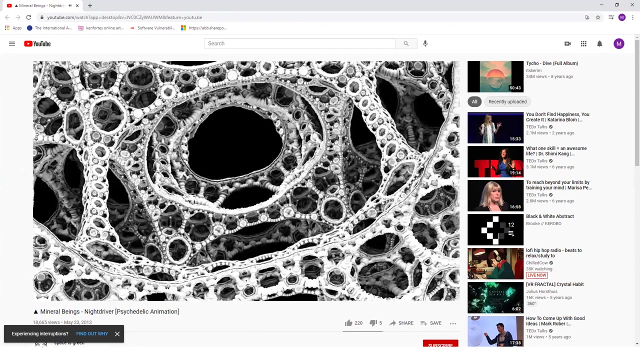 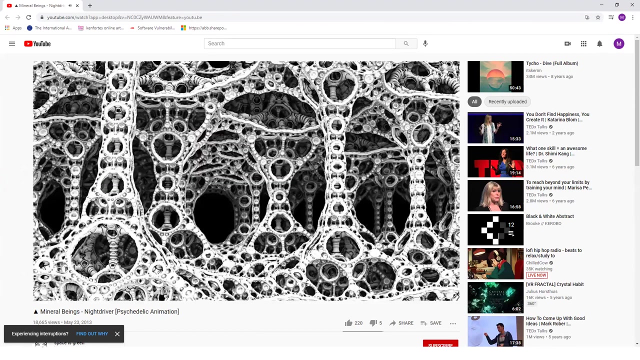 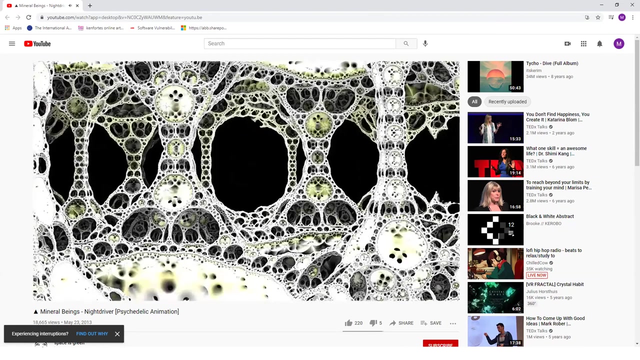 yep, Okay, it's just a little bit of a problem. I'm facing this network not so great. hopefully it'll come. I think it's a little bit of a problem. 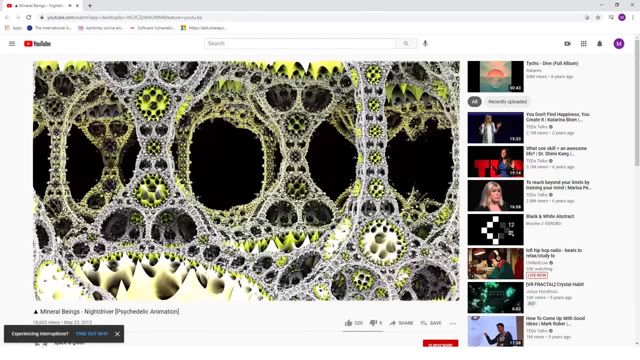 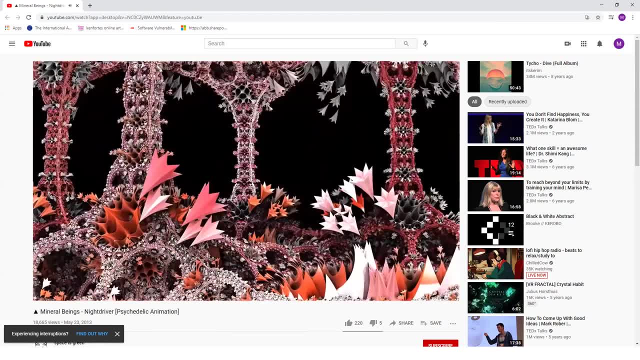 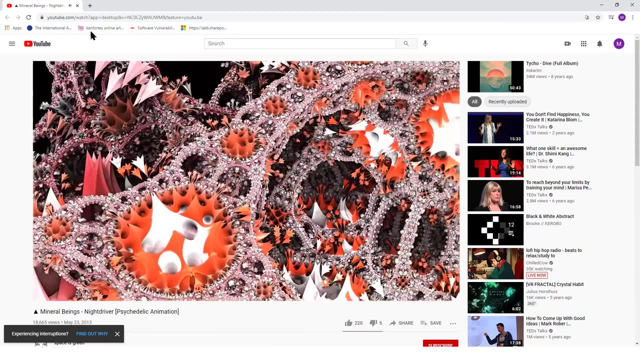 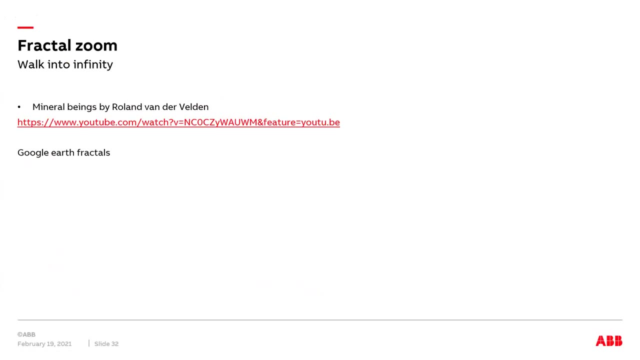 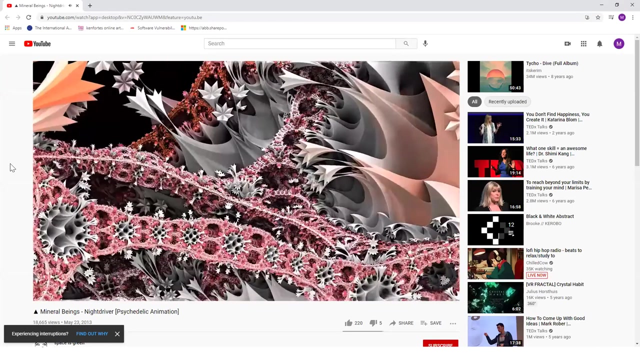 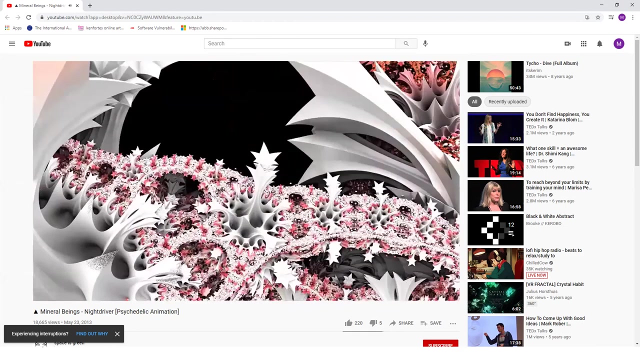 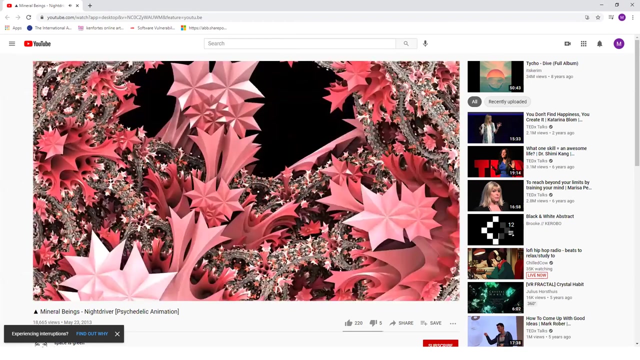 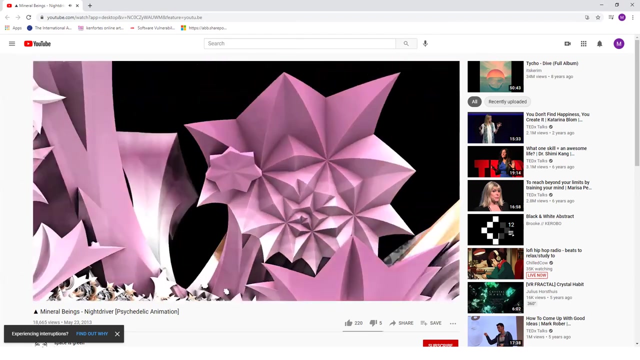 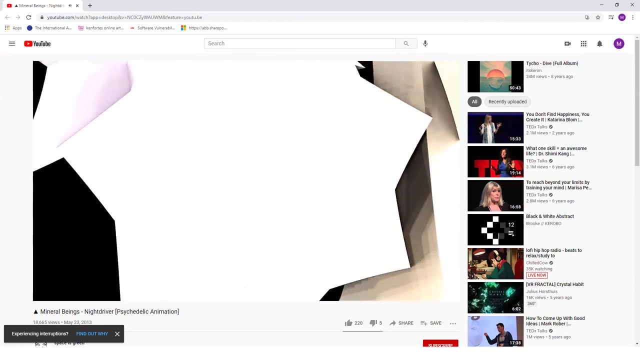 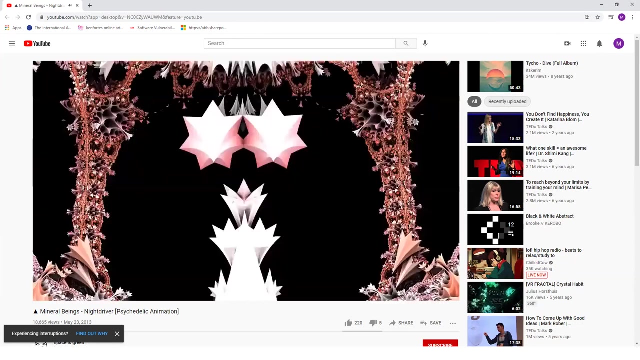 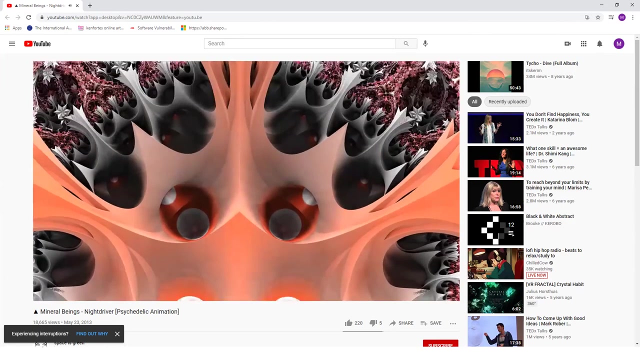 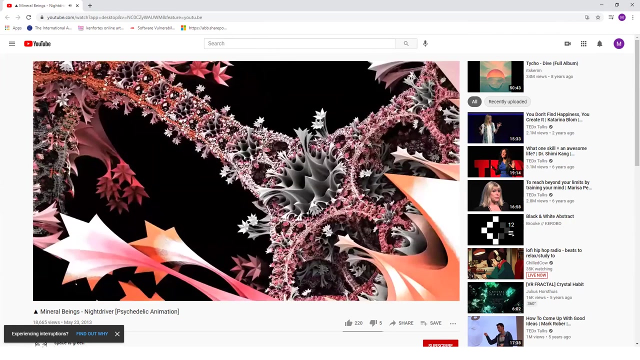 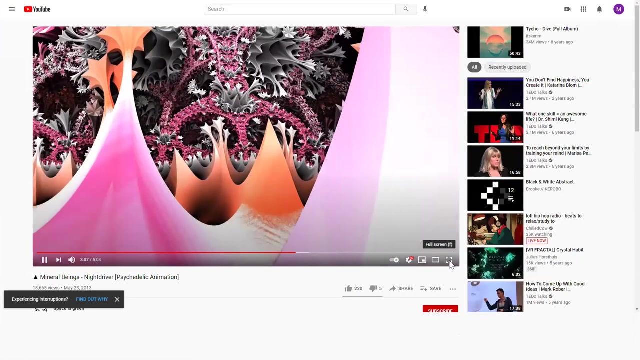 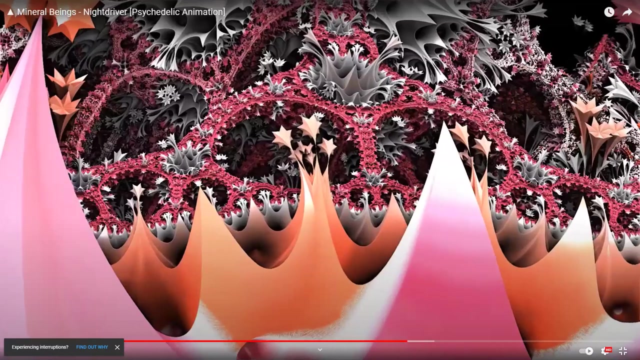 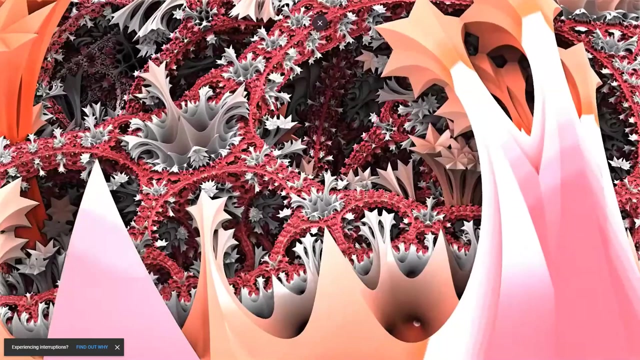 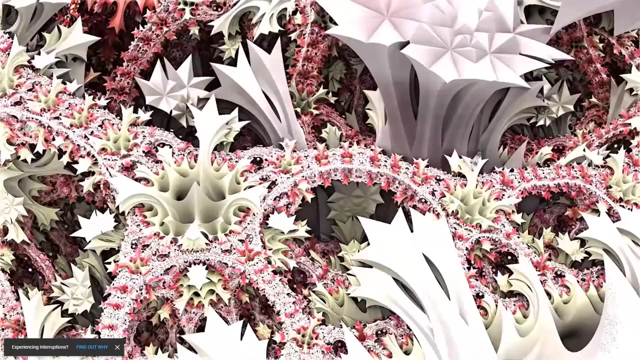 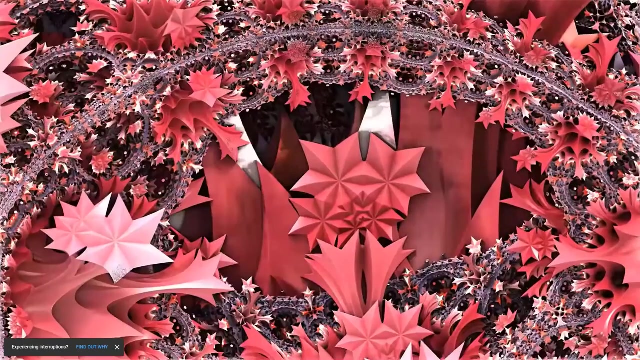 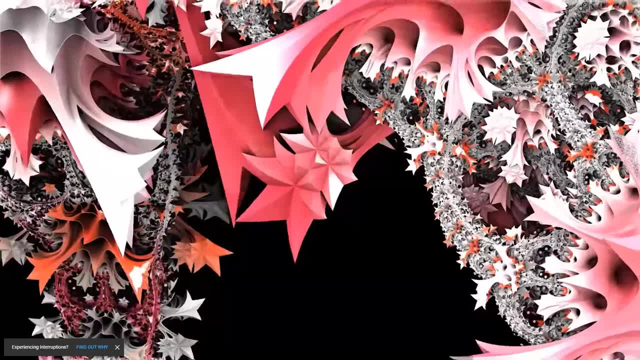 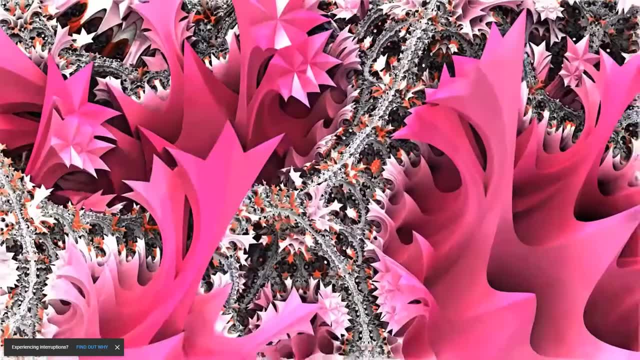 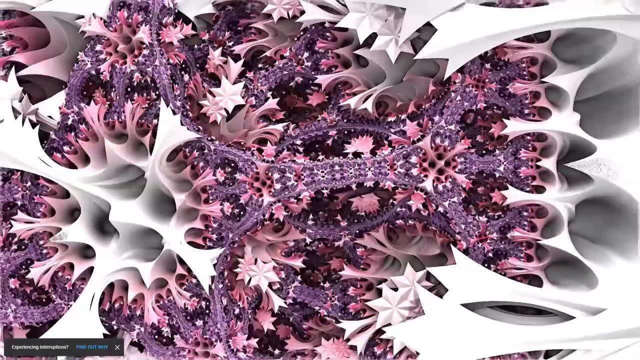 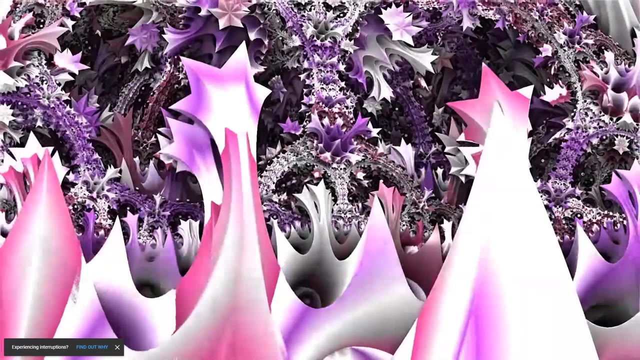 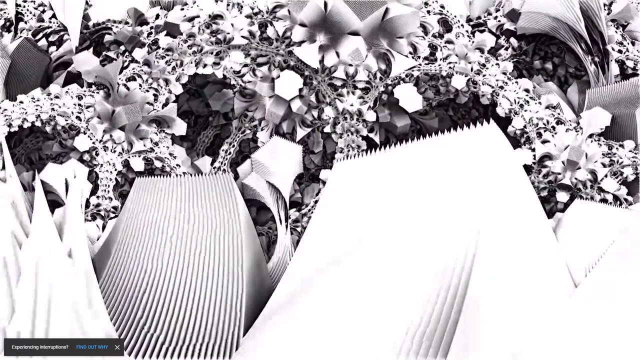 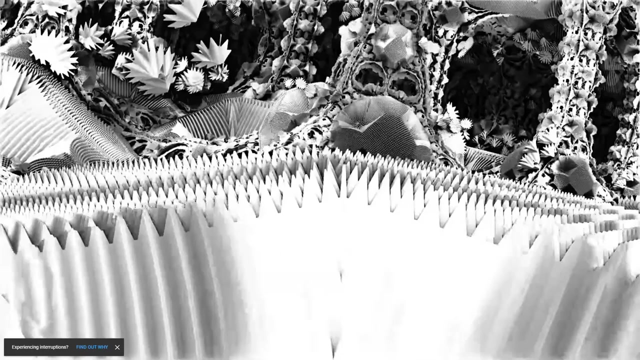 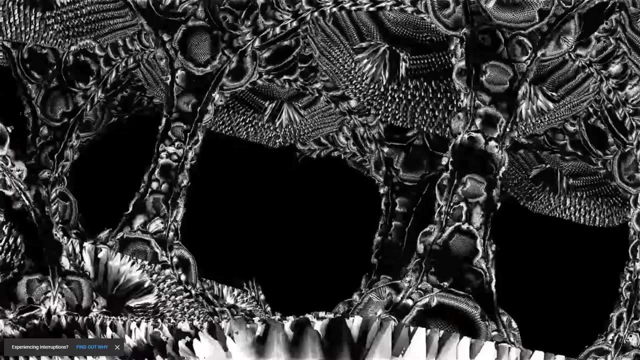 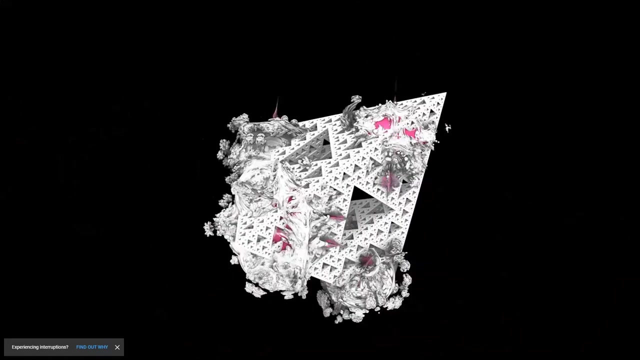 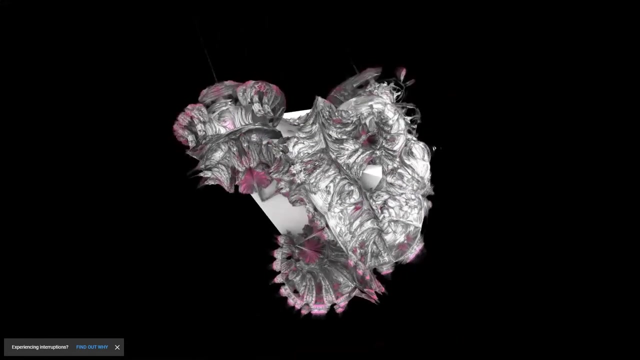 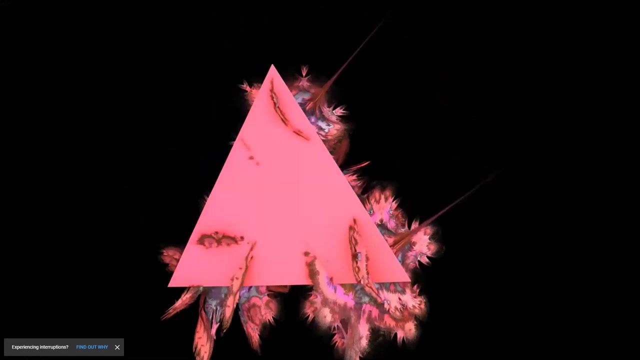 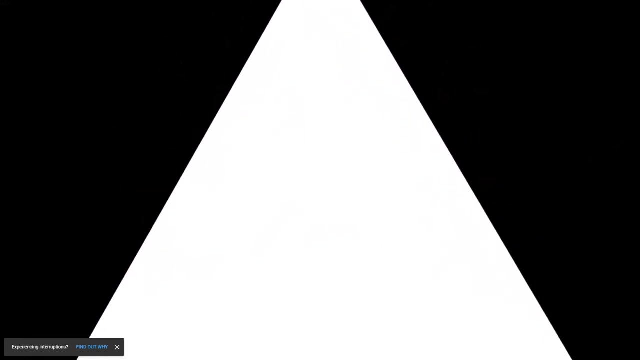 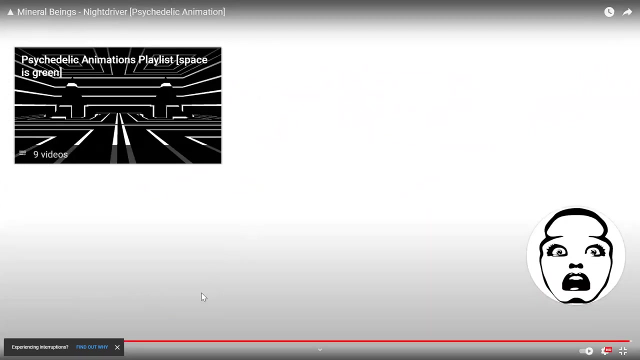 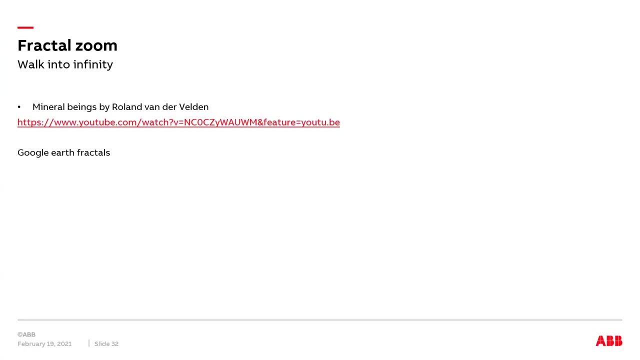 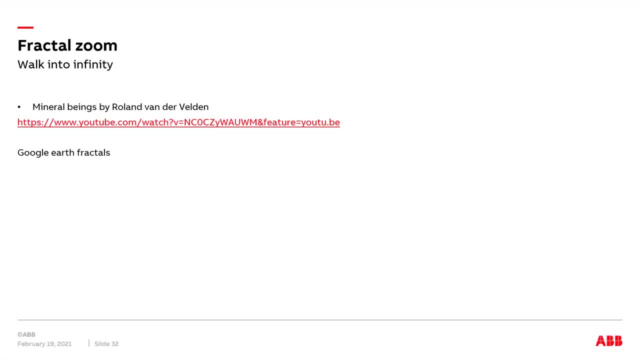 Yeah, So this is one person who I know he creates this. I have not grown up to This level of creating things. One is it because I still haven't started to pay money and buy programs for doing all this. Because if you want to do this level of 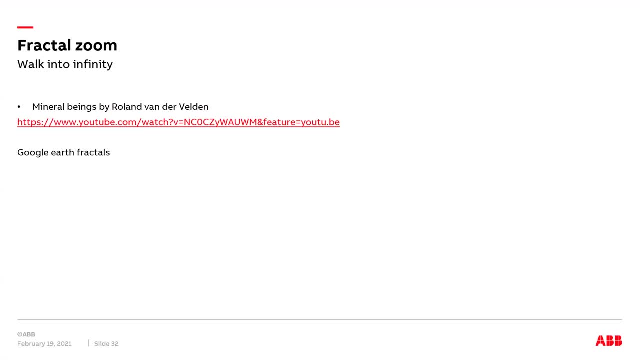 zoom and fractal zooms you can look at in the YouTube. fractal zoom- you will get a lot of videos. But this is something which, because I know this person, I put it and I haven't grown a lot to that level. maybe i should try, with this much of interest, to spend some money and buy some ultra. 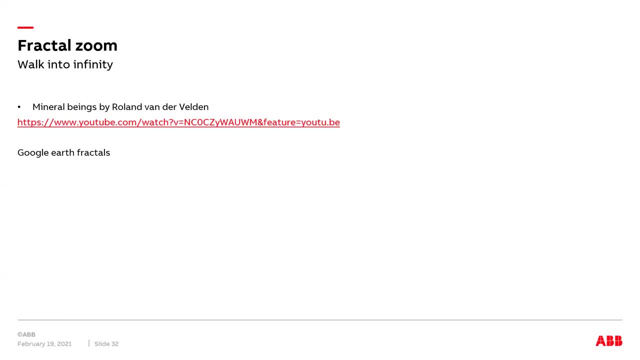 fractal, ultra fractal, has these kind of features where you can mix music as well as create this zoom inside the open source programs won't take you to this level of detail. it's a very interesting field, i guess. yeah, i think, if it has to hold my interest for this much time, then it is very interesting. 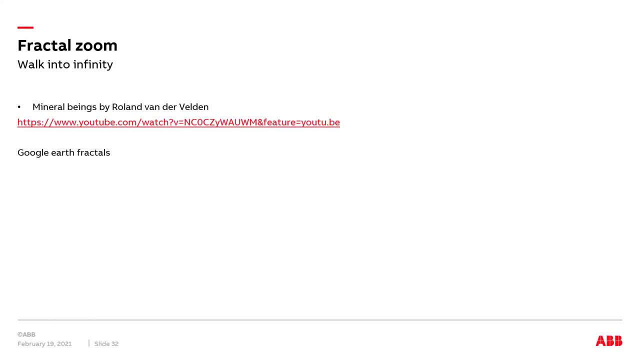 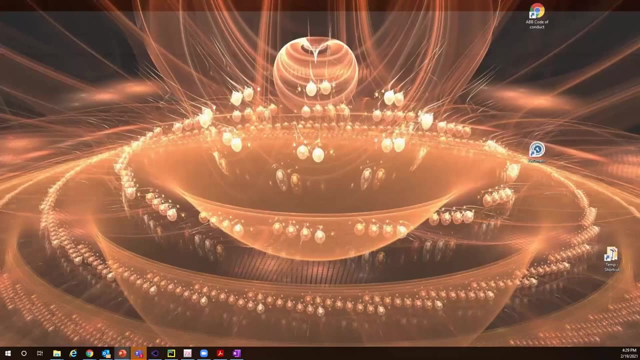 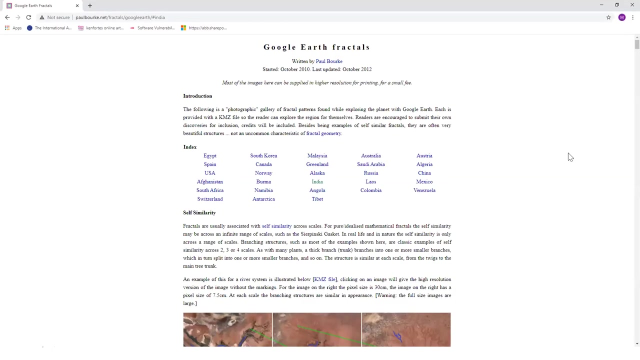 and i'll also show you something. yeah, in fact, i am coming to more or less to towards the end. i'll show you something which is even more interesting. that is, where do i have see, if you look at google earth- okay, i was telling that- lot of patterns inside in nature. they are all. 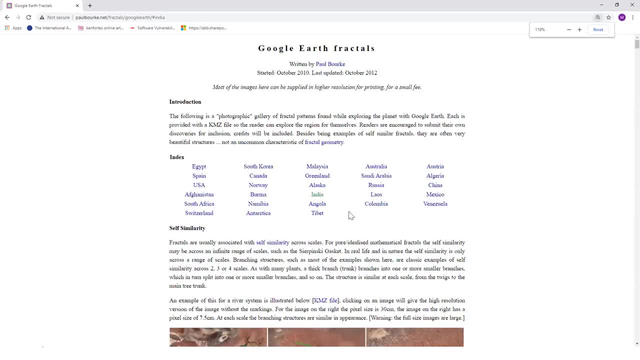 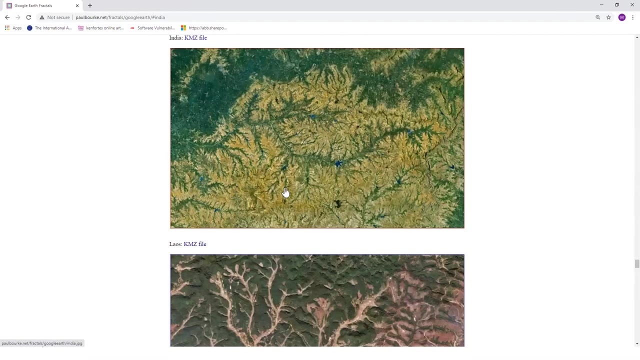 fractal patterns. i was telling that right before. so these are captures from google earth. if you are looking at google earth, you can see. then you should be able to see fractals, right? so these are all patterns. so i only have put some patterns from this country, india, where i don't know where exactly these are they. 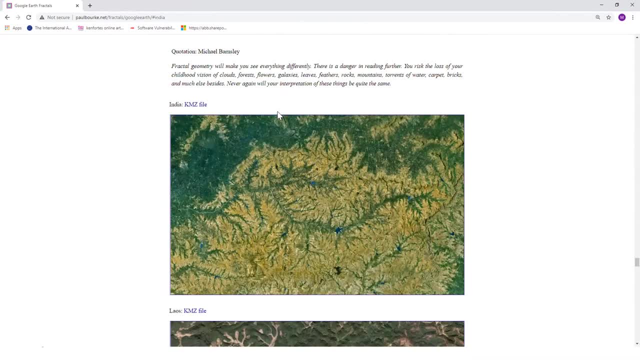 must have given the coordinates somewhere, so i liked that sentence that we have. they have written there also the google earth captures. these are like you play around on google earth. you go find out pictures in google earth and then you will see them. these are just screen screen captures. 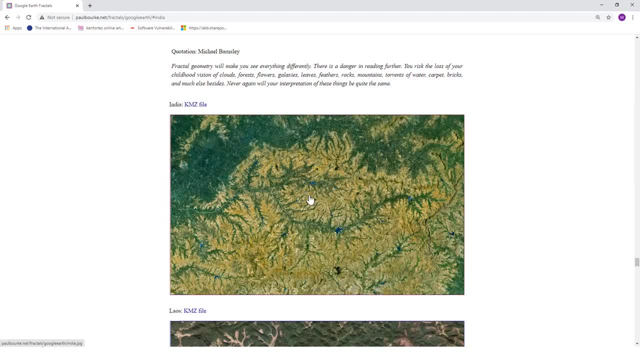 from google earth, okay, no. so i found them very interesting in the. this is public domain only, so i thought, okay, maybe i should show it. see what, though, he is writing. there is fractal geometry that will make you see everything differently. there is a danger: in reading further, you risk the loss of your childhood. division of clouds, forest flowers, galaxies, leaves. 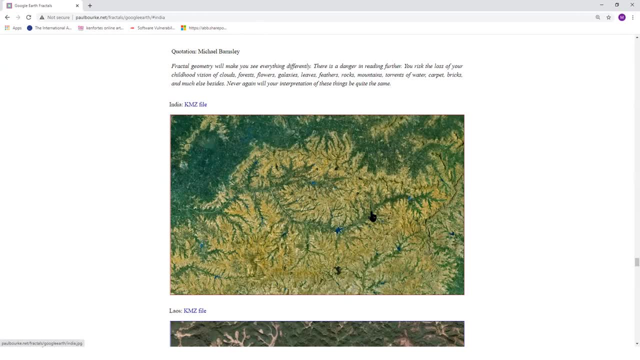 feathers, rocks, mountains, uh, bricks, whatever it be, never again you will see your interpretation of things as quite the same, but i don't know with me what has happened, whether i lost the child or after in the last from 2016, i think i'm doing it for past four or five years, so whether i regained 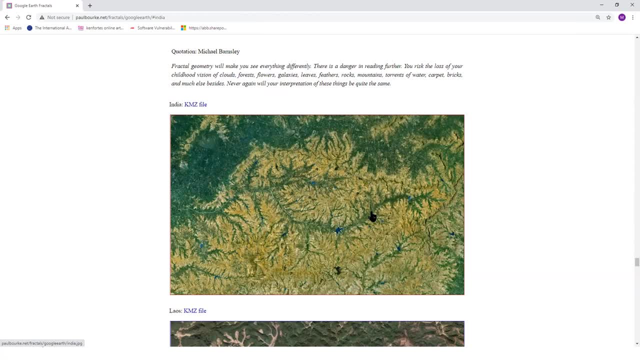 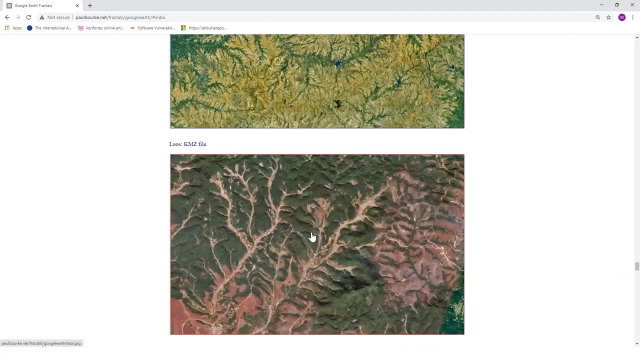 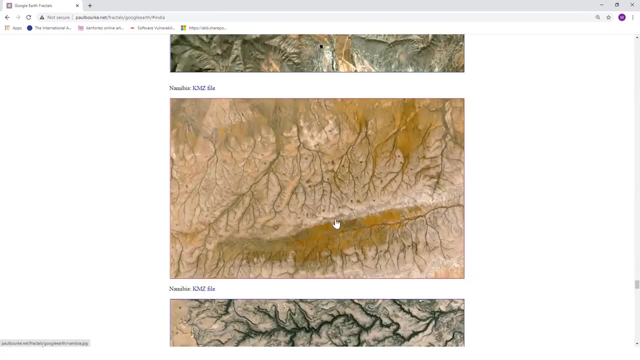 my childhood, or whether i maybe for small children who may lose their childhood. maybe you will regain it again, but these are google earth capture pictures from various locations. these are from various locations in india itself. like you can see how these rocks and rock formation- or this must be some rivers or dried up patterns- how they are becoming. 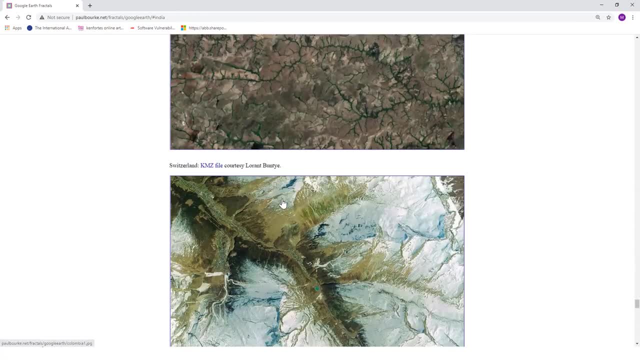 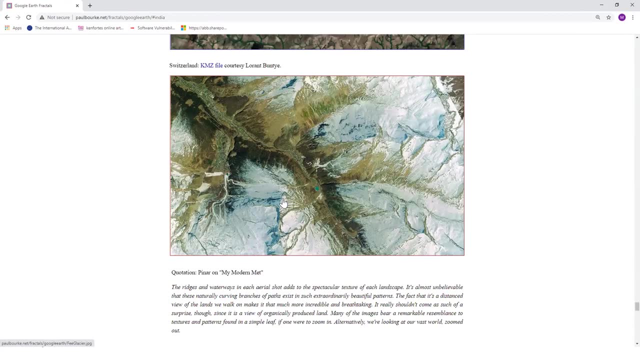 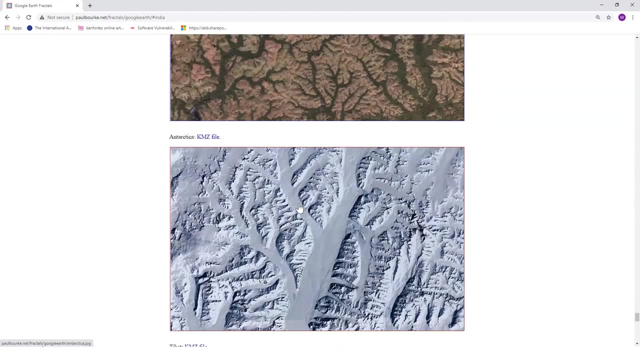 fractal patterns, amazing patterns. this is what we call as the complexity and the emergence philosophy that being talked about itself. like it, it gives you a different outcome based on where you are starting, and small change is enough to create huge variation when it is applied over a long period of time and, in that, to a larger system. 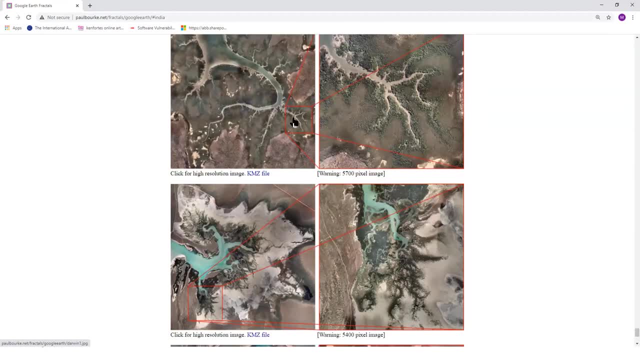 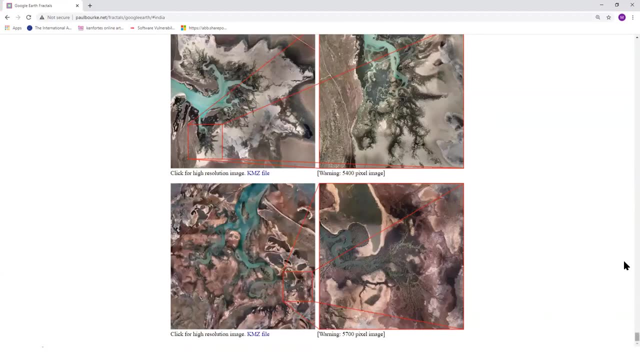 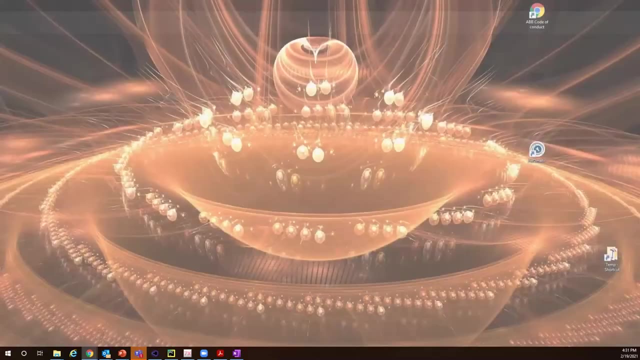 like this. these are google's captures which you may not even think of. what is there? see? they pick this one area and how it has come? very interesting patterns. so these are all what i am doing for time, pass interest for time. then i have put some references here. maybe fractal foundation, these people 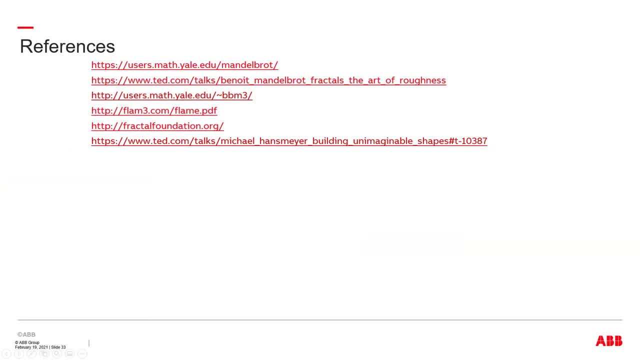 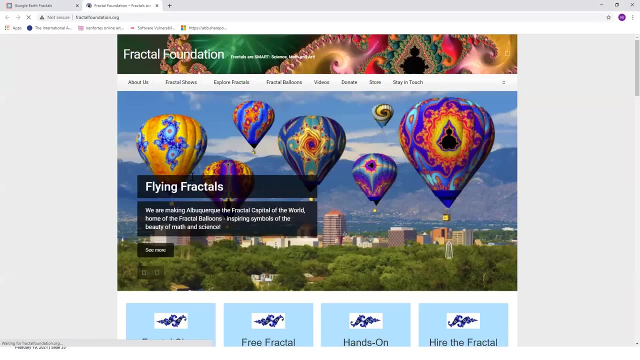 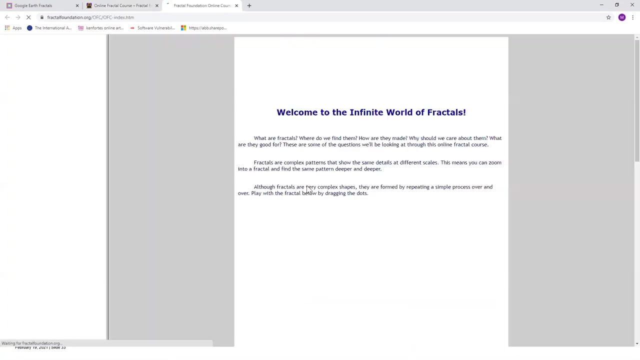 have some tutorials and all that. if you want to understand basics, see. fractal foundation is a very interesting place you can. they have a lot of a lot of resources there, like they even have some tutorial. explore online fractal course. okay, like some of the pictures i showed you are taken from this online fractal course, 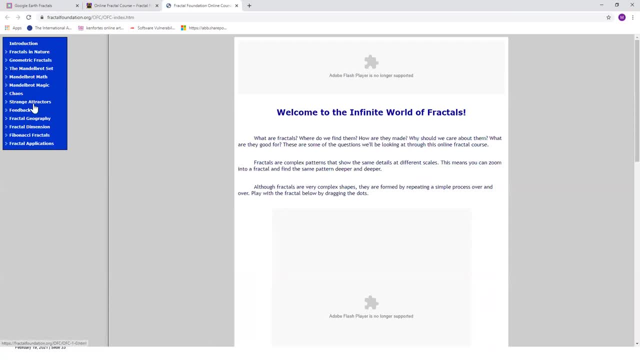 they explain what is kaios, strange attractors but kaios, and strange actors and all i have learned from some of the other mass book and maths packages, but then you could pick from anywhere. see they like fibonacci sequence. you must be knowing this fibonacci sequence. 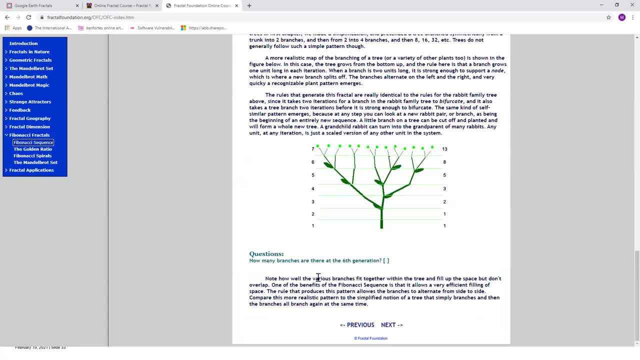 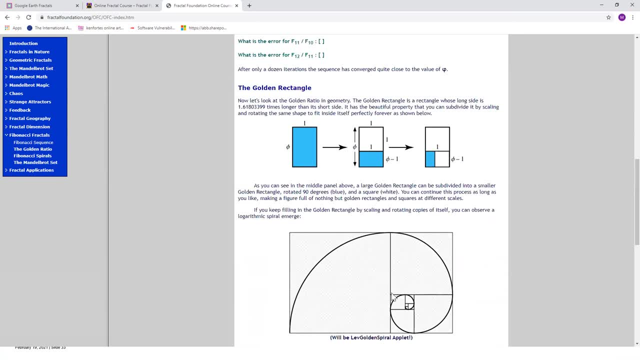 and this rabbit breeding story. you must be knowing it. you could go and pick and then see where they are. they're very interesting resources. uh, golden ratio, fibonacci series. you will be knowing all this. i don't think i need to explain all this, but then these are interesting materials. so now, 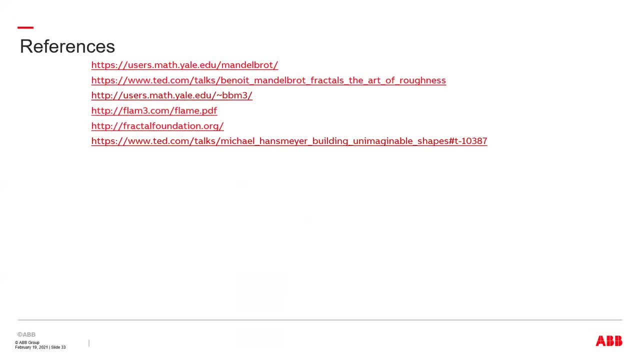 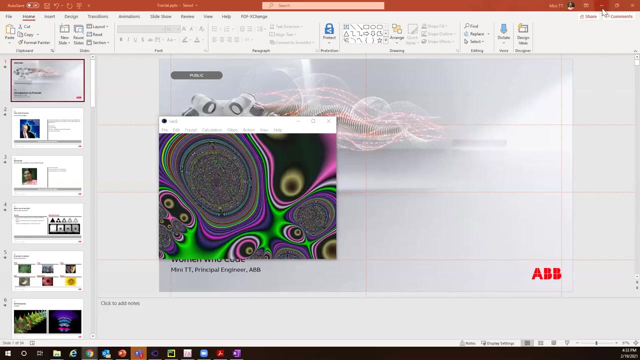 i'm waiting for questions or comments or feedback or opinions or fascinations or whatever you want to see or whatever it be, and if you are interested in seeing some more of my pictures, i will show you some more of my pictures also. yes, i would like to see the pictures. you want to see more pictures? okay, 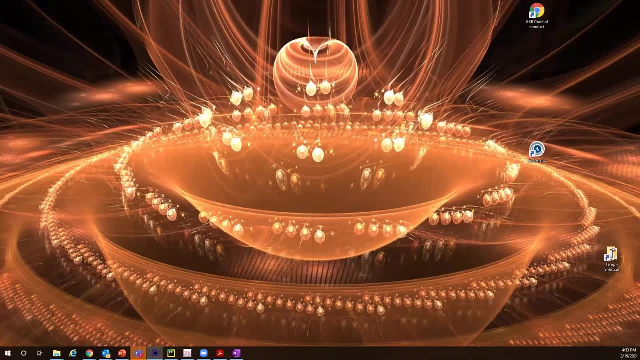 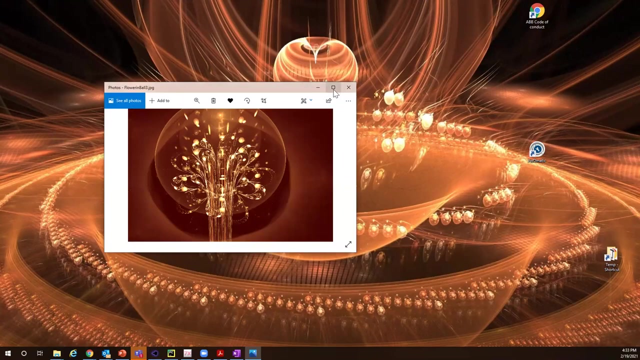 i have no problem in showing off, so let it be so. these are things which i had created in the recent times, maybe sometime. what you see in the desktop, you see that desktop picture right right now. yes, that's also one such picture. only, wow, somewhere in the galaxy looks like- yeah, some people say that it looks like some chandelier. 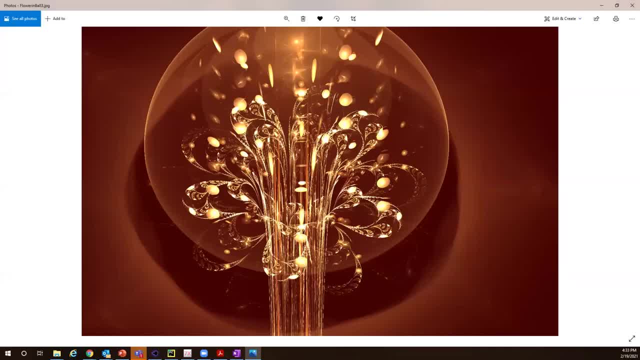 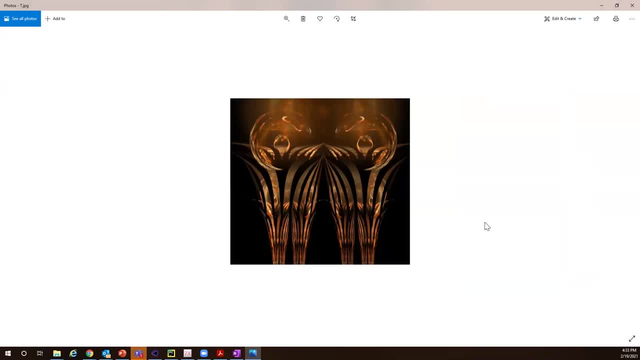 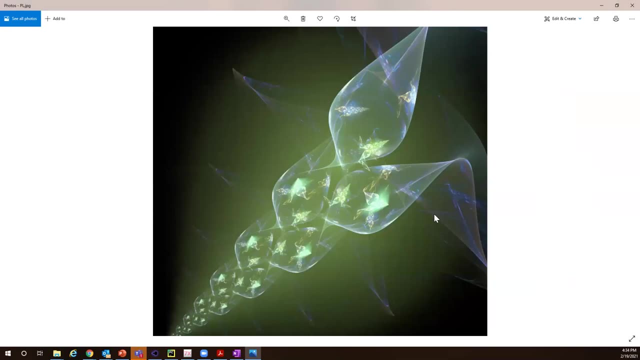 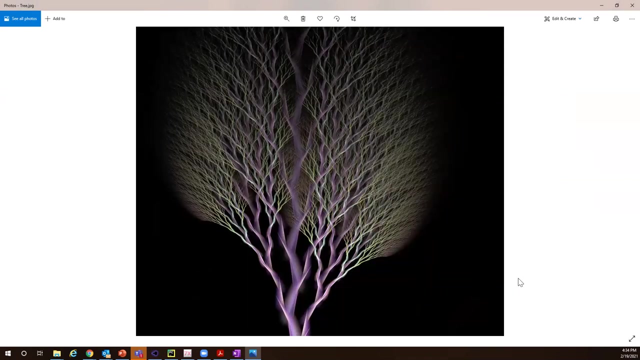 fancy chantelier. yeah, yeah, these are some other pictures. why do i say play? next i'm planning to put start a graphic business t-shirt. you want to do the graphics designer? yeah, it's very. these are something which i have created recently in the christmas holiday time. this picture, i like this one very much. it's extremely simple, but it looks very nice. 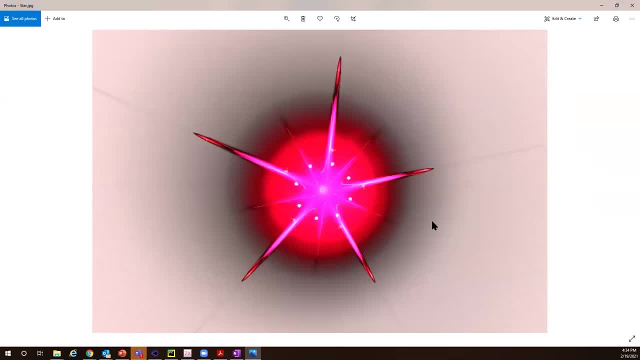 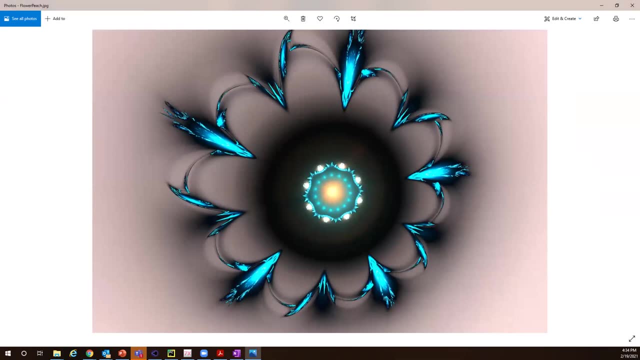 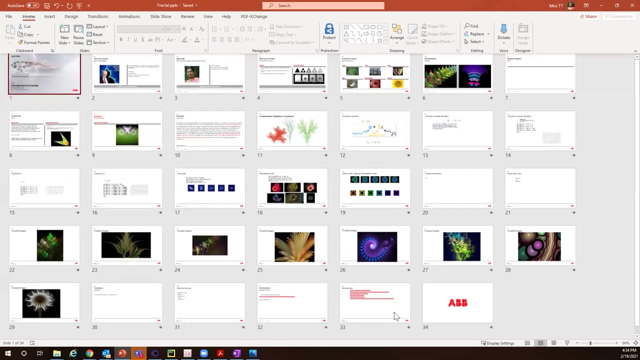 somehow i like the color combination mini. and there is one request: to put all the references in the chat window. if you want to copy and put the references in the chat window, okay, why not? and the slice slides? will it be shared? i don't know whether i should. 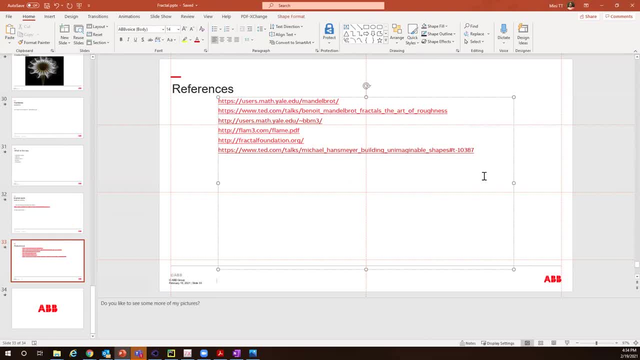 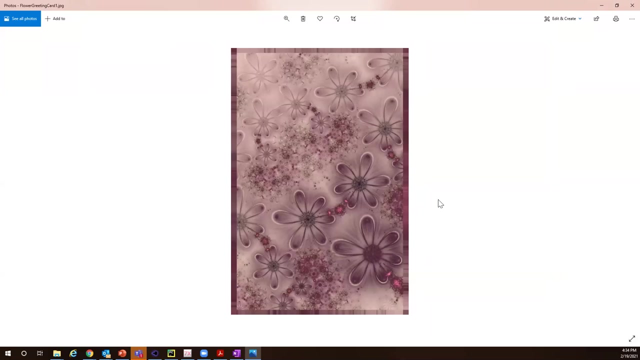 let me think of shiva. okay, okay, references i have pasted here itself. okay, we were seeing pictures, right? yeah, this one also. this is something which i like so much for the reason that even that edges that you see there, all these are from fractal rendering. it is not edited in. 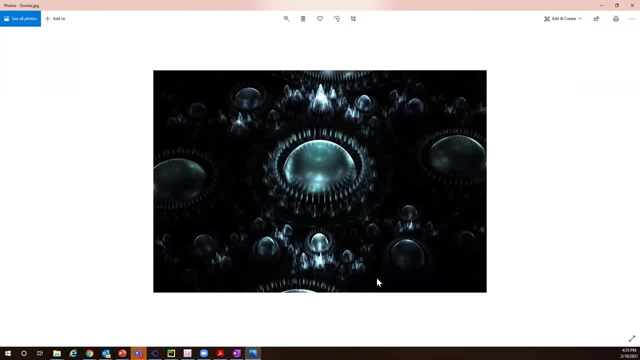 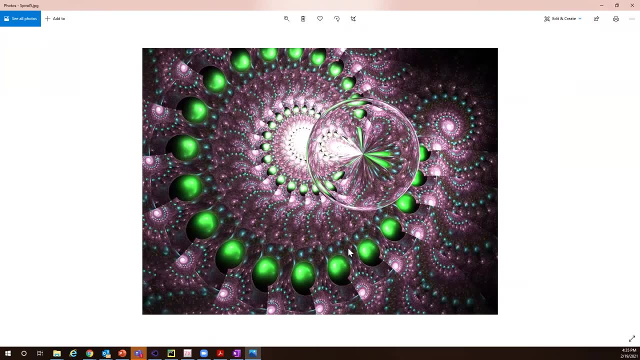 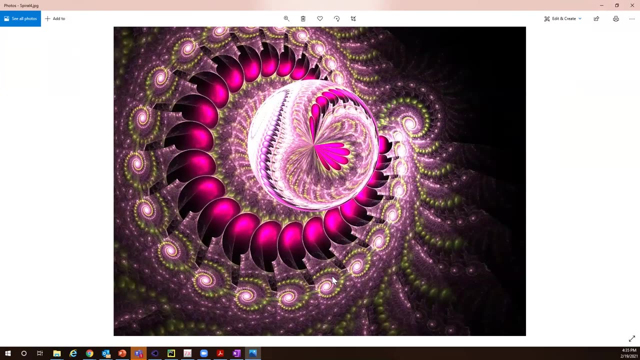 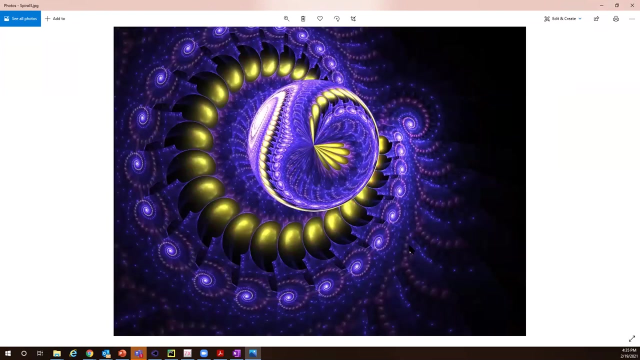 photoshop or somewhere. oh, oh, this one. i have created so many with different, different colors, because that was a time when i was getting interested in the colors. you can see that fractal geometry. once i have explained, you will see that. see, the bigger pattern, even the smaller patterns, are the same, whatever you see around. right? yes, yes. 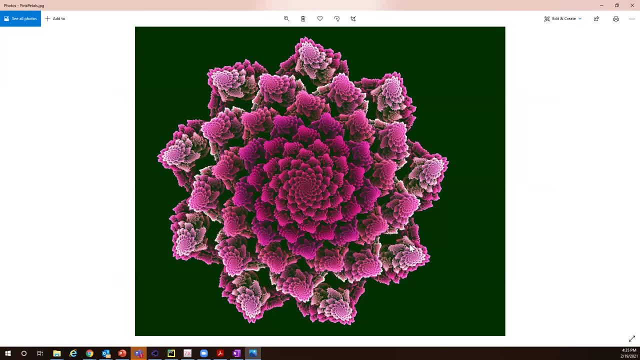 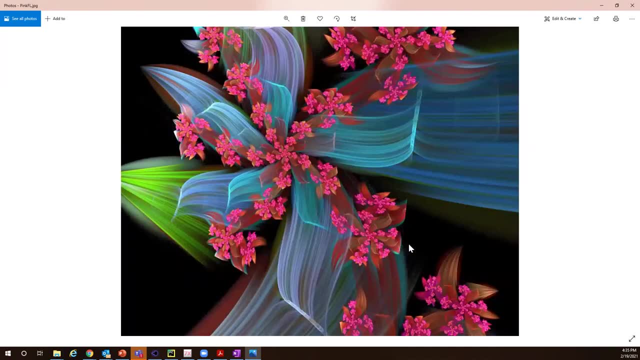 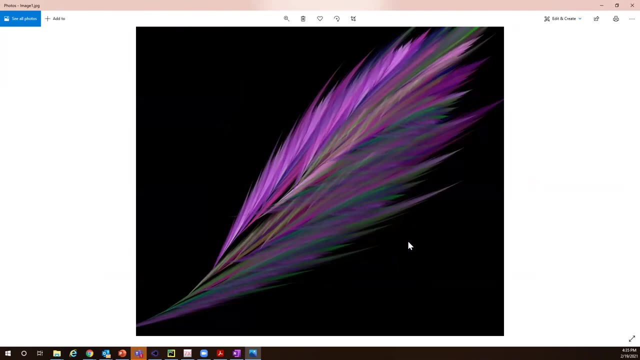 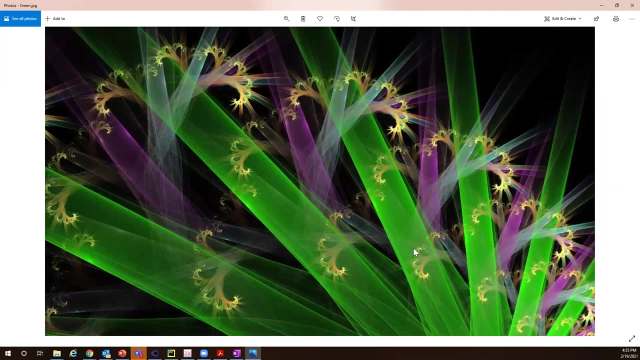 so nice, beautiful they are. you said that the greatest Reserve picture that you've ever seen. so would you look closer? actually, that picture that was created now was mine. none of your pictures have got that Grand fazer. these pictures, i think my number fancy. in fact, these are pictures which: uh, this also. i like this. so many flowers, right. 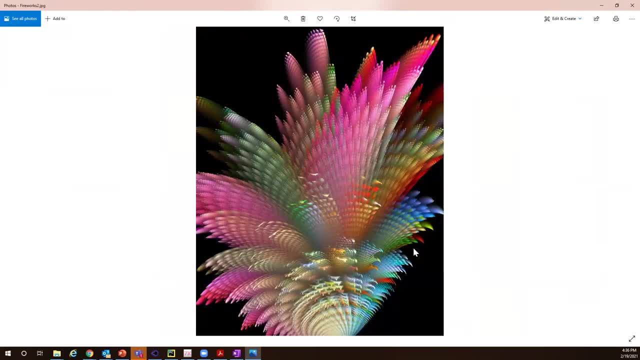 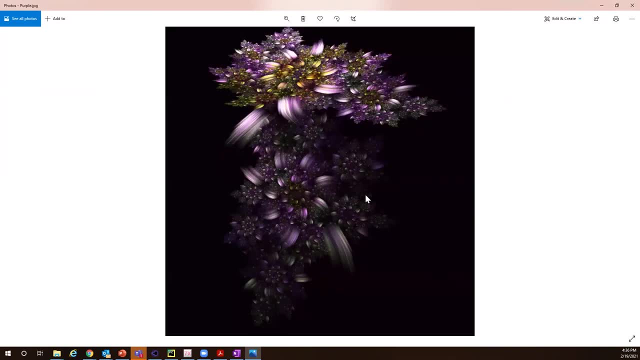 that is distributed over julia. not all of them are great pictures. i'm just showing my folder. i wouldn't have spent much time but created all these bokeh pictures also. i like there are so many here. okay, my system is having full of these kind of pictures. it's so nice, it's good. i think. 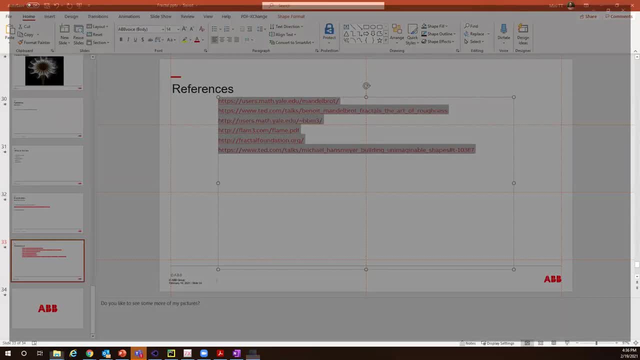 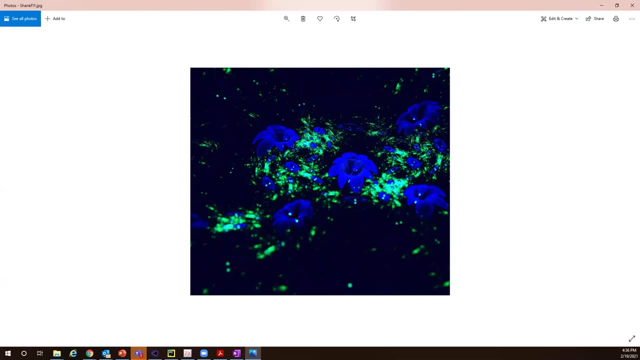 maybe i'll show something which is this one, something which i am very proud of. this is something which, because the it was a challenge to differentiate that flowers blue and the plant green and keep it there right, so somehow this one is something which i like it so much. 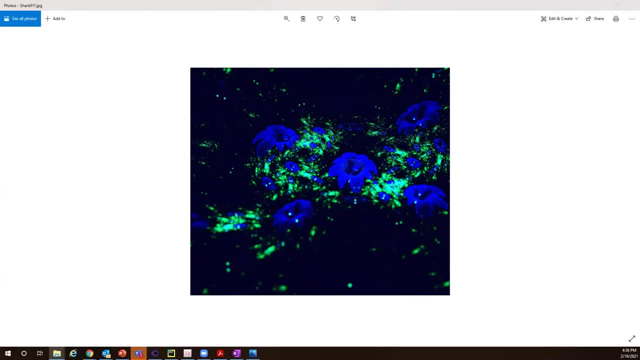 but maybe for the viewer it doesn't make so much difference. maybe the programming or the challenge is differentiating, so i don't write programs for all these. i pick and choose programs and try to play around to get what i want. yeah, and i'll also show you some flowers. that would be. 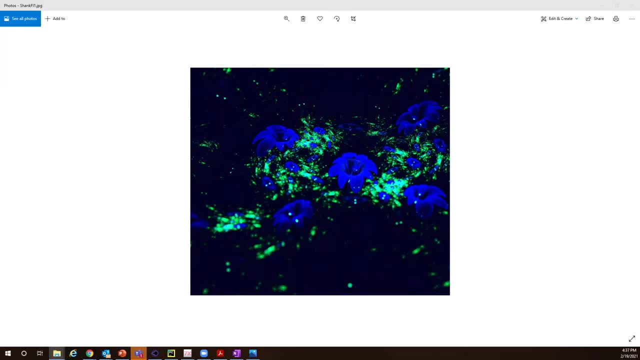 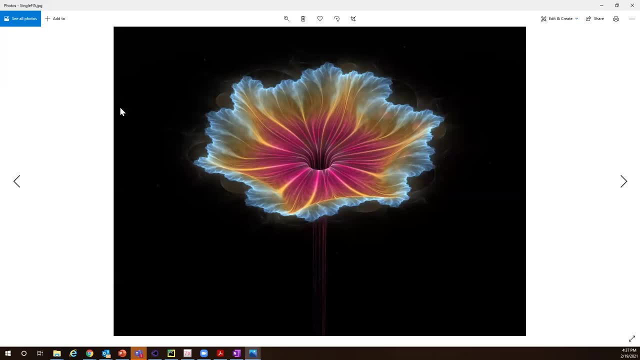 some single flowers i had created. not that one is better or another is better, but see this one, this is something which has, like, caught my fascination, like especially the edges and the glow and all that can you do and show once, like how you do, what all you select, how much time it will take to see you play around. 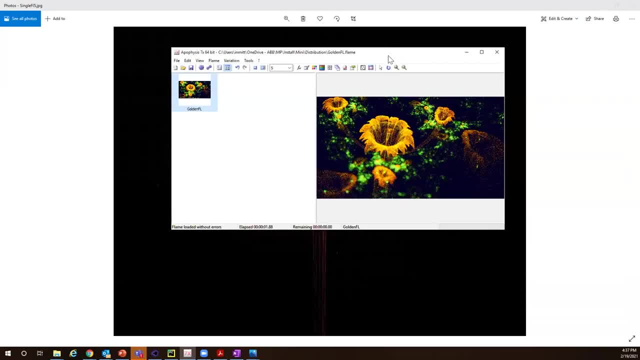 i showed this apophysis program. right, all these from apophysics, all these, whatever i showed, are created by apophysis. all the balance, and that's an important part of it. they're hidden there. it's not that the you don't get into a flower or something. 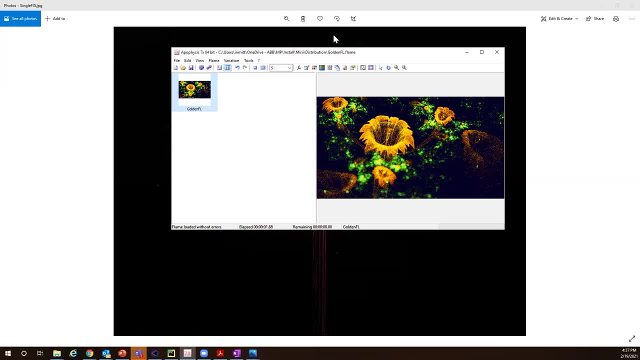 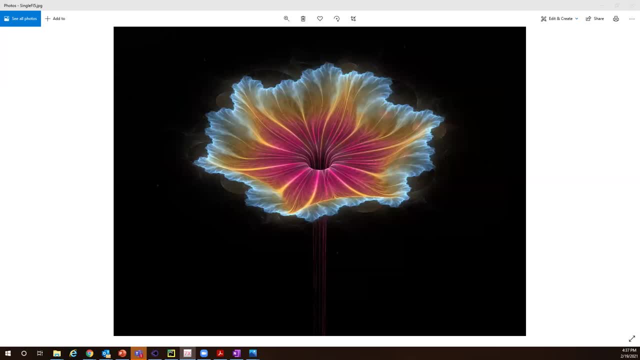 immediately: okay, there are hidden there. you may see that random. you lose your patience. it's just colors it like when you, you can lose your patience. also, she has spent around four years, i think from 2016. i've been doing this for five years. yeah, five years. 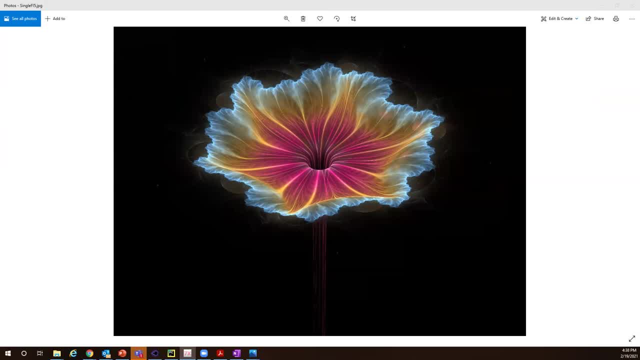 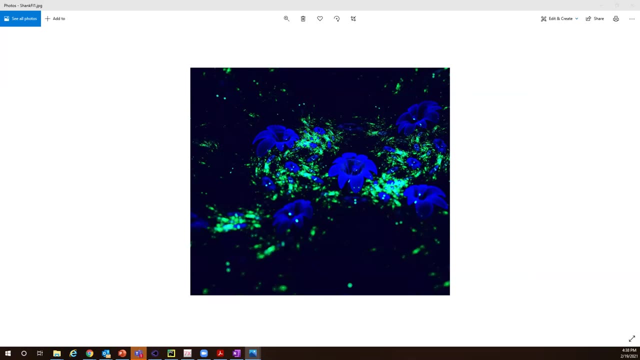 of side works sometime or the other. so these are all. whatever captures have come out of all these. yeah, i'm sure within a day we cannot do no, but you enjoy the process, yes, but not depend so much on the outcome, like when you look at i want to create some output. then only you will get frustrated, okay. 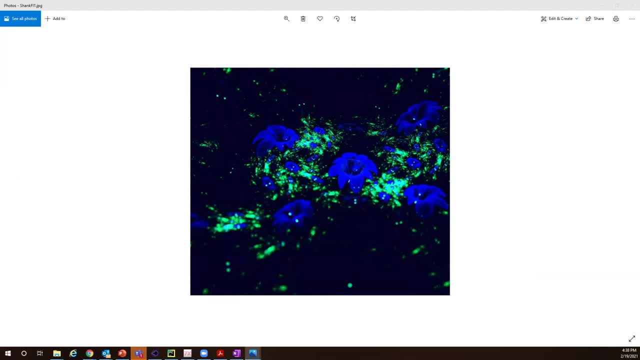 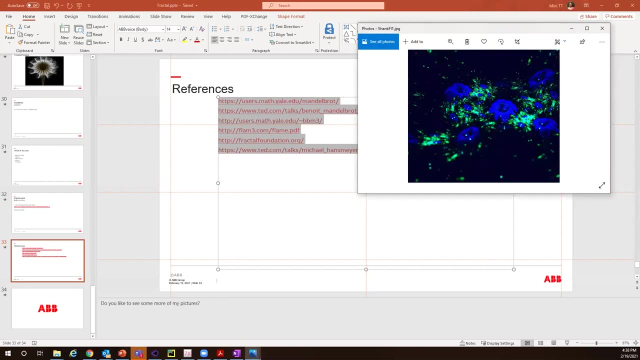 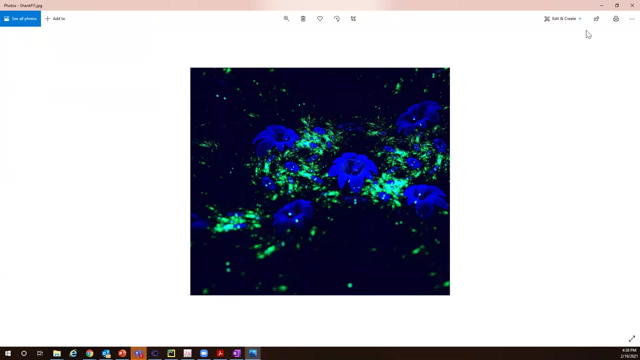 yes, yes, okay, what else? when i started to draw previous take hold, hold that blue color picture, only yes, and that one. when i started to draw, i got something like this: not on the center, one at the edges. i could see some spots alone. was it because of the picture, or it is no? no, no, i have not seen. that is what. 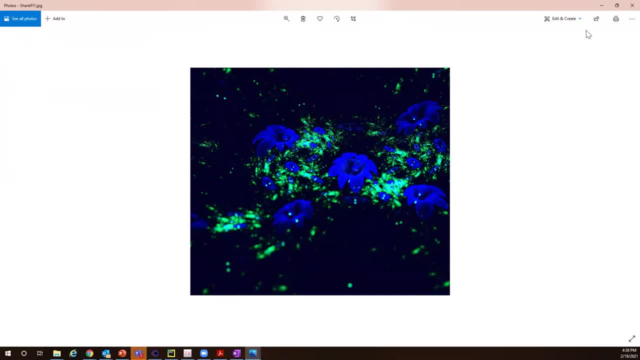 yeah, you get back to the basic. first, you put that concept into your mind. it is chaos. it's complexity theory and chaos. so your beauty is there, but then it could be there hidden somewhere. see, it's like small change. small changes can give huge change in the output. 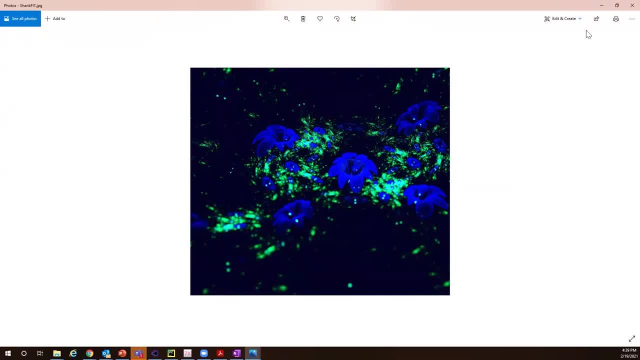 small change in input can have huge change in the output. so if you just try start from somewhere, you may not reach anywhere. okay, that also could happen. get to that concept of chaos theory deep into you. so when i see random, i didn't get anything, i have to change my constant. 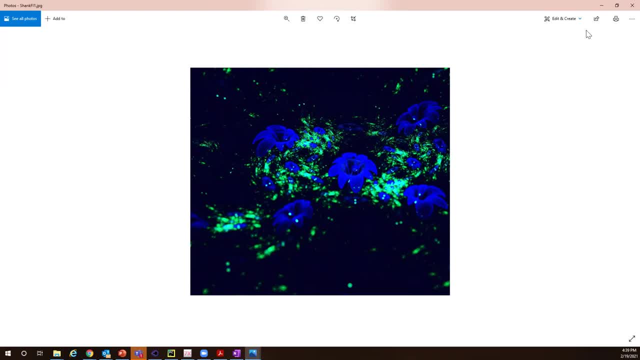 you play around with that constant, the parameters and even that location of that triangles. which program are you using, apophysis? no, i wrote my own python program. you wrote your own program. i suggest, if you like- i don't know whether that is a way everybody wants to do- like when i started. 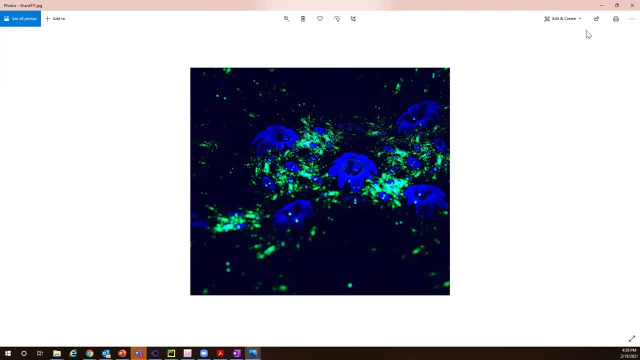 i used to write my own program, but then i only used to do simple thing like mandelbrot set, basic mandelbrot set or do that, that syringe, whiskey triangles or i only were doing a very small, simple program with my own program. but when it reached a complex one like this, i started to use 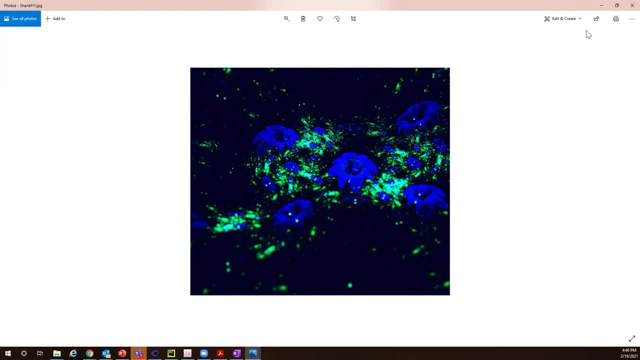 these software packages because it it can be too much overwhelming, both to focus on the program as well as on the parameter. so the the complex ones, this kind of difficult ones, i don't get into with programs of my own. in fact, these days i'm not writing programs, i think, other than trying to. 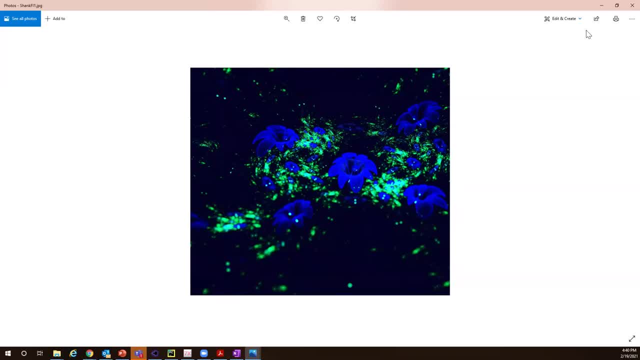 understand. when i want to understand that mandelbrot or what is the mathematics behind, then i may write some program, but to get some pictures i depend on pro these tools. yeah, but if it all depends on how much patience you have, okay, leave your contact or linkedin handle or something. 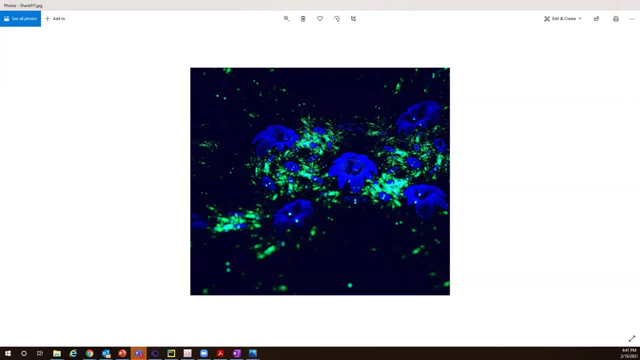 so that you can get back slides. also, you can delete any confidential information and share it. i don't know what is confidential, because these are all personal interests there may be. the only thing which i have a fear is there may be things which i would have copy pasted from somewhere from. 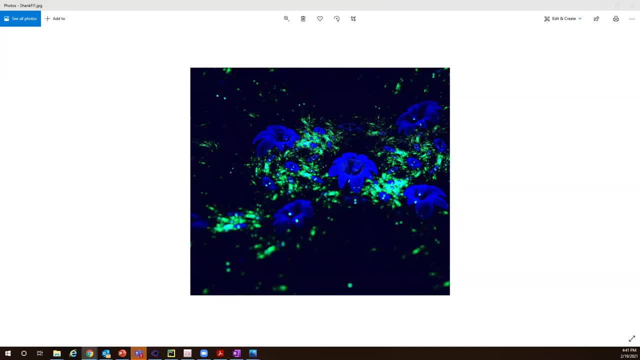 google and i would have played around. so they may have some copyright which i may not be aware of, so maybe we'll use it internally. you can share. you'll use it internally, but i can prefer it. i will give my linkedin handle. okay, so that is me. 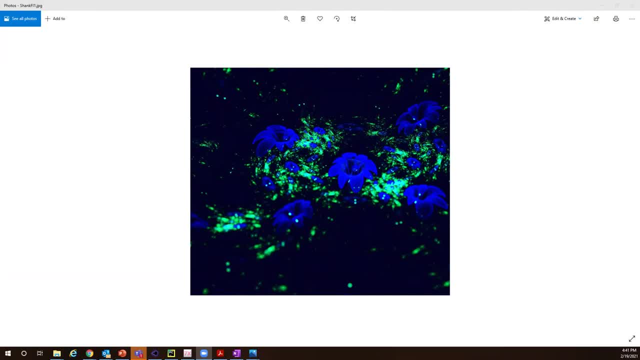 fractal group: emotions fractal group. i am not the admin of that group. okay, let me check that group. i'm not the admin. the person whom i showed that video, right, that person is the admin. i look up that group and give you thank you and i learned a lot. i am, i am into fractals last one year for hobby. i started, but 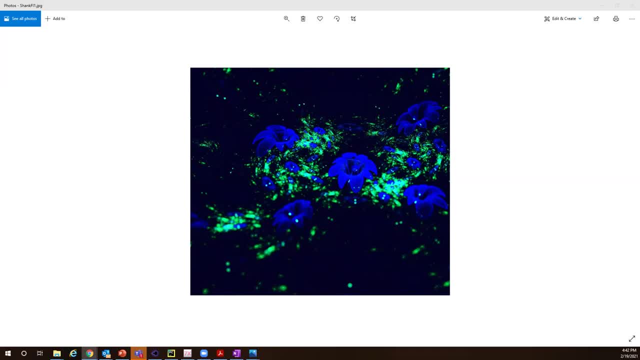 i didn't go anywhere, i just saw something. in fact, i didn't have any intention to do any of this. okay, it's not that i got. well, i started liking fractals, or then i did something. no, i didn't do at all. i had a fascination for numbers, so from number, somehow, i got into it. that's what happened.